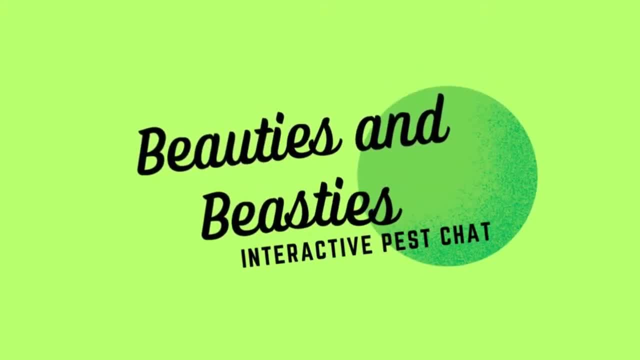 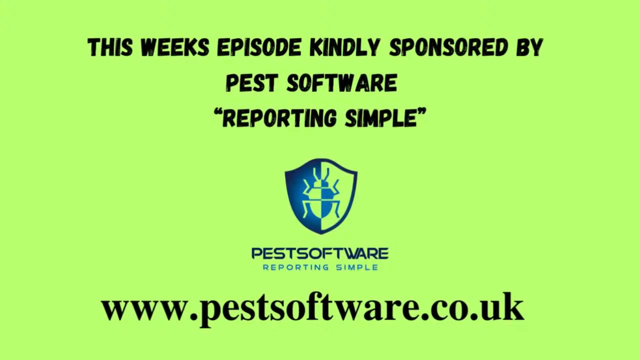 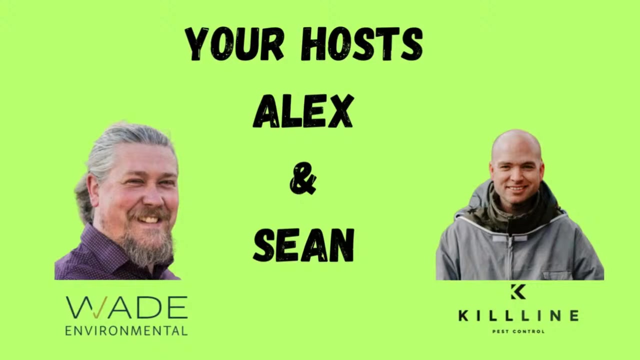 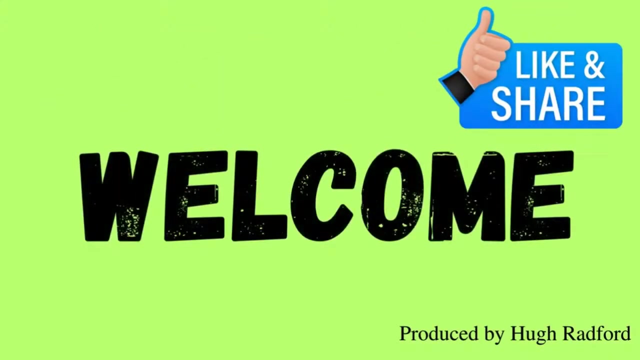 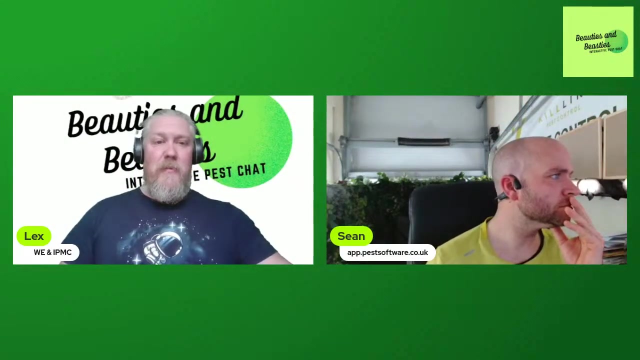 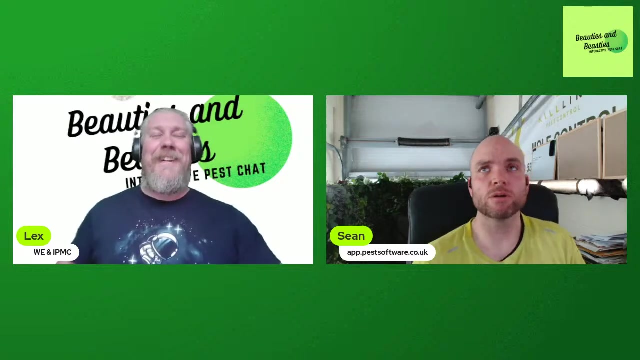 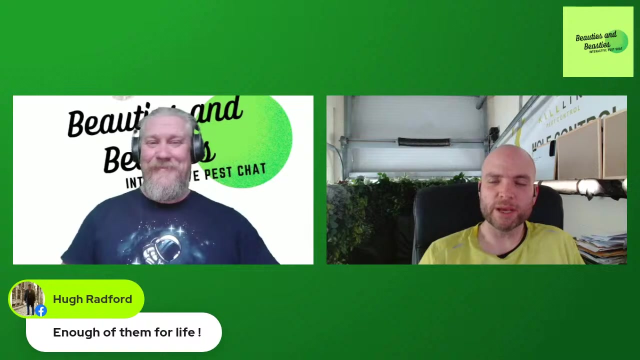 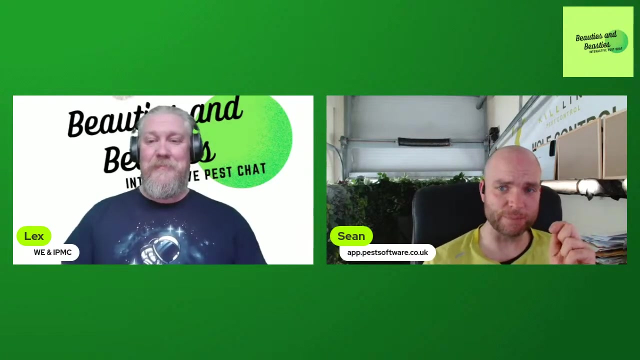 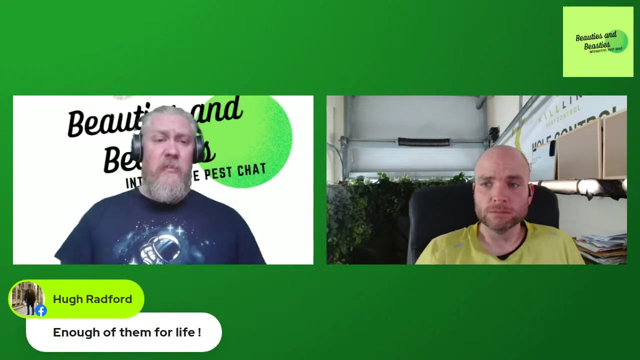 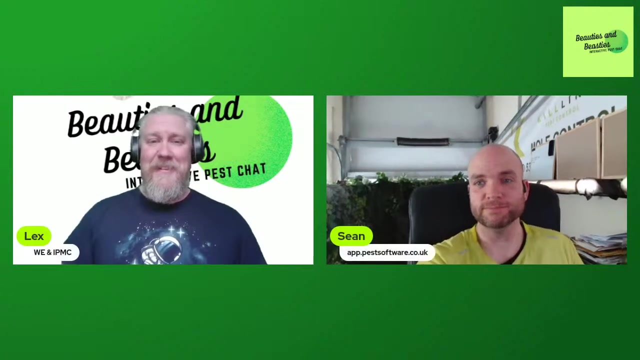 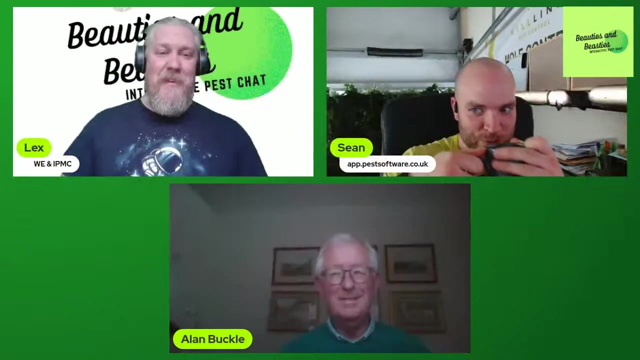 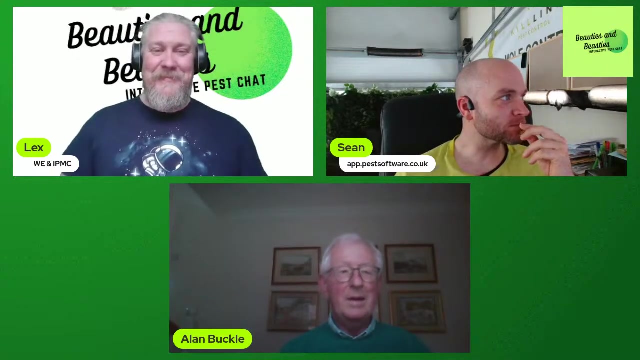 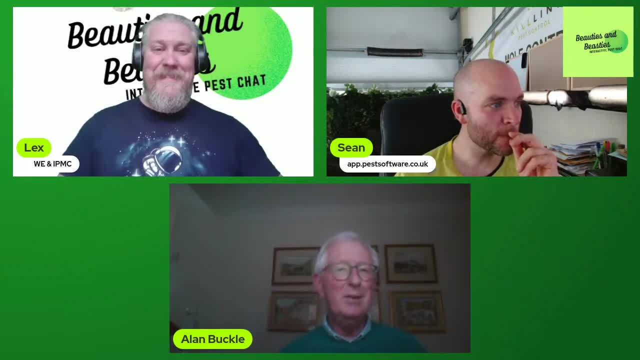 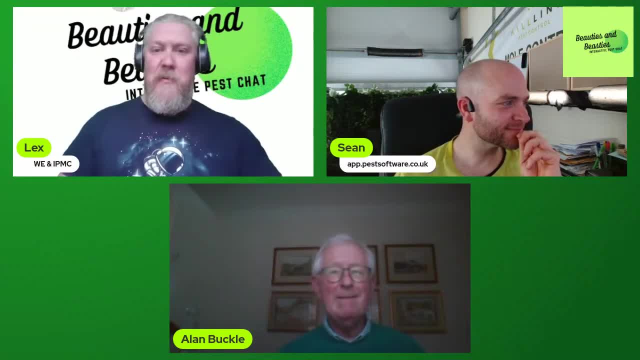 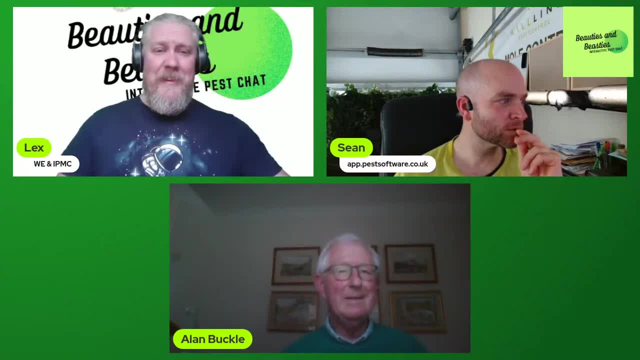 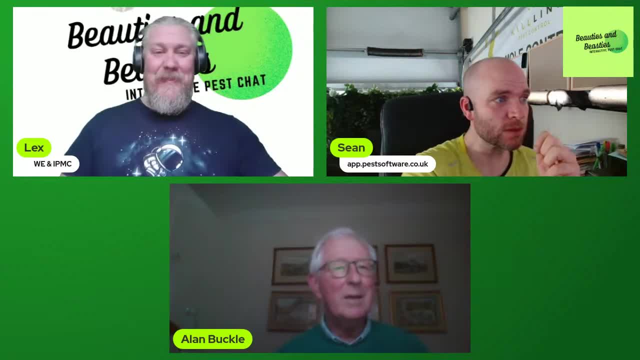 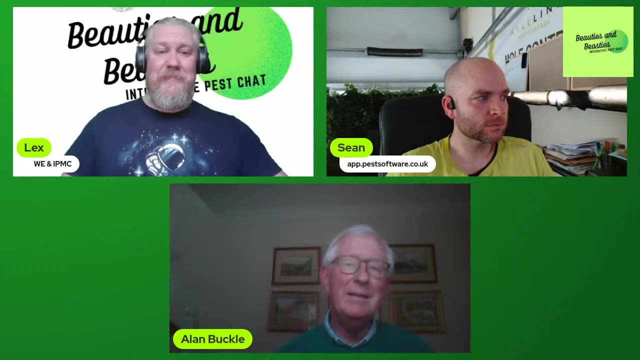 of the month. um, in a few weeks i won't be the chairman of crew anymore, and so i am. i'm walking away from that, but i have um been in the business for well for 50 years, and so i've done loads of things, but working sort of backwards. i'm probably stopping not too far away, but um, as most of you, i 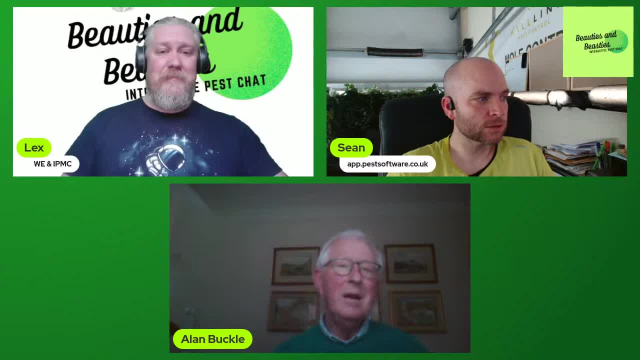 think will know, you'll know me as as chair of of crew uk and we did that, for i've been doing that for 20 years. it set up in 2003, um, and it had a very low key start and was just bobbling along for 10 years or so, really, until some things happened in the regulatory world with 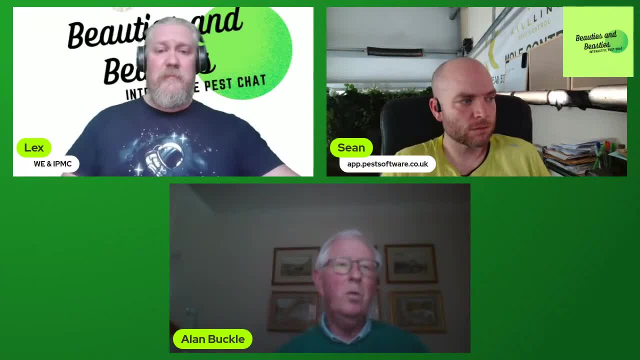 anticoagulants, um, and we it looked for a while so we were going to lose them. hse, the regulator was saying that we're not going to allow these to be used outside at all. everything was going to go indoors only. um. but the quick um bottom line is, they said, that if we set 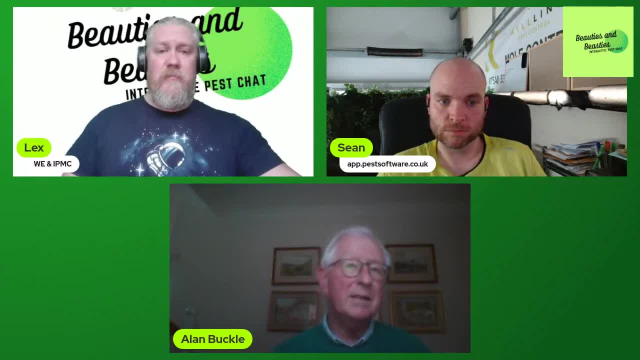 up this stewardship regime. um, they authorize these products for use outdoors, and so some of them got uses in open air and some of them got uses in and around buildings, but at least outdoors, which means that we could use them for for rat control in if effect. anything that is restricted to indoors only means you really can't use it for efficient. 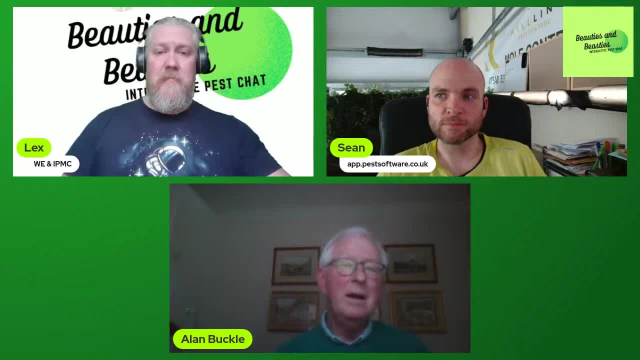 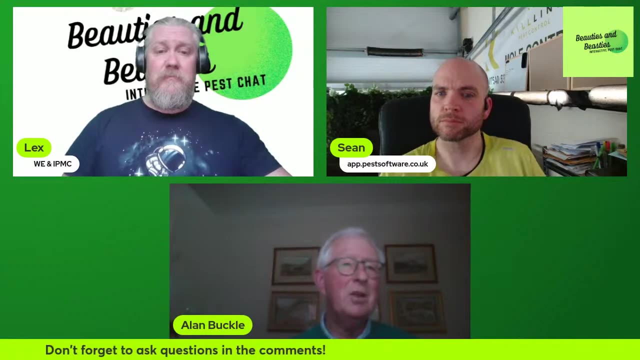 rat control. i don't think very many people can think of a? um, certainly a building on a farm- um that things can't go in and out of fairly freely. so we set up the stewardship regime and, um, that's been running for 10. uh well, it took us almost four years to actually get the show on the road. 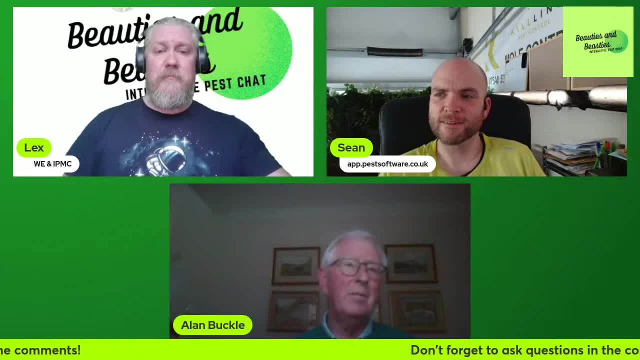 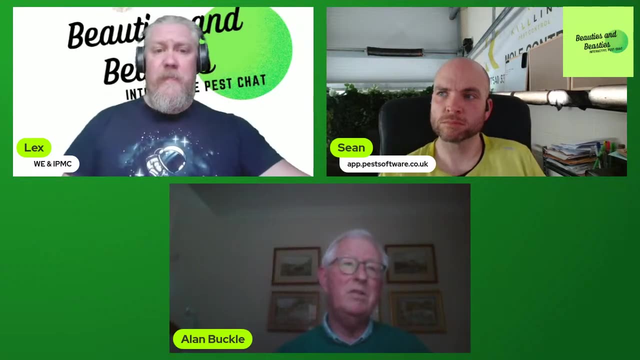 um, i think lots of people don't really realize that. um, but we started the stewardship regime in 2016, but it was a huge amount of work to put the whole show together. um, and that that that took a while. so, yeah, that's how most of you know me. before that i i worked in industry and i 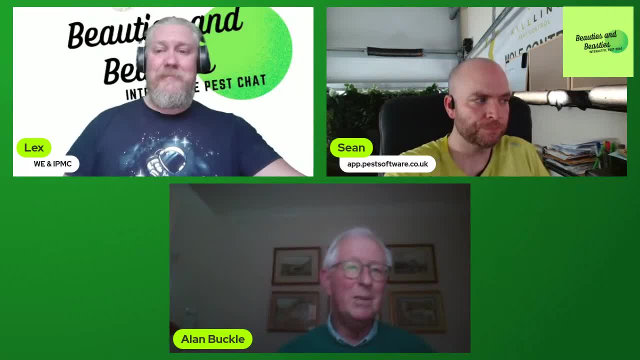 was always on the technical side, so i i didn't- i didn't- flog anything to anybody. um, i was always a research and development manager and i worked in genta, uh, based in basel um, and in those days i was doing much more to do with things like that, and i was doing much more to do with things like that. 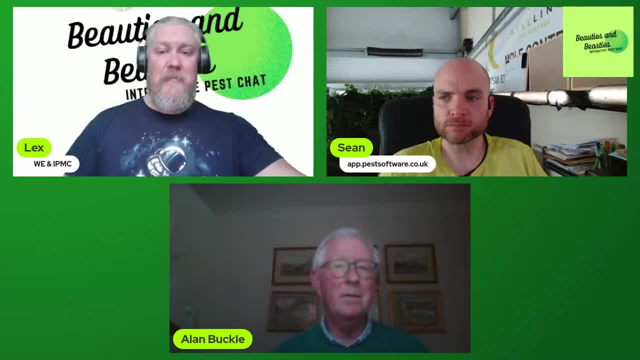 insects, in fact, for for quite a long part of my career um i was working on insect control, because markets for insect insect based um solutions are much bigger than rat ones, and so loads and loads of my work was to do with um malaria control with cockroaches um termites. 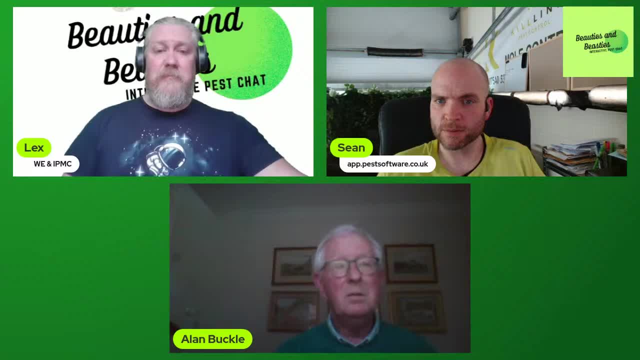 even, and we did lots of termite projects too. so, um, that was in gender, and before that, um, it was something called zeneca. we're now really going back in trade history- um well, actually wasn't it. and then it was zenica and then it was. well, it spent a while as astrazeneca. um, 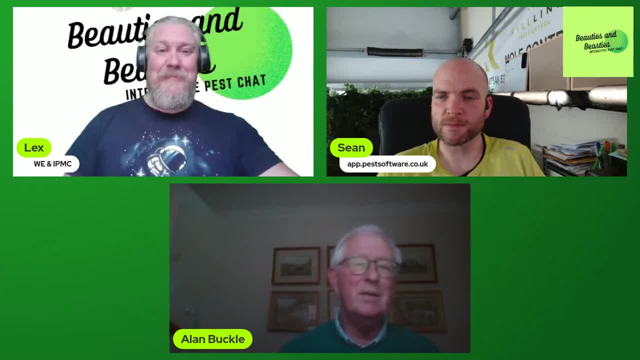 they. they then kicked us out of astrazeneca because we were the dirty part of the- they were the fouty- so they got shot at us. um, and so we zenica. um, i was a government researcher for quite some time and and did loads and loads of the early work to develop, um, all of these. 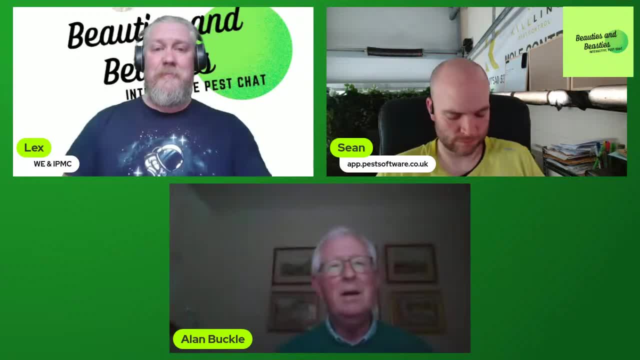 anticoagulants. so there was a guy up in probably the middle of a highway in witness inventing rhodiophicum and diphenicum and flocumafen in his lab and he was giving me little files of white powder and i was putting them on farms um in wales and hampshire to see. 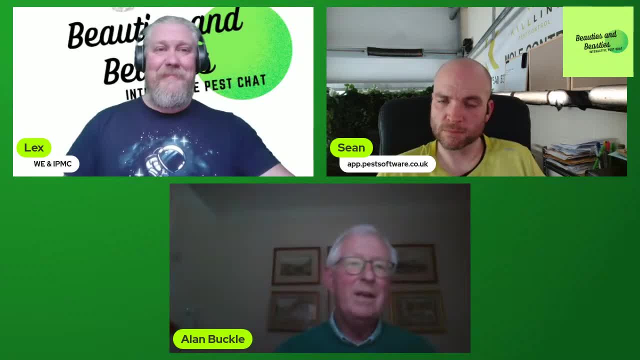 if they, if they work. that that was sort of back in the in the 80s. so that that's how far back i go, and i think that's probably enough of the history. well, i mean, that's that's. that's a fair way back, and i'm right in understanding that. you know, some of those little vials that we're using were 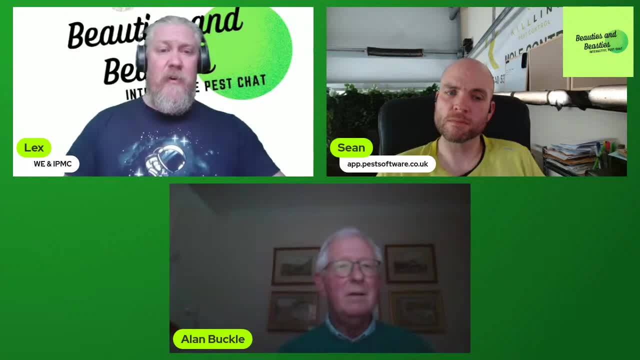 things like rhodiophicum, weren't they there? there you were involved with the testing of things like rhodiophicum and products that we use to this very day. well, yes, the the very early field trials um were on some of those products. i i came in a little. bit late. i was out in malaysia for four years while um rhodiophicum was was coming along. i was testing it in rice fields, um, but um i i came back from malaysia and it was then that flocumafen came along, and so i did all of the um development field trials: on, on on flocumafen, um, and then 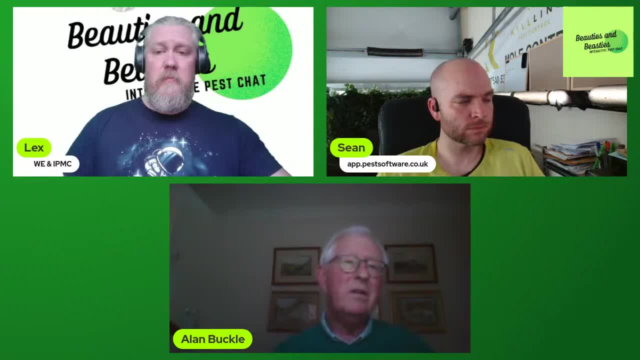 after that i got sort of headhunted out of um the minister of agriculture and went into what was then ici. so, um, i i joined, i joined ic i plant protection division um, and i've just been involved with with rodenticide ever since we we did the very 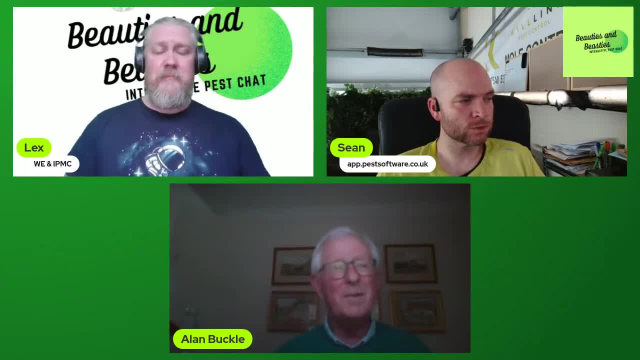 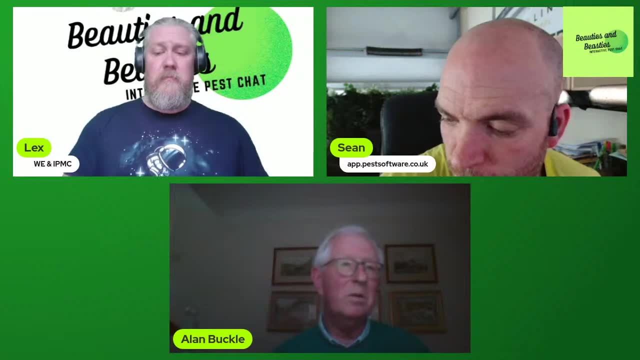 early work to develop the very earliest and first wax blocks. um we, up until we got started, most of the baits were whole grain baits or cut grains, and so we we developed pellets as well. um and then we had to develop um pulse baiting, and so quite a lot of the work that i did was to start. 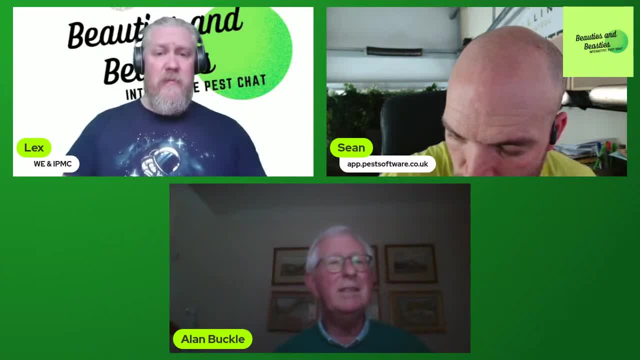 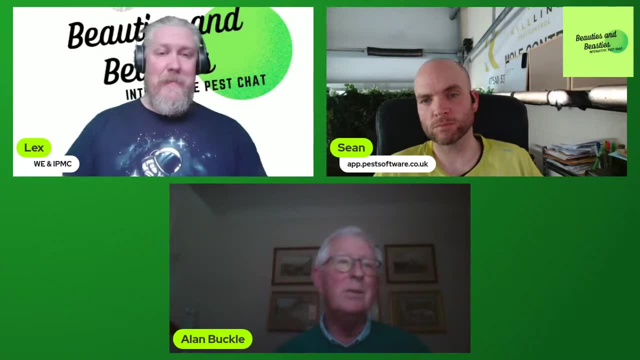 the ball rolling with post, with pulse baiting to try to stop rats eating as much brodyphicum as they wanted to do and would kill them the time's over. so we had to find a way to stop that, and that was what pulse baiting was about. was uh, a project that you did with um, me and and duboc was. 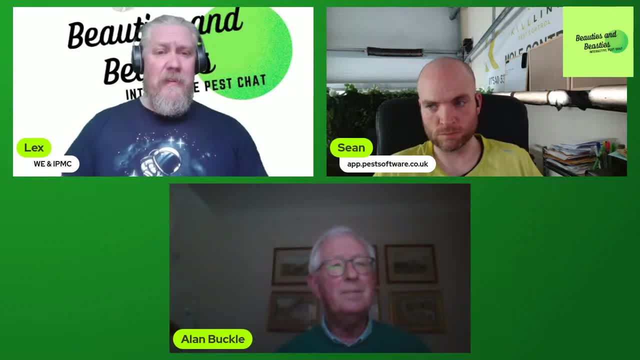 it. um, who? who helped you with that? well, yes, adrian agent. um, he, he, his, his and my past were quite well entwined, because he did my job at the ministry and just out. twice i stepped into his job in the ministry and then he, he came and pulled me out of the minister agriculture and dropped me into icr. 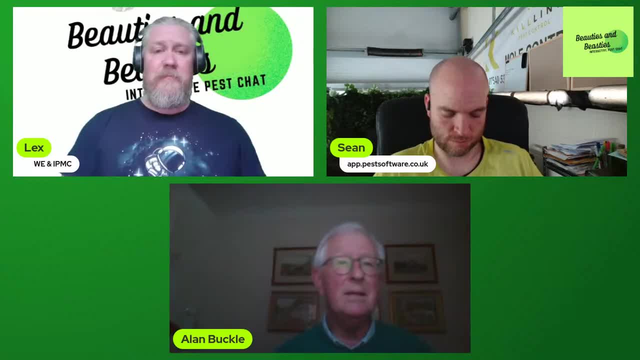 underneath him. so that that was, that was what what happened there. but we we did lots of the early work on on bitrex as well. someone came along, a guy um called called harry payne, um he had this bittering agent and he thought it would um. 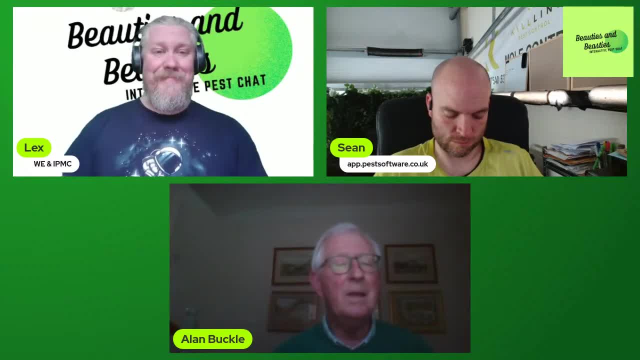 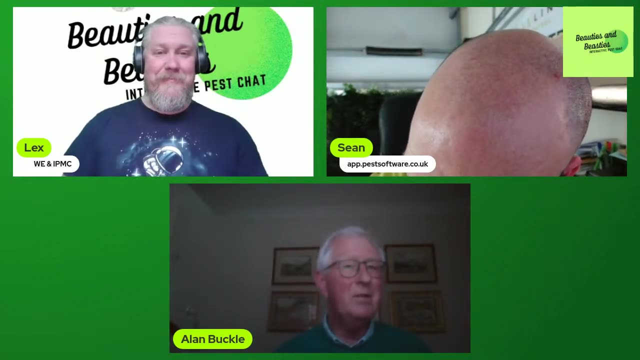 be an idea to put it in rat bait, because he didn't think rats could- um, could, could- taste it, because he'd been doing some sort of toxicology work on it. and he knocked on our door and said this might be a human-tasted terror. and so we did all of the early lab work and field work. 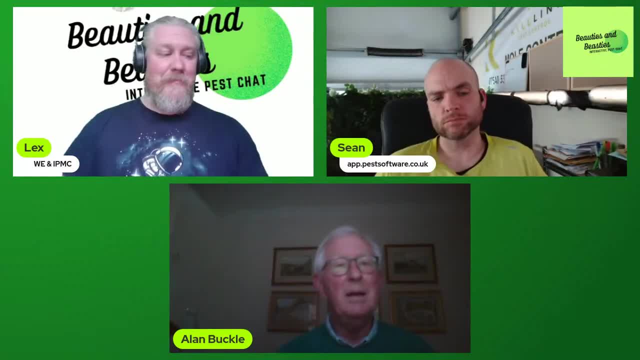 to get bitrex into the very first um rat baits and since, since then, that's gone global as well. so pretty much all the. what are your thoughts? yeah, so what are your thoughts on bitrex? because i'm reading more and more studies coming out. these: 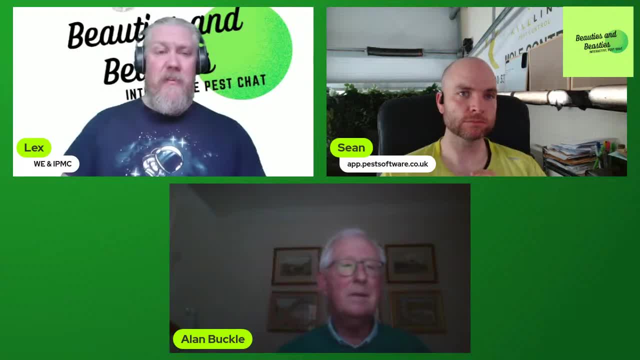 days saying that, uh, what once was um undetectable by rats and mice. um, we've, over the last 40 years or so, been selecting for mice that can now um taste bitrex, and some of the control failures we see maybe as a result of um. you know this, you know a genetic um trait: to be able to suddenly taste it. 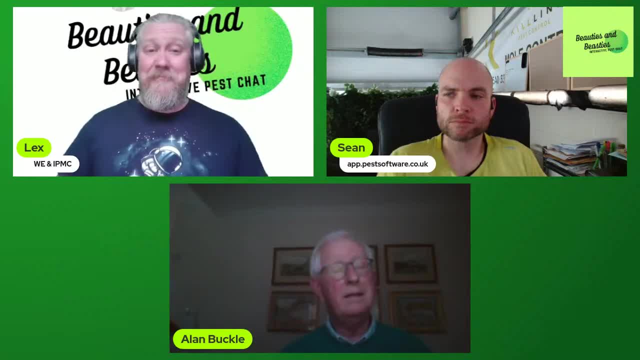 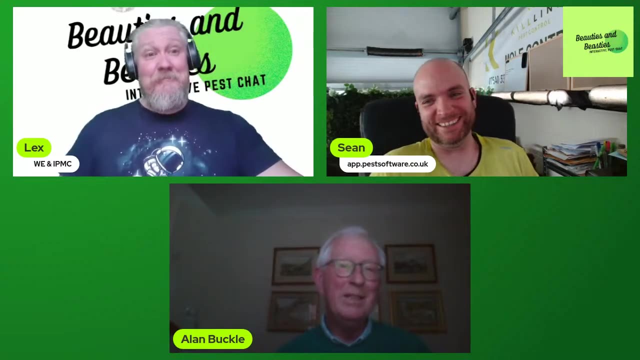 um, and i think it's interesting, i, i, i don't. i don't think that's surprising at all. i mean, if, if you can think of selection pressure that is stronger than you eat this, you're dead. you don't eat this, you survive- that's a fairly extreme selection pressure. so, um, yeah, that that that's i'm. 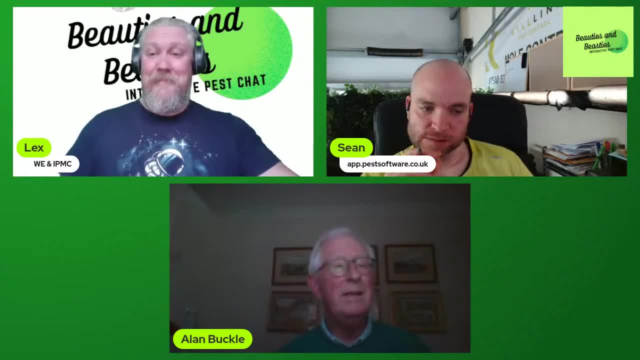 surprised. it's in fact that long. i mean we, we did all the lab trials um, first of all with um lab rats and mice albinos, and the session was that their sensory perceptions were much less acute than the wild rats were, and so we we had to go and do lots. 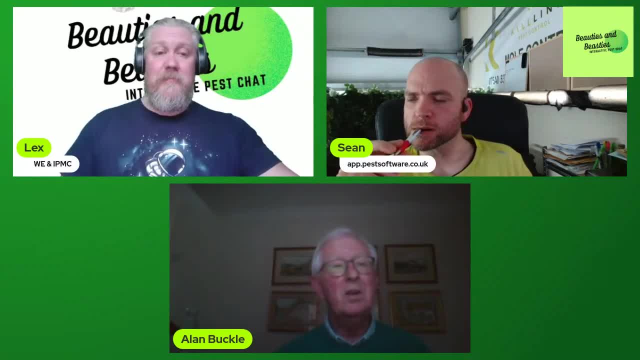 of wild rat tests, both in the lab and in the field, to try to persuade ourselves. because when we tasted this stuff it was absolutely mind-blowingly terrible and we, we, well, i couldn't understand why a rat couldn't taste it. but, um, there is some physiology, um explanation for that, um, but 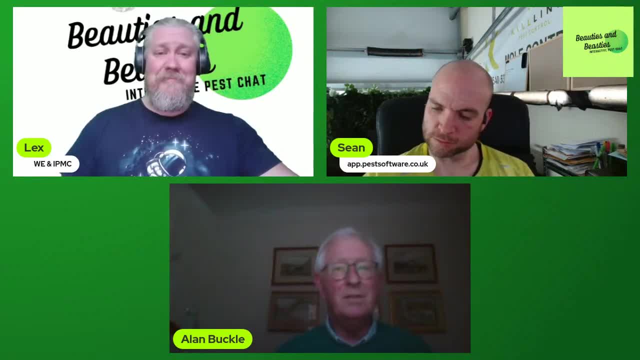 um, yeah well, we did the test. it worked fine, but after 40 years, um, anything could be happening. answer, well, i mean, i, i could know, you know me, i could, i could nerd out horribly. but we're starting to get some questions through and actually there's a really good one just popped up and i saw sean's uh ears prick up at this. so sean, 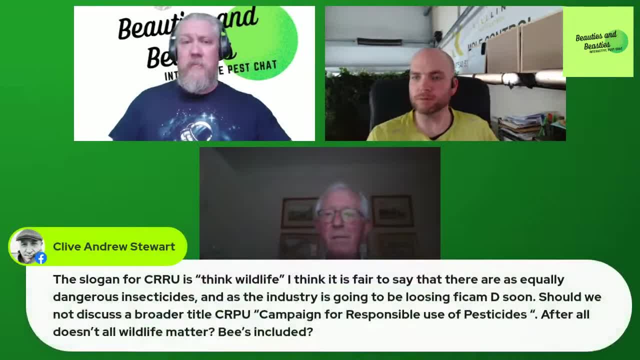 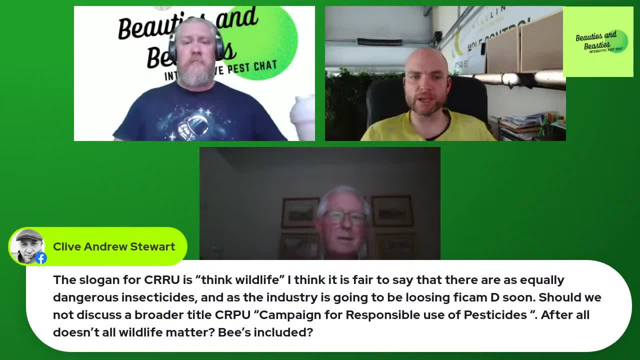 do you want to? do you want to just uh clive's? um, there we go. yeah, the slogan for crew is, i think, wildlife. i think it's fair to say that there are equally dangerous insecticides. loss of fat and piperinol at the minute, isn't it? and as an industry is going to be losing fire. 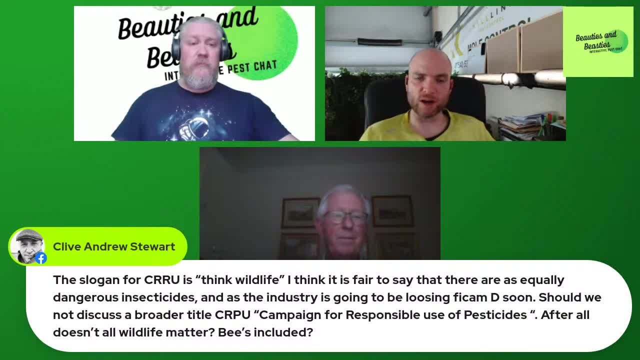 camp day soon. should we not discuss a broader title: crpu, the campaign for responsible use of pesticides? after all, doesn't all wildlife matter, bees included? talk about bees. anyone mentions the other thing, you get sacked. you don't know what we're talking about, alan, if anyone mentions 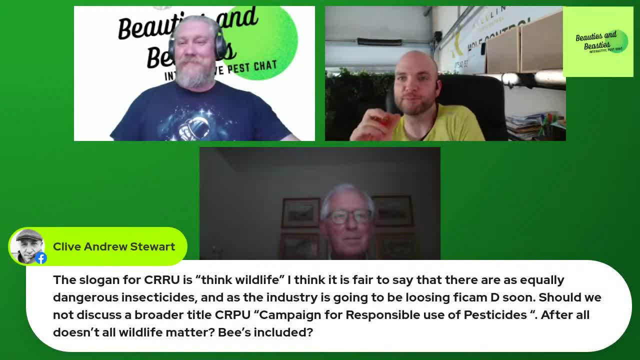 anything to do with what spoke for the last four weeks. you get sacked, thrown off. but yeah, um, well, that i mean thank, thank heavens. i'm leaving at the end of the month because that that new, new um campaign that you're just starting there is is quite, is quite a big one. it's a very 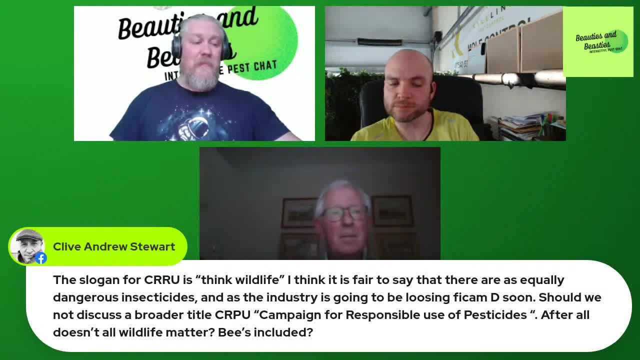 serious point and i'm not making light of it at all. um some time ago, um once, crew not going with stewardship, it started to sound like a good idea. um it really um. i don't want to go too much into the politics of it, but it it satisfied um the regulators, um, for quite a long. 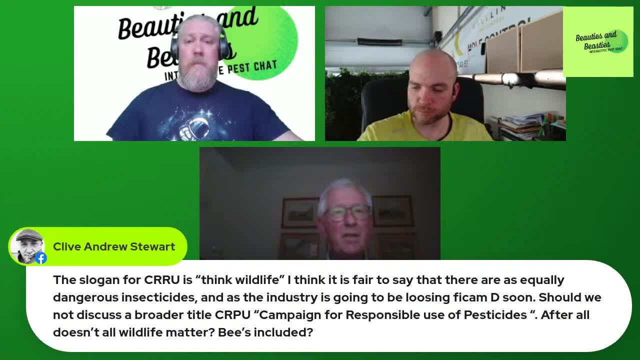 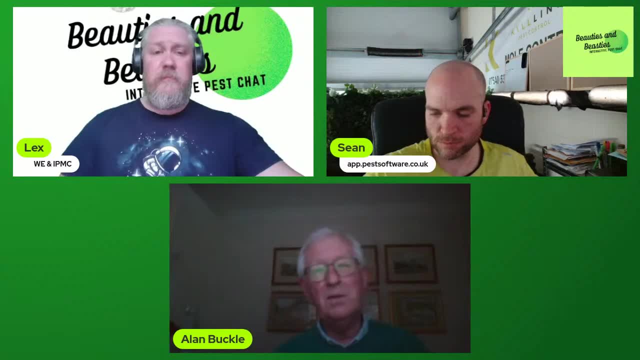 time that, um, we were doing something about these highly toxic, highly persistent chemicals that are the anticoagulants. um, i'm sure most of you know that, that they're actually, they're all um candidates for substitution and that that's a polite regulatory term. some, the candidate for substitution. 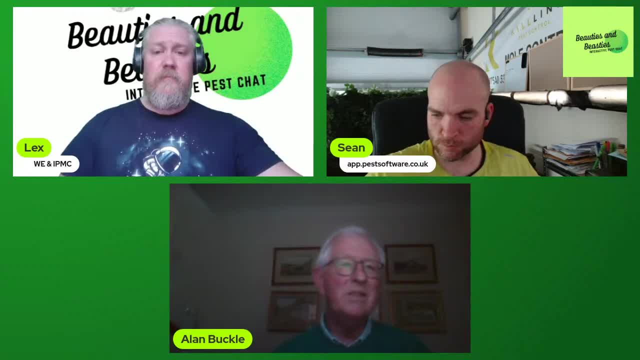 which actually means we just want to get rid of them as fast as we can, and they, they, none of them should should be on the market um, but we, we managed to placate and and sort of keep the lid on the whole thing and allow rodenticides to be used um and to and and to carry on from for for many years, and those 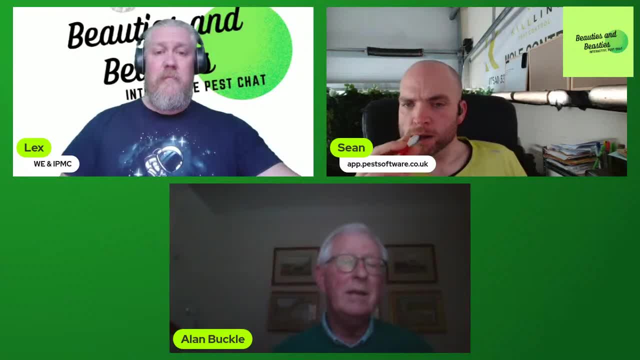 that were dealing with this exercise said: yeah, well, that does sound like a good idea. if, if you can do it, um, why can't we? and for some time there was talk about a similar insecticide group, um, i i don't know what they would have called it, um, but that didn't come. 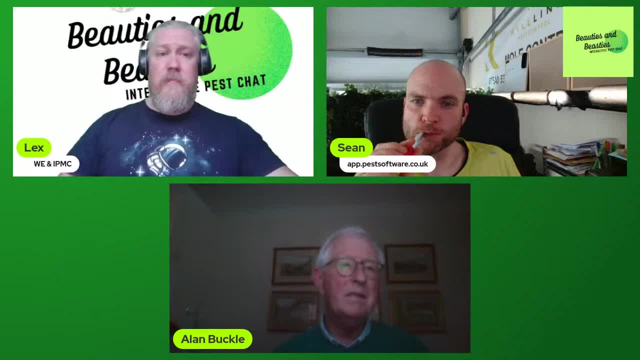 to anything. it was certainly there. there were. there was talk in bpca um that they they wanted to try to pull together um a group to defend insecticides in the same, in the same way. um, and certainly i couldn't agree more about all wildlife matters. it's not, it's not just the ones. 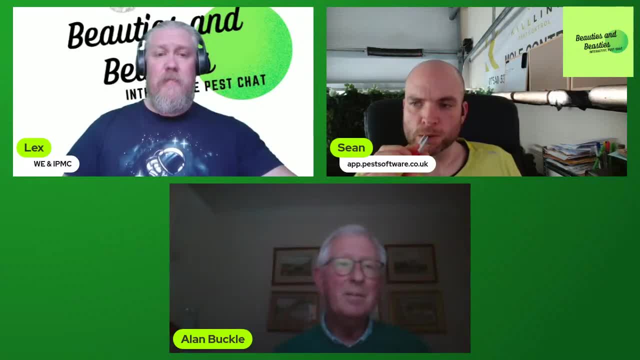 that are affected by, uh, rodenticides. but, um, we we've we've bitten off a huge chunk with crew and we really haven't haven't digested it at all, and so, um, i i wouldn't want to be taking on um a load of other work. i'll stop. i'll stop talking. 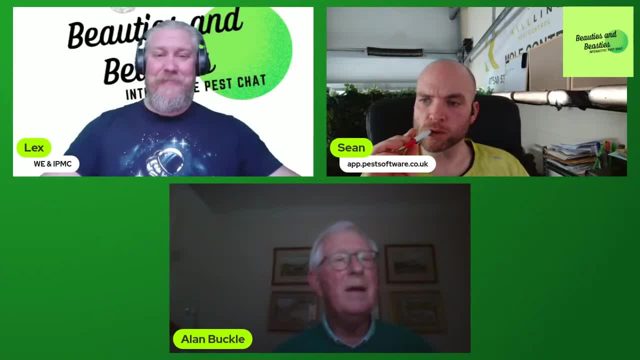 about this one now. but, um, almost all of the companies that sell these products- and you mentioned um, fi cam, um, they all have their own stewardship programs. um, the crew program in the uk is only a one-off um, and so, um, i think that's a good point, um, because, um, all of the rodenticide manufacturers 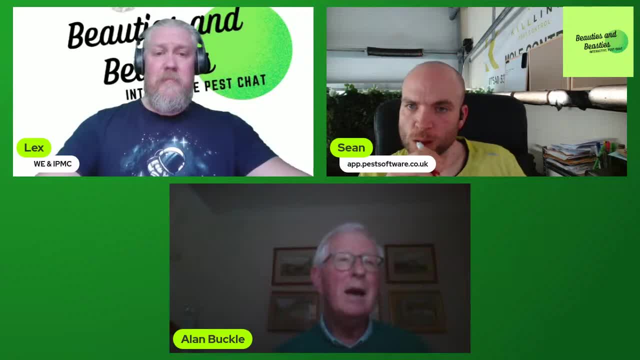 all thought they were under exactly the same pressure and all got into a room and said we need to do something about it. let's start crew. um, but um, more behind the scenes perhaps. um, you will find that almost all of the big companies, particularly the envus, stroke bayer, bsf. 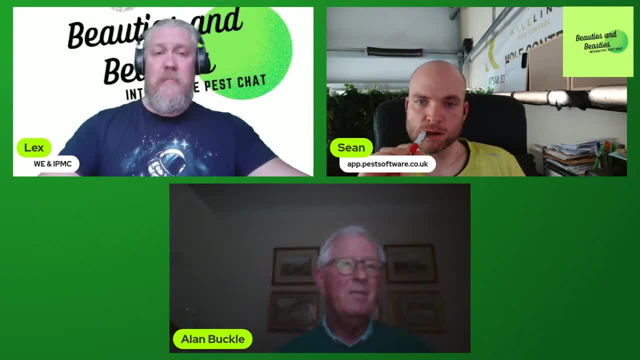 syngentas, all of those multinationals have whole bunches of people doing stewardship and trying to do something about it. i think it's um, uh, i think that's a really good point. um, i think it's a really good point and i think that's a really real um, very good point um to uh to hear from them as to 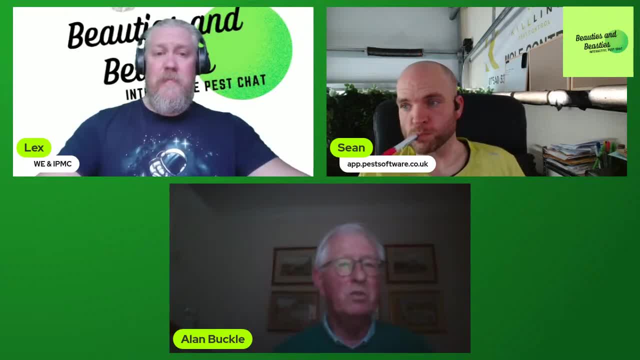 how they're doing with the work that they're doing with this and um. so i i think i think, as i mentioned uh at the time i hurt, when i was um trying to get around with this- we would have had, uh, some kind of um um problems with um um. then i think we had, i will say a few of the things that 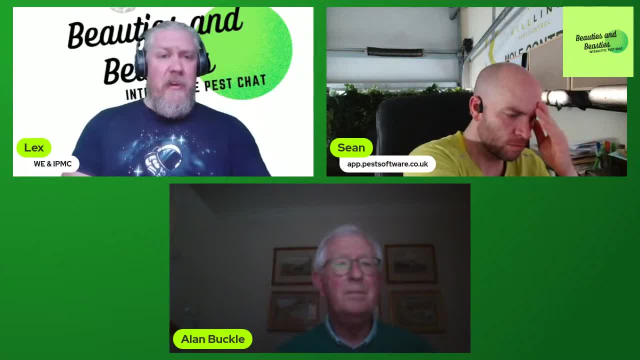 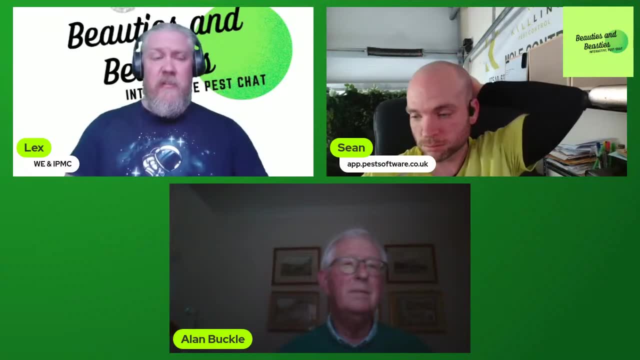 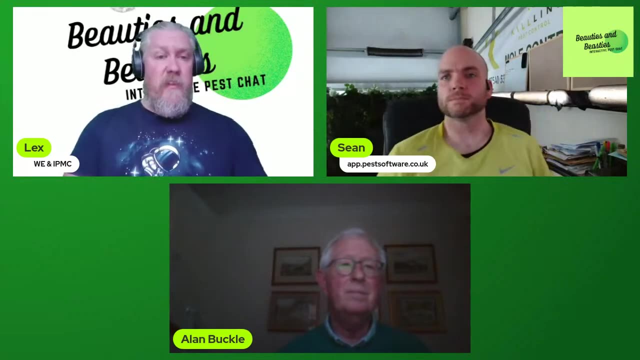 can understand this very well. um, the 25 parts per million and reprotoxic um saga was an interesting one because when, when industry spoke to uh the regulators and that was discussed, it was the, the body of science that the regulators had behind them- said that anything, uh, there's this. 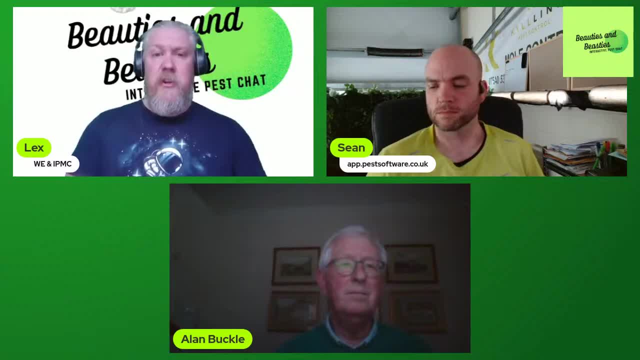 thing called fetal warfarin syndrome, and anything that is based on the molecule warfarin has the capacity to cause damage to the unborn child, and they then came up with this caveat that anything above 30 parts per million is going to be, uh, potentially reprotoxic. however, when, when we 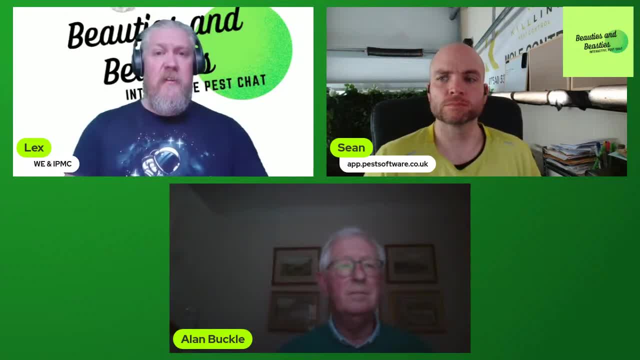 challenged them and said: okay, so if we don't, what happens? instead of eating a single 50 ppm block, someone eats 225 ppm blocks. everyone shrugged um and and so it's. it's interesting to see that, you know, there is there's good science and there's bad science, and it can sometimes be. 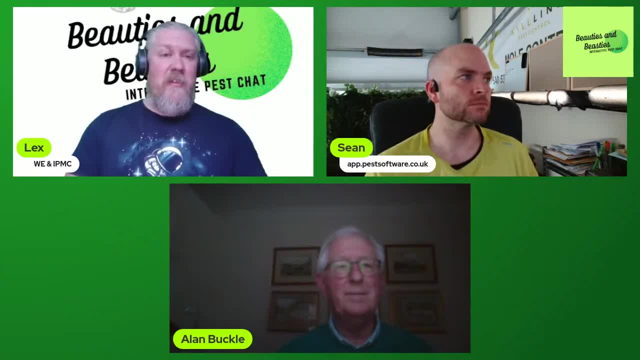 um, you know, it can lead to these fairly interesting complications throughout our industry, which is quite novel. so there we go. i, i was, i was chairman, i was chairman of another industry group. um, there's this group called sephic, um, based in brussels, and they are um a group. it's a bit like: 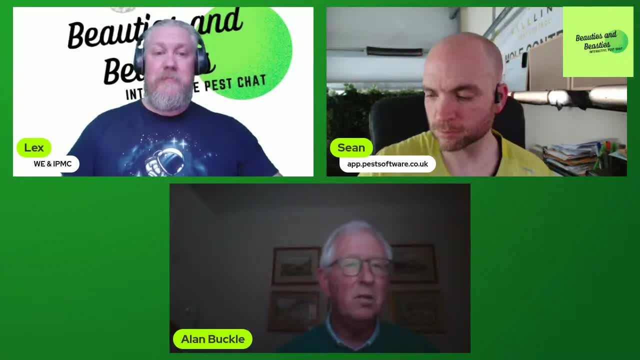 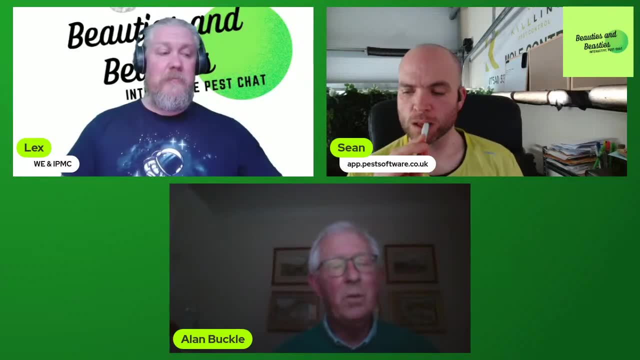 crew and and all of the manufacturers of all of the biocides sit, sit in a room at at sephic. um, we, we, we. we had a rodenticide team and we fought that reprotoxin issue for 10 years and we actually managed to keep them at bay for for 10. 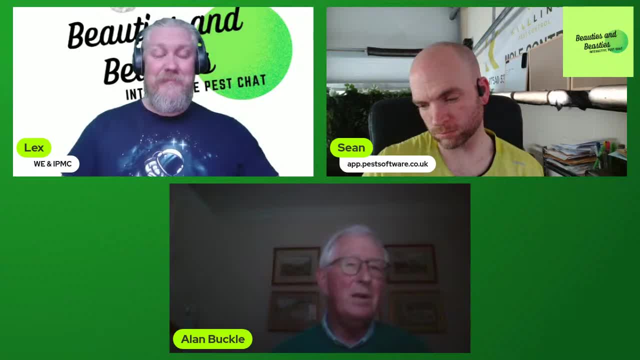 whole years, but eventually they managed to find a way to sink us um and they they used, i would say, questionable means, but they were determined to get these substances labeled reprotoxins and, although we delayed it for 10 years by a number of different things that we did, 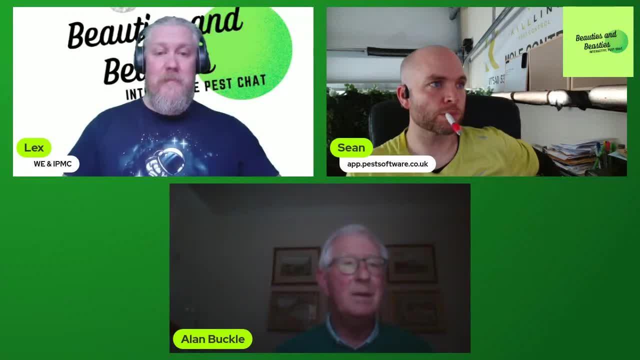 um they, they got through in the end just goes to show you that a lot of these um things that people you know, these changes that uh, we see happen and um, the pest control industry, the, the all of the guys listening to this today- think happen overnight and on a dime some of them have. 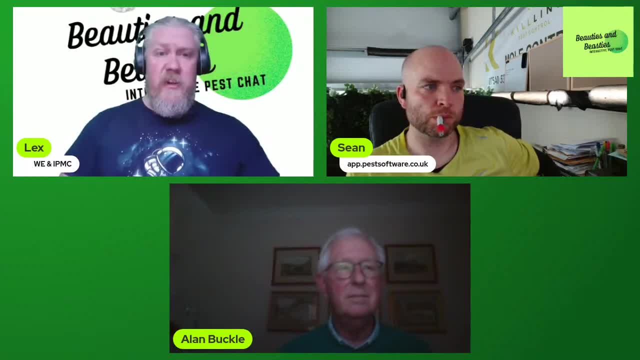 been actually in the mills and in the works for um, you know, 10, 10 years, 10 years plus. i mean sorry i didn't, i didn't mean to to interrupt, but but you know the, the industry stewardship is fighting these things for all it's worth. all the time below the surface, um, but um, obviously the uh. 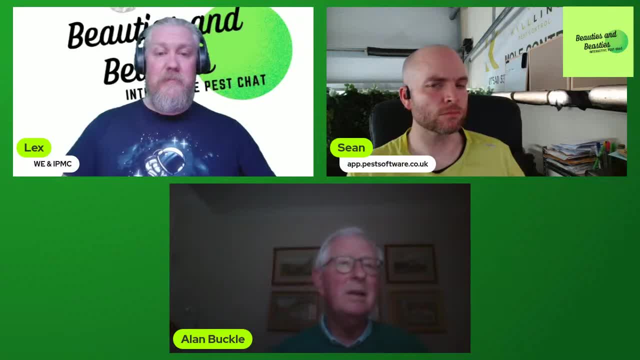 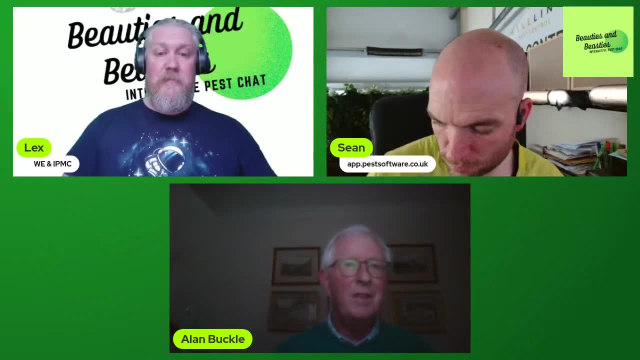 the regulators hold a lot of very strong cards, um, and they've got time in their hands and they can wait, and they just wait and wait and they find different ways to um, to go at things until eventually they, they, they win the game and that's that's. that's certainly what's what's been happening. well, i mean, hugh radford makes an. 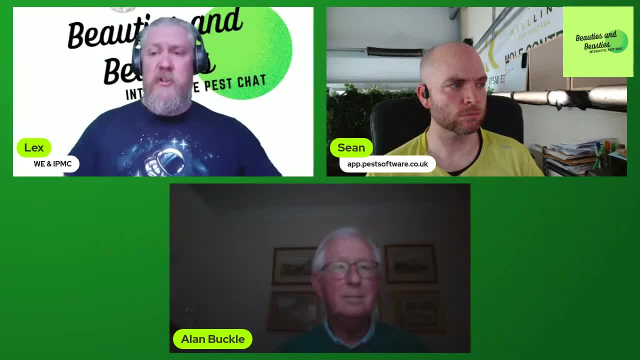 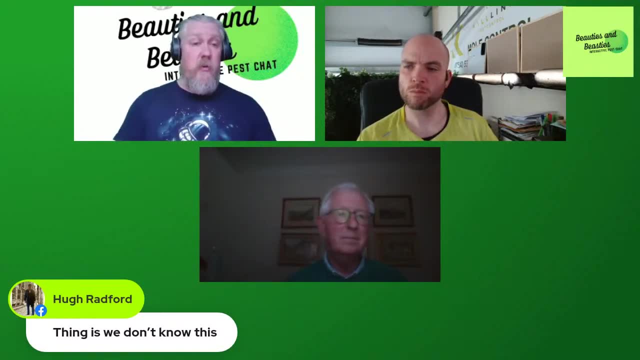 interesting point, which is- and this is, and i have voiced this before- which is um, a lot of people on the ground, a lot of the people using these products- you know, the vast majority of the industry- who are not the manufacturers and distributors and developers of these products. 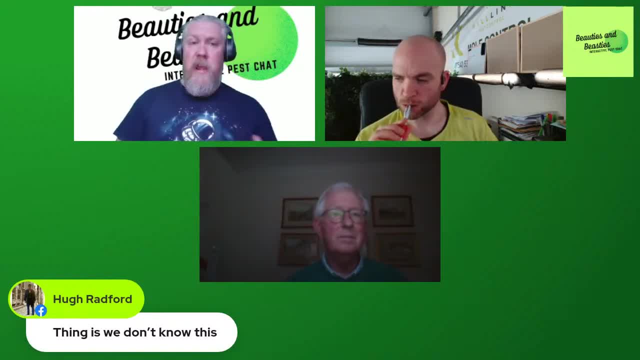 they have no idea what's going on behind the scenes. there's probably a lot more empathy and a lot more support for, you know, crew, sephic and a lot of these um, stewardship models, um, but people don't know. and i have to say- and i'll stick my neck out on the block here, crew has. 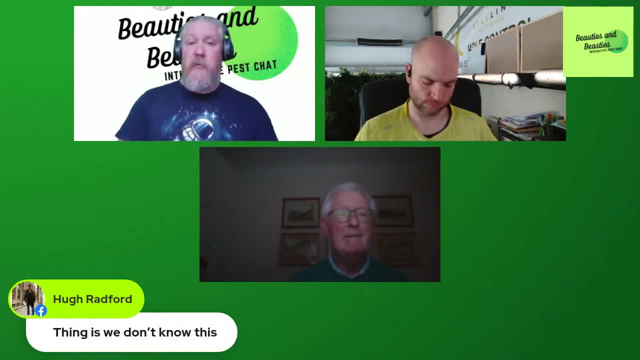 not been great at disseminating information out and back down to the public at least. um, a lot of pest controllers feel that, uh- and i don't think i'm wrong in saying that- i think we'll probably get a couple of comments there, hopefully agreeing with me, um, and a lot of them feel as though there's 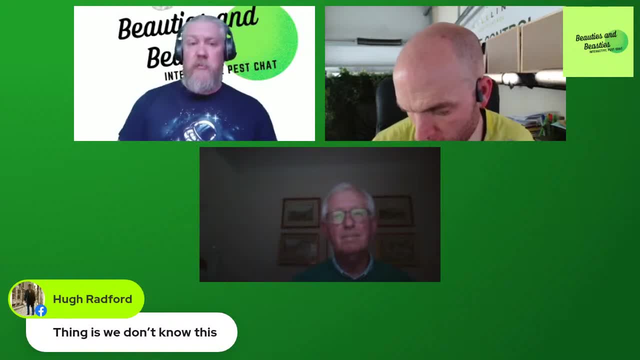 no communication. um, which is unfortunate because of all of the things that you guys have been doing- the scenes. there's obviously things going on, but that's that's how it is. well, alex, i i'd like to question that. some, some, somewhat, they are there. there is a process that 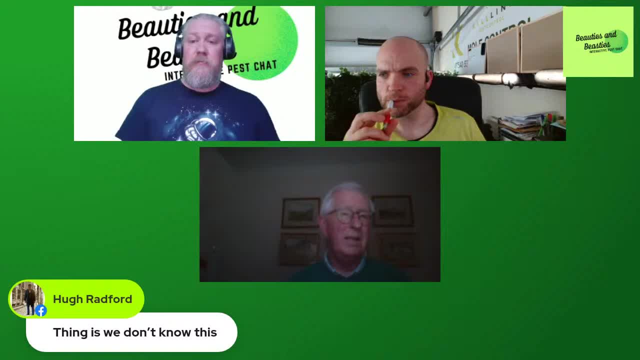 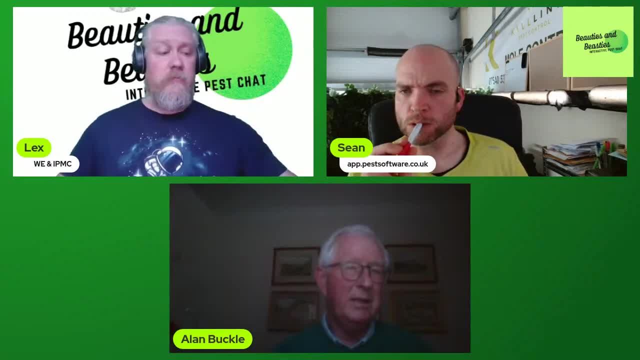 and he and i um write these press releases, um, and then they go out to almost everyone that we can get. who would receive one of these press releases? and what then happens? almost always they're all picked up by the main pest control magazines. so professional pest control, pest control news, um. 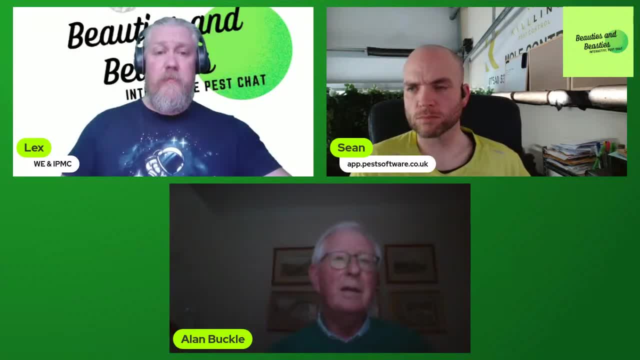 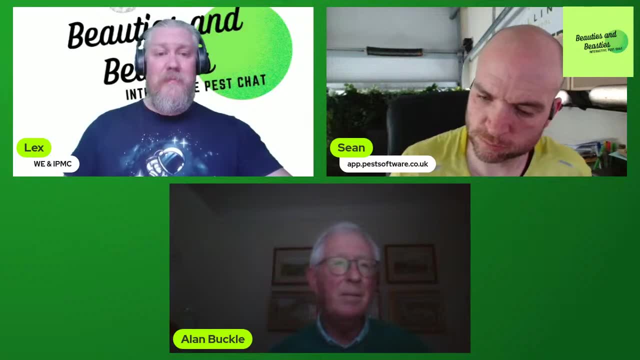 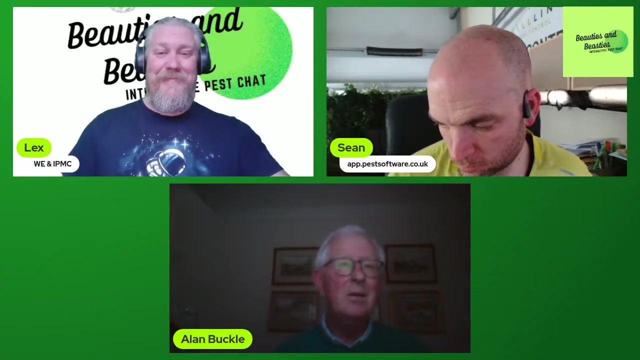 that there are four and i- they're not all all coming to mind, but almost everything that that we write um when i pick up um pest control news or people, or ppc or or pest or today's technician, those are the other ones, those four, um i i'm in almost every one, almost every week or every time they come out so and i get them all and 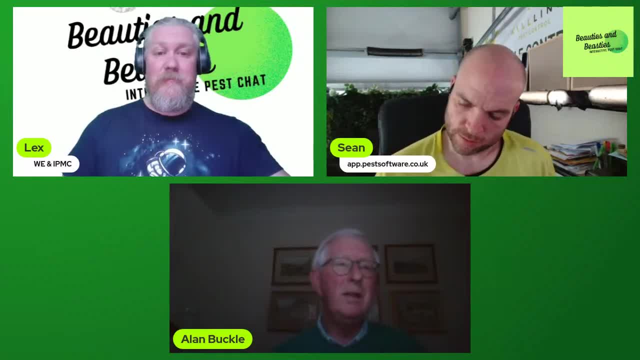 i i look to see. so that's our main channel of communication. um, we do rely quite a lot on the association, and the trade associations have us have a seat at the crew table, and so we do rely on them um taking the crew information and messages out to their members. but that's the process that 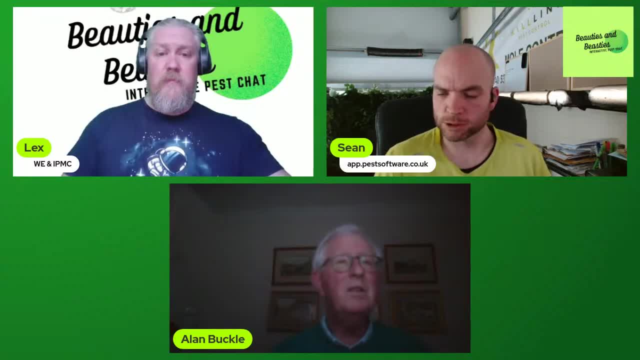 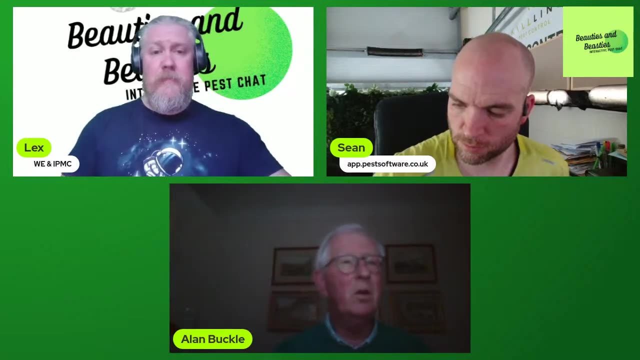 has has been operating. um. you're not the first that that said that and i'm not going to say we couldn't have done things better and i'm sure i'm sure we could. um, as you know, there's a new um chairman coming along starting on the 1st of may and i i know that communication is is very 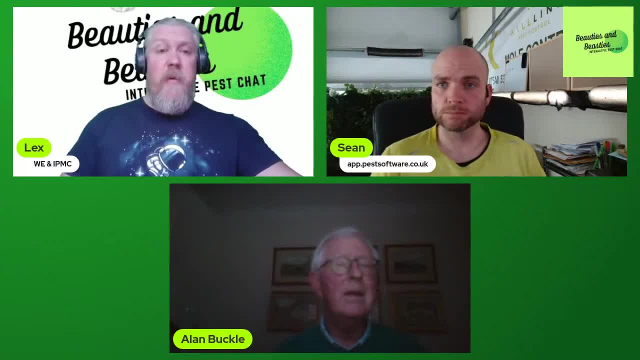 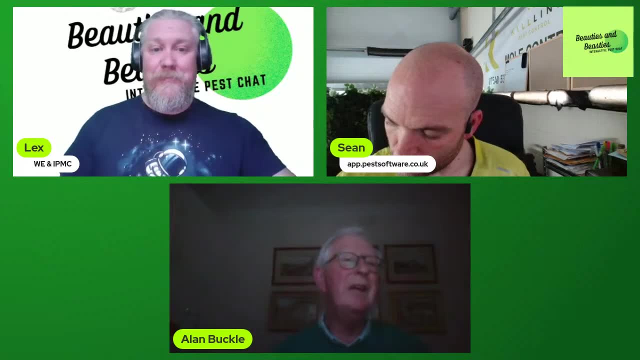 high on on his list. it's interesting. i mean we'll get on to talking about- i'm sorry, i was just. i'm just going to say let me ask you a question then. i mean, how better than that should we be dealing with and getting information to and information back from um professional pest controllers? 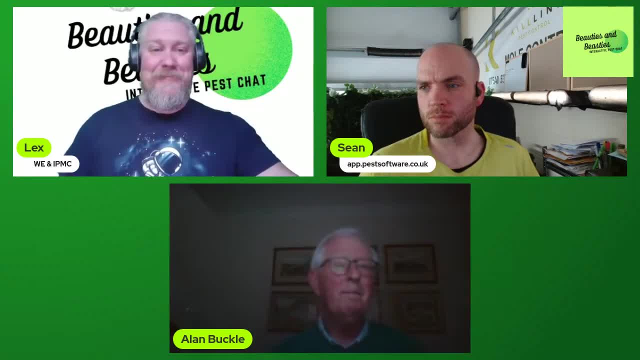 obviously i can't speak to every yeah, go on. well, i was about to say it's, it's, this, um, it's been a constant thought of mine and sean, i'm sure it's going to weigh in a second, but in our industry, you know, we have a third of people are bpca, a third of people are mpta and a third of people. 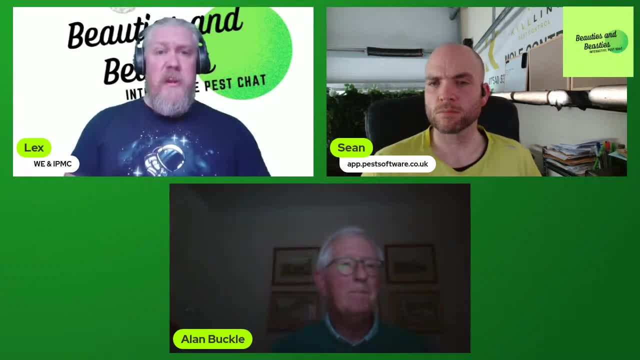 just are not affiliated at all, and of that probably you know, less than half of the pest control market um subscribes to the magazines of any various formats. so there's a huge gap in there. now i'm not saying social media is necessarily the way, but there 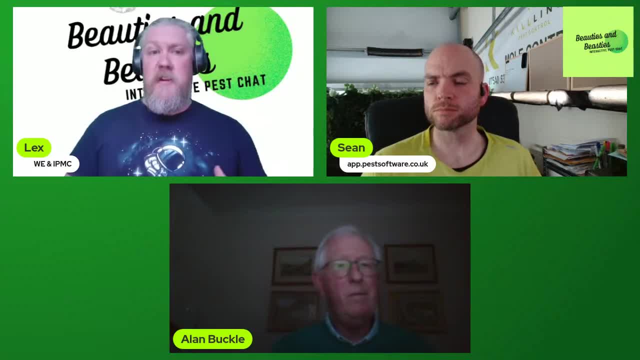 is actually very little on the way of um social media or you know, which is how a lot of people interact these days. alternatively, um better use of things like the distributors actually putting flyers and putting information in every pest control, the only unifying factor of every pest. 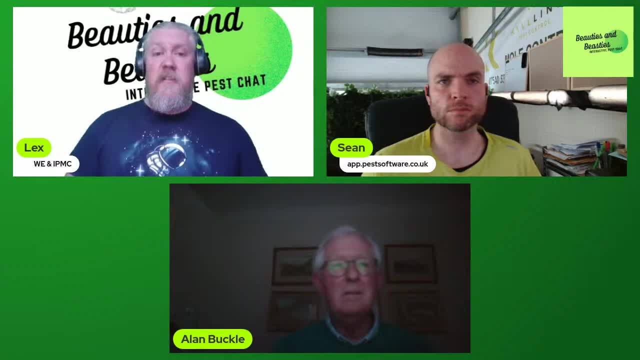 controller in the uk is they buy rodenticides and so with that, potentially a flyers out, you know, warning notices on your next purchase of rodenticides. just to clue people in. i'm not saying i have the answers, but um it's, we're a very fractured. 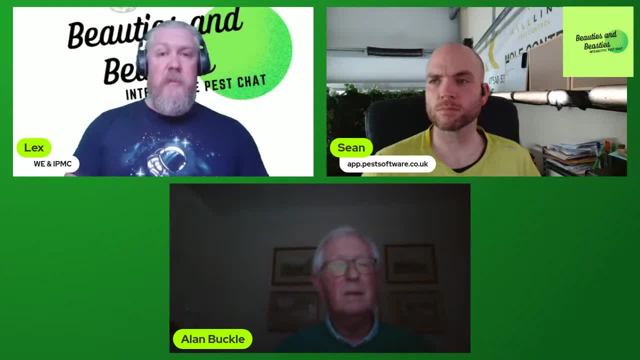 industry and it's it's having a single medium of communication is always going to exclude a huge number of people. yes, um, i mean what? the? the way you just described the sort of the segregation of the professional pest control industry. um, we've actually got three user groups, all of which 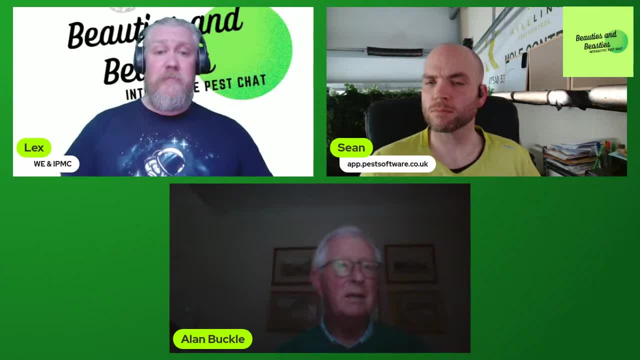 are gamekeepers and our farmers, um, and you think we don't do such a very good job to get to professional pest controllers. i can tell you we we do a much worse job getting to farmers because there are about 30 times more of them and, um, we don't get into their magazines very much at all. 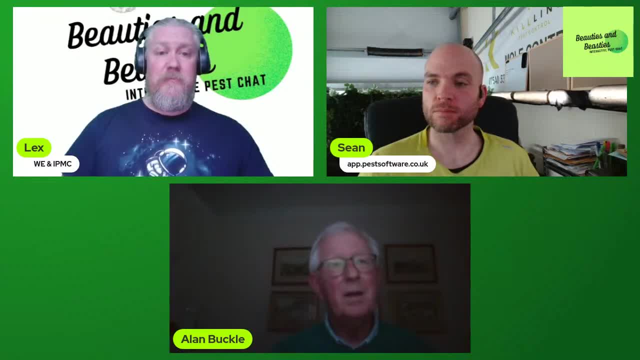 um, it's quite difficult to get anything through through um farmers weekly, or one or one of those. um. i can't say too much about communications um, because i believe there is going to be a significant change in crew communications um very soon indeed. um, i haven't seen it being. 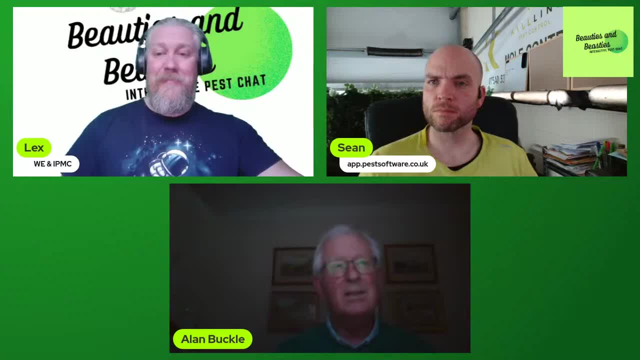 publicly announced um. so i i can't say anything in public, but i believe that things are going to change. all right from me. just listen to that. i think i absolutely get what you're saying about sort of disseminating it via the other um people, but i think from being an end user of the product. 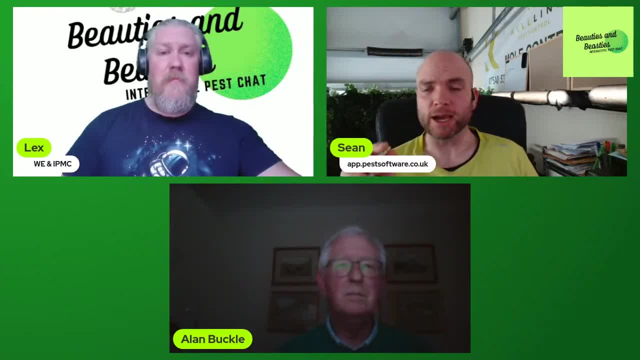 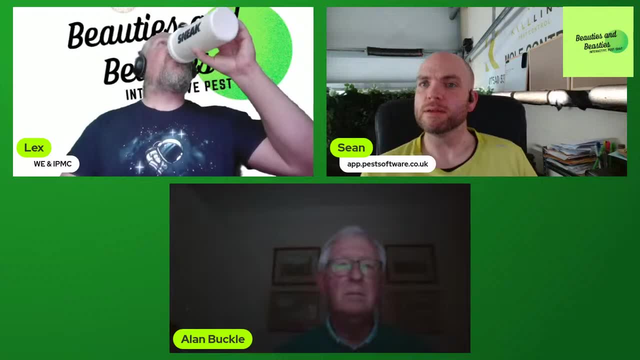 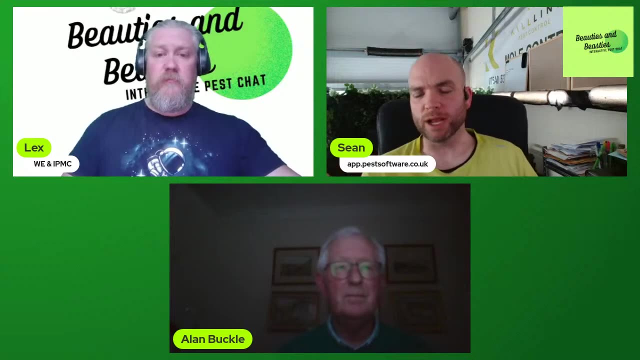 it almost feels like you're a second. i can understand why you're doing it, but it feels like you're like you're an afterthought, like we'll tell them and then they'll tell them. for me, i think if there was a facebook page for crew and that post was published, everyone would like that. 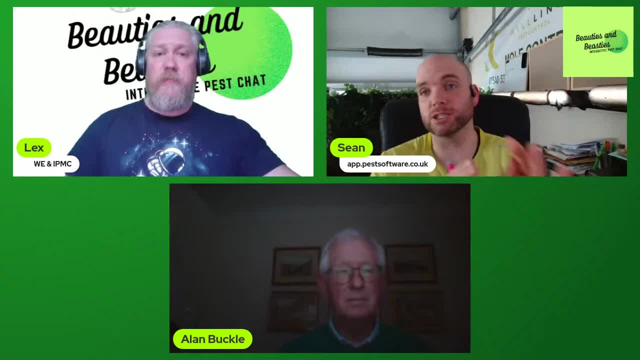 and then they would get that opportunity to put their comments on, to put their thoughts on. don't get us wrong, i absolutely understand that. that that would be a a blessing and a curse for yourselves and us, because there's always going to be one wally, isn't there? at least one? um, who's? 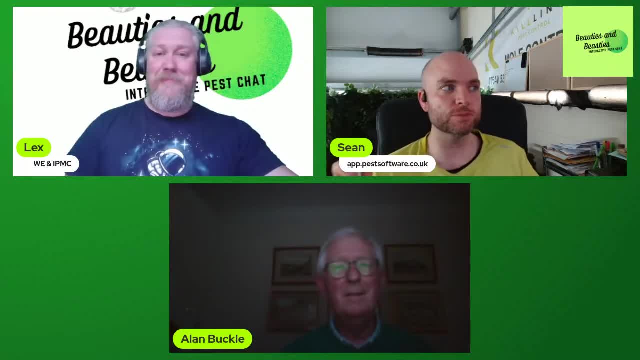 going to make comments, like you know, we know, you know like you're not stupid, but it would definitely be, um, a good way to get that feeling back, because even when the when it, when it does come out, you give it to them, they put it in the magazine, but it's it's sort of down the line and then, as you, 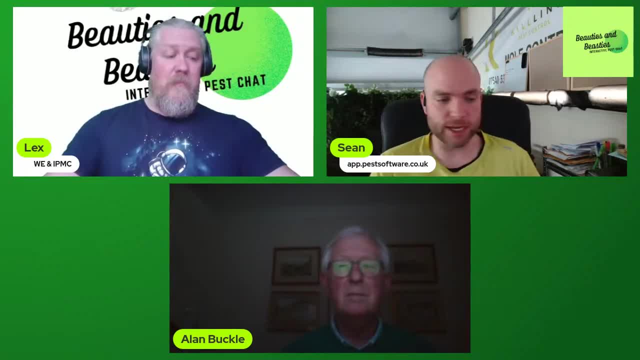 say there's no way to get that feedback back. and in today's day and age, everyone's attention is on this. you know, nobody reads a newspaper anymore. they watch that, they pick up that, um, they pick up that phone and they look at it 24: 7.. uh that. 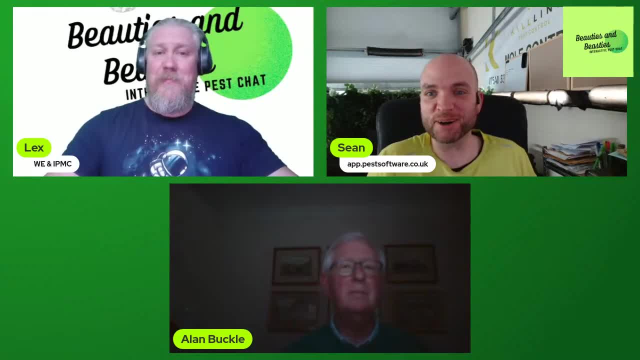 but, as you say, there's a new guy coming in and it might all change tomorrow, mate. well, it's going to change tomorrow by the sounds of things. well, yeah, yeah, not, not, not just the chair, yeah, but, but, but, but also the communication. we, we are very aware, well aware, that crew has been incredibly slow to get onto social media. 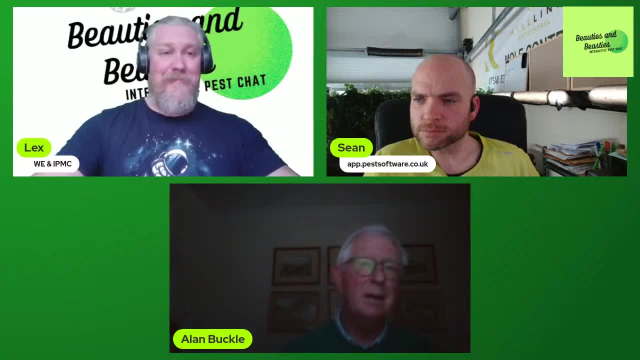 um, i've been trying to get that picked up in crew for a long time- um, i don't know how many years years that there was a reluctance to go into the social media just because of the the amount of traffic that you had by a single post. there was then an agreement: dip in the social media. 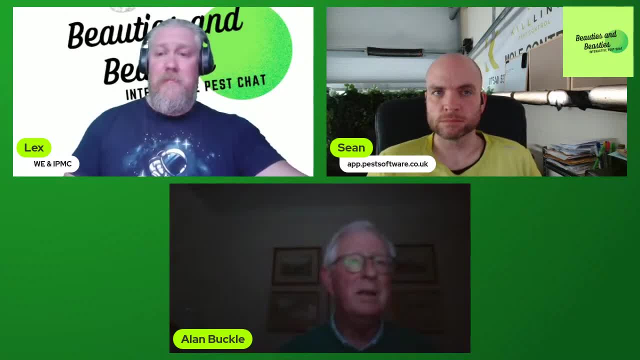 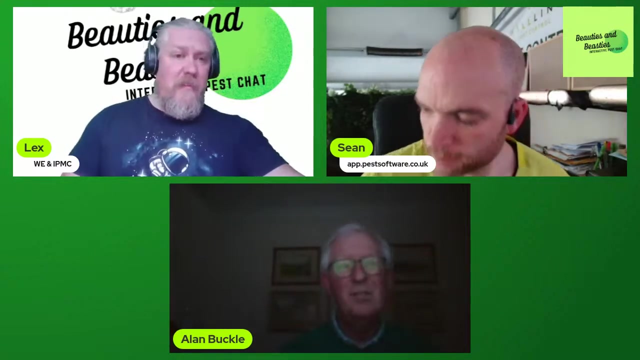 water and I believe, well, I know there is a twitter or x account for crew and that that's the only social media that we use, but I always change. that's coming is going to look, absolutely going to look at that, and so there will be some movement on that. so, and I'm afraid, it's not very satisfying. 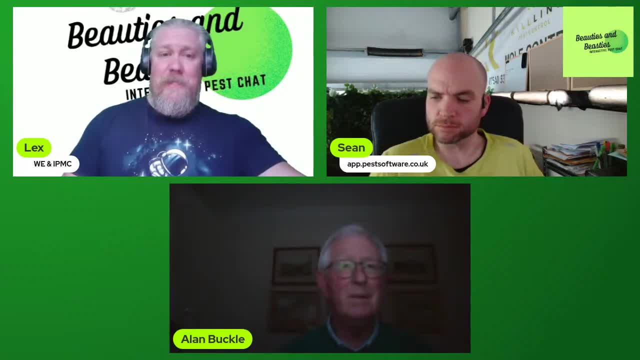 to watch this space thing. so I mean it's interesting you bring up farmers, because farmers are a interesting discussion point with a lot of professional pest controllers and it's a bit of a sore spot as well that it seems as though a lot of pressures from regulatory changes and a lot 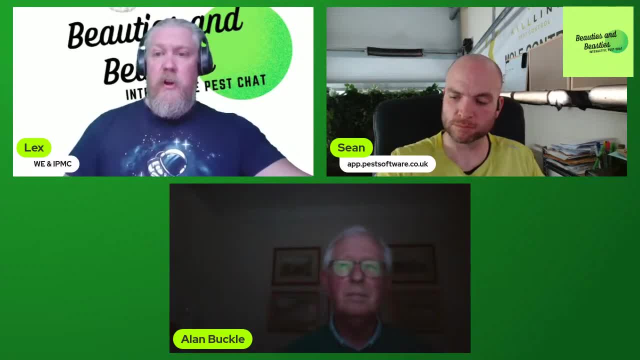 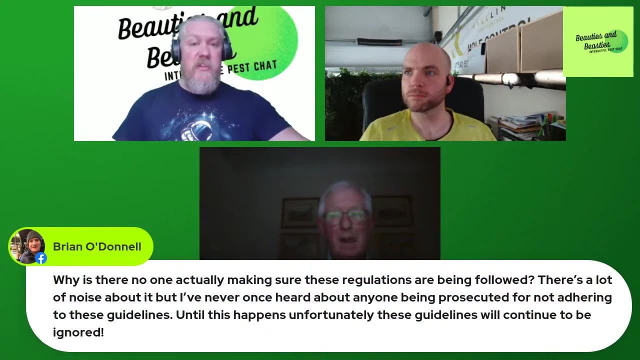 of pressures from, you know, industry bodies fall on the professionals and yet at the same time, it feels as though these other user groups largely get away scot-free. and to quote someone here, Brian O'Donnell. he says that why is there no one actually making sure that these regulations being 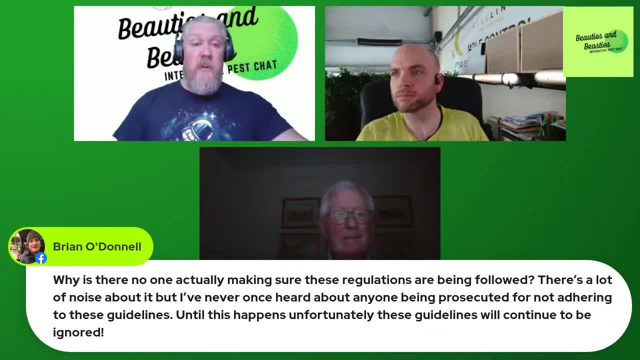 followed we? we do it to the best of our abilities, or most of us try to, but we do it to the best of our abilities, or most of us try to, but no one seems to be held accountable- the other user groups- for the issues we're identified, and 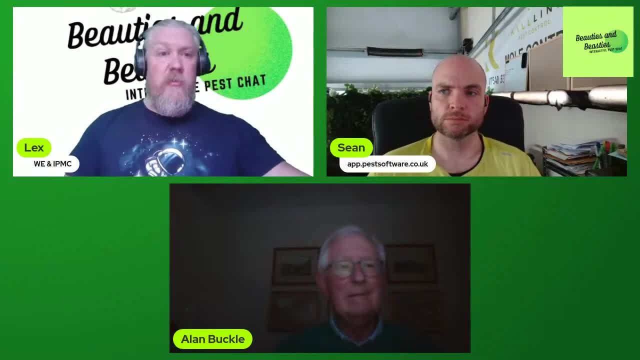 specifically when we are looking at things like the escars residues, which we'll talk about in a minute, because that's a whole, whole other story, isn't it? well, it is. I mean, the question about enforcement is again something that is incredibly important. there is a whole department in DEFRA by a whole department in England who are there to 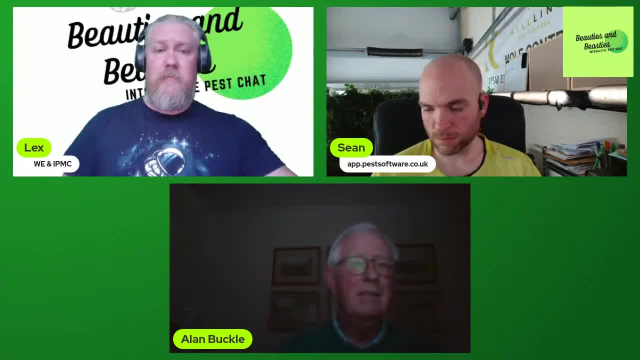 prosecute or detect and prosecute people who use pesticides or abuse them, and particularly rodenticides get misused and abused. there are these enforcement bodies. they they are very much overworked, they don't have enough resource and I just wish they did. whoever that that person was was saying that there's no prosecutions. 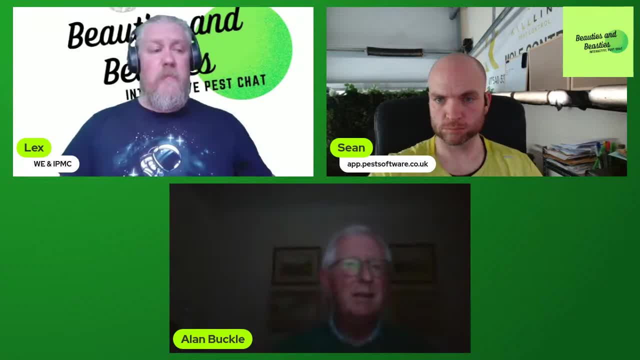 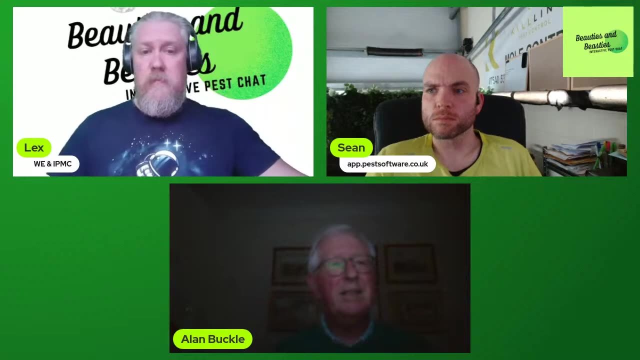 there most certainly are prosecutions. there are nowhere near as many as there there might be, and I wish, I wish there were more the. the problem with this, with this whole issue, is that the effects of these rodenticides are though if a bird of prey is exposed at a particular site. 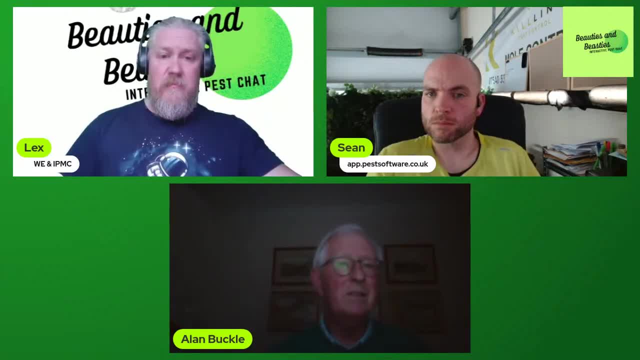 it's, it can be 20 miles away when it's when it's found dead and so someone picks it up. it goes into the wildlife instance investigation scheme. it gets his liver analyzed. they know what killed it. but then someone's got to go to that site and try to find out where it picked that up. 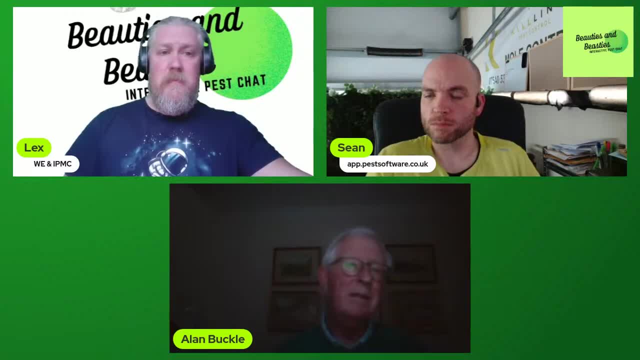 and that's almost impossible to do, and so the the, these government agencies have their own sort of crown prosecution service. they're a bunch of um? um legals who look at each case and and look at the chances that they they may be able to press the case, take them to court and have a reasonable chance of prosecution. and it's incredibly difficult. 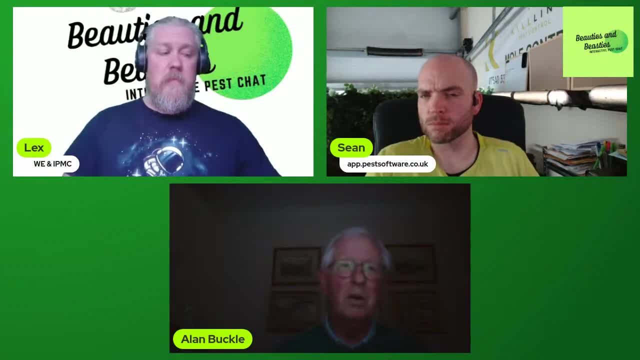 to get um evidence that stands up in the court of law. if someone managed to kill a buzzard or a or a white tally, that they got the guy who did what the um, he got the guy that did the white tail eagle, because they just threw everything at it. but it's, it's a, it's a. 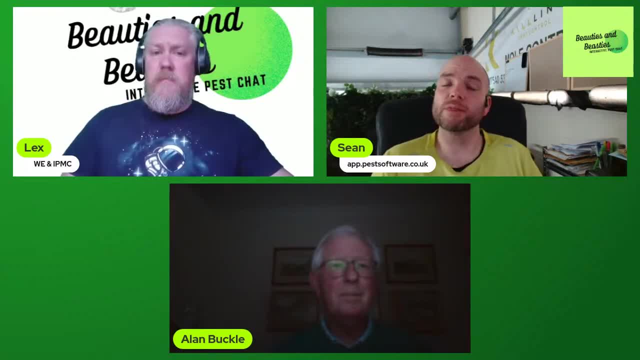 very difficult one, but are we not? are we not thinking like too extreme there, in that there's going to be a very, very small handful of people who are a nightmare? that being said, is it- is this not just a case that the auditors need to be better informed, better educated, um better at their job? so when? 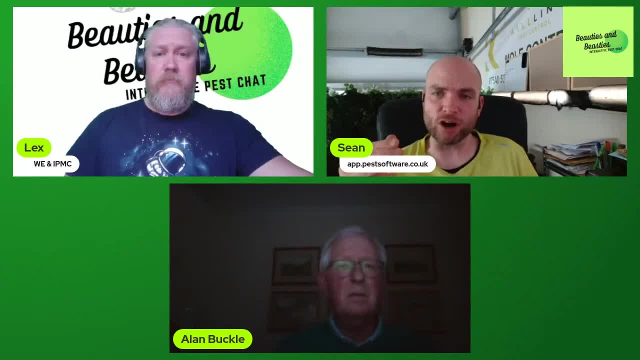 they do turn up on farms. they can go around and get the farmers to feel their audits so that they know the type of things that farmers are going to do and they know what to look for. they understand how poisons should be used and shouldn't be used. that they can identify the poisons they can see. 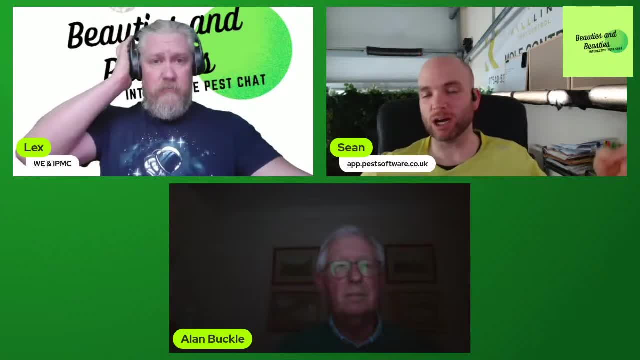 the difference between harmonics, cilantro wheat, how much should be in a box, etc. and then actually get them to feel their audit, so that the farmers are in a position where they're like we're going to have to do it properly, otherwise we'll fail the audit. it's not just about having the paperwork. 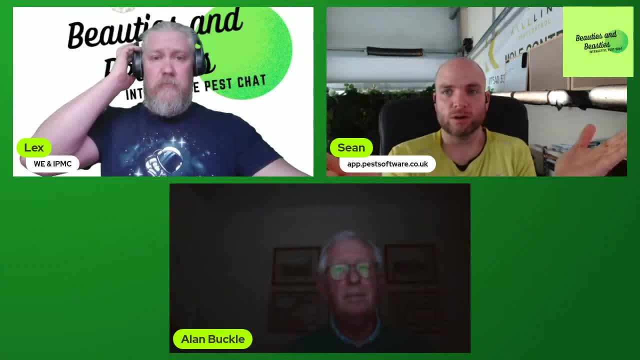 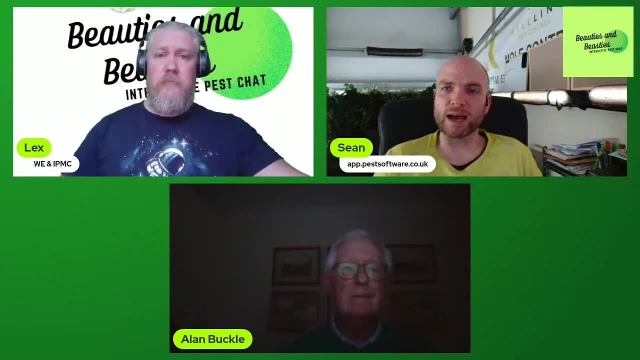 correct, because that's all the auditors do, isn't it? they go out, they look, they go like that, yeah, yeah, no, they never. they never do any searching or anything. and you can get a non-compliance for paperwork, but you'll never get a non-compliance farm and poison lying around where birds can get to it. 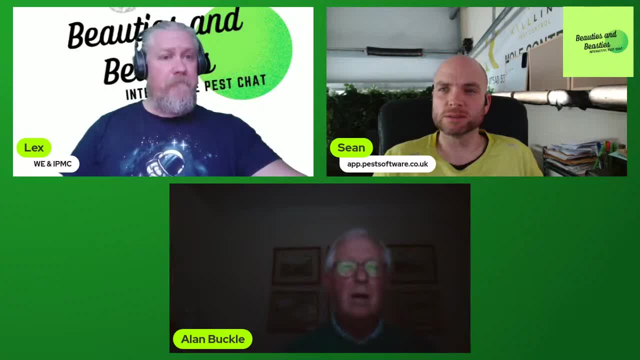 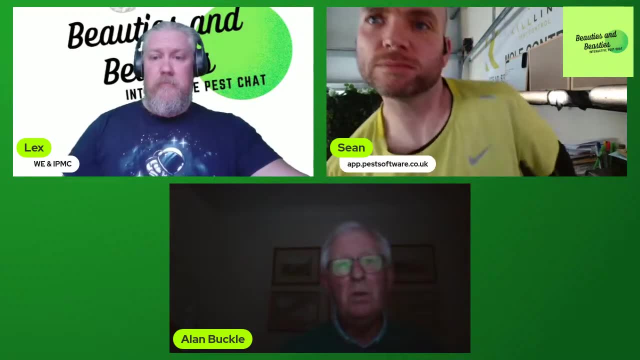 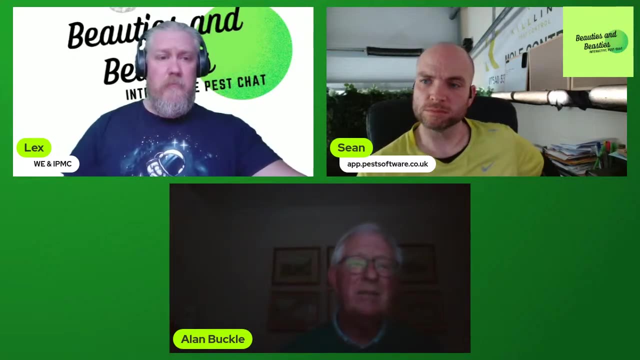 well, that certainly should should be happening. we we work with all these farmland schemes. they've got requirements that we put as crew into all of their, their their standards. i think about 70 farm and shoreland schemes went through a process with us where they integrated into the 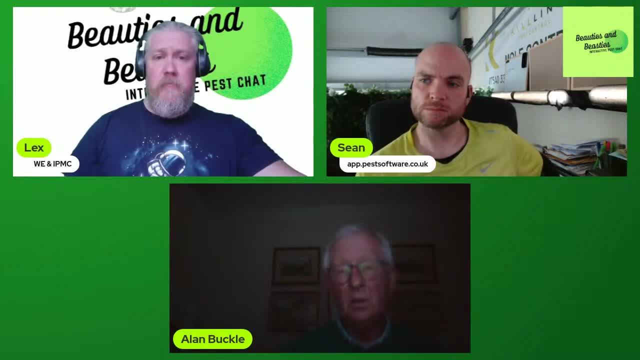 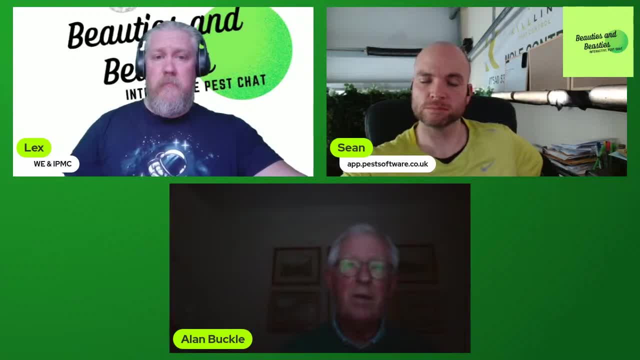 failed their all of rodent pest control. and you know i don't want to give a load of of excuses on on here, um, and sort of try and get away with it by saying, well, it's, it's very complicated, short, i'm very sorry, um, but what, what? what happens first of all is the auditors when they go onto a farm. 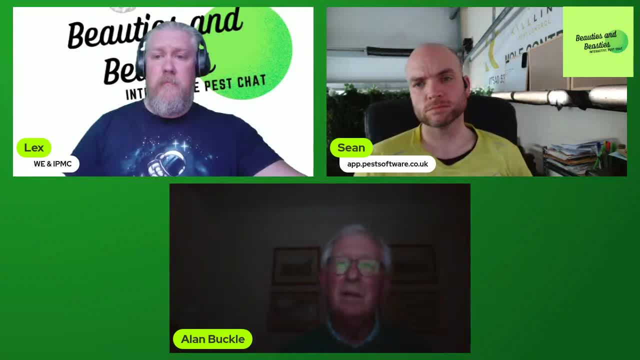 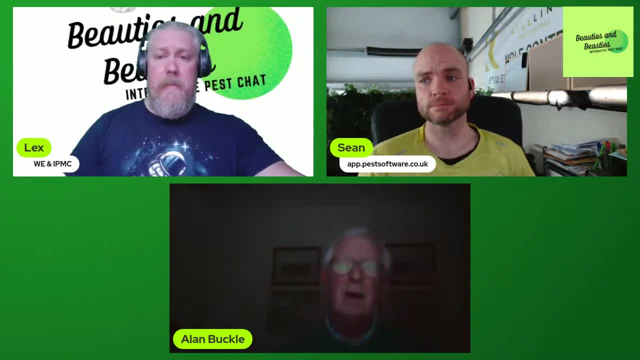 um, but also what happens is the farmers fail their audit, um, and they're given a certain amount of time to put things right and an auditor comes back and checks it has been put right and then, and then the farmers go back onto the scheme. um, we try to find out from all of these. 17. 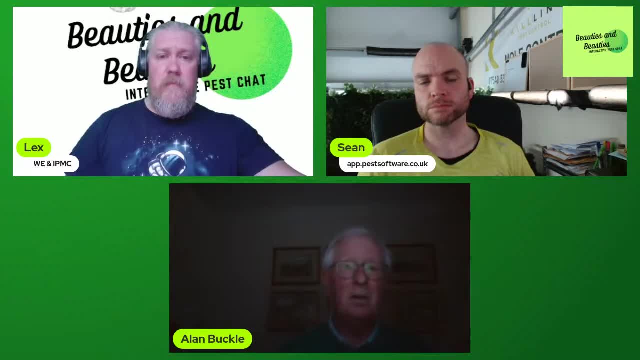 crew approved farmer shoreland schemes. exactly how many farmers fail their audits because of failed rodent control? um, but the farm assurance schemes are very reluctant to release that, that, that information. some of them do and and and some won't. they say it's confidential information that they hold between their members and their them as a farm farm assurance scheme. but um, 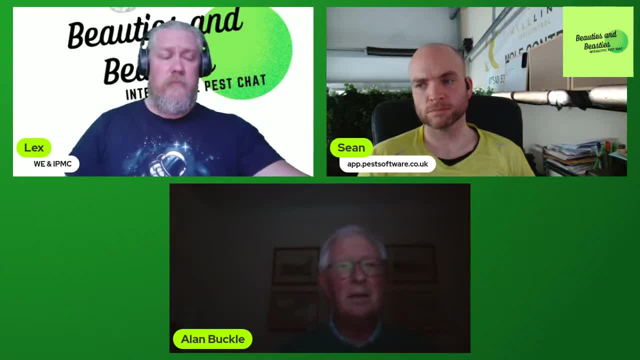 somebody should be looking on every one of these, i think, uh, 80 000 farms that are audited according to crew code of best practice, and they, they should be looking at them and they should be looking at the record. for what absolutely can i sorry, can i just ask one quick question now? why do we have 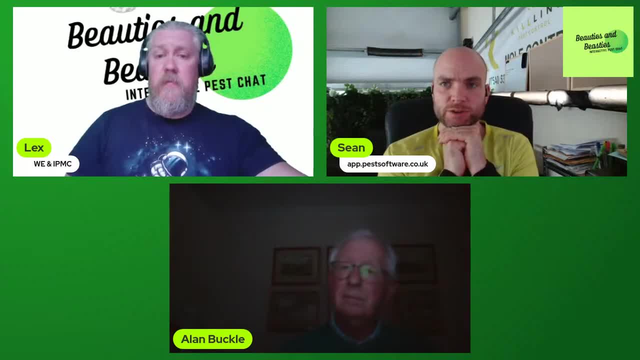 or why does it appear that we have different levels of users of professional um rodenticide? so we have pest controllers, farmers and gamekeepers. the farmers and gamekeepers seem to be lumped into the same process that they have to use, and pest controllers have to be lumped into. 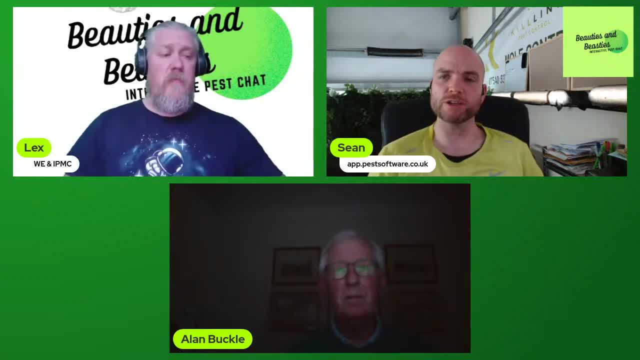 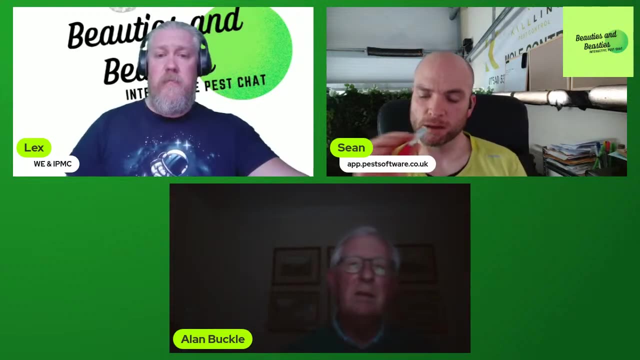 something else. if you using the same product, why? why don't we just all have exactly the same stipulations and specifications on us for being able to use them? um well, from- i'm trying to get my date right- but from the 1st of january 2026, that that that happens? we we have. we have made that change. 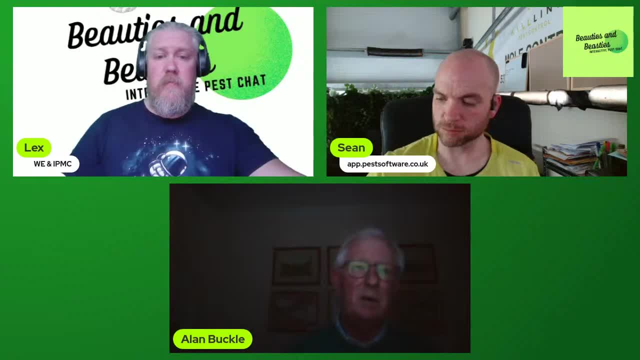 um, and everybody will have to pass um or or take a course, pass the exam and get a certification um from an off-call regulated training course, and the farmers and the gamekeepers need to do that just as much as um professional pest controllers do um, so there. 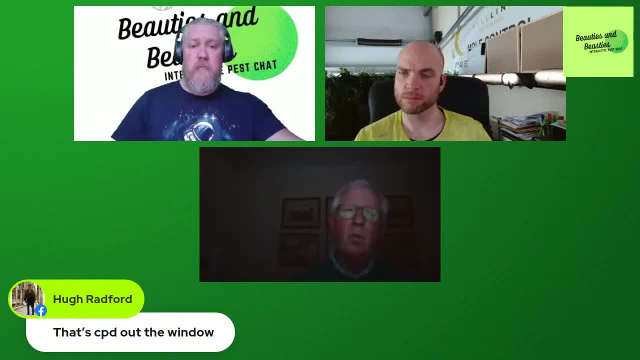 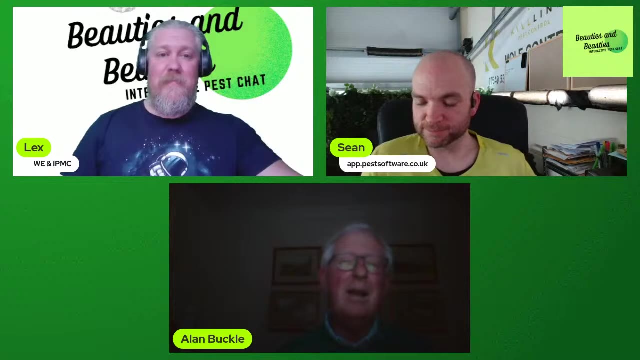 will be that level, level playing field. when we, when, when we, um, i'm, i'm assailed by questions in all, in all directions, um, about cpd out of the window, i'm, i'm, i, i could, i can come back to it, um, and we can do all the research. why not now, um, so yeah, so i'm sorry i've i've lost my track a bit. 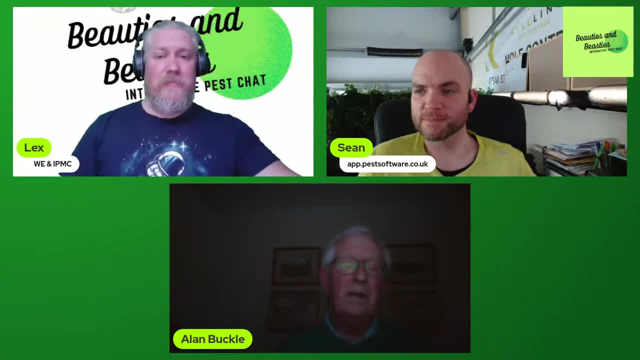 now, but um, we want everybody to be trained in exactly the same way. professional pest controllers um do much more in pest control um than just control rats and mice, and so their training is much broader. and the rat and mouse bit of it is um, it's not a one-on-one thing for everybody, but for 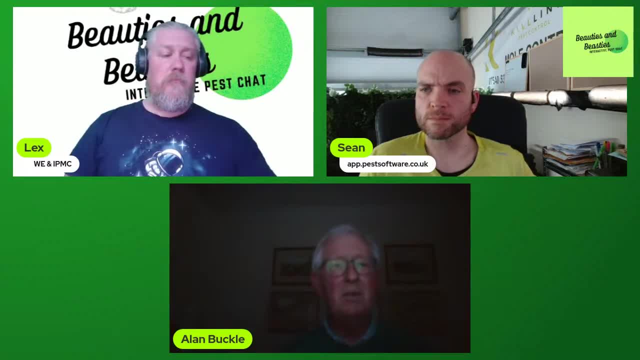 it is a significant part, but it's only a part of it. farmers and game keepers only want to know how to control rats and mice when, when they want to buy a rodenticide, they don't want to be trained how to do fleas, cockroaches, bugs and all those. so we have created specific um single training. 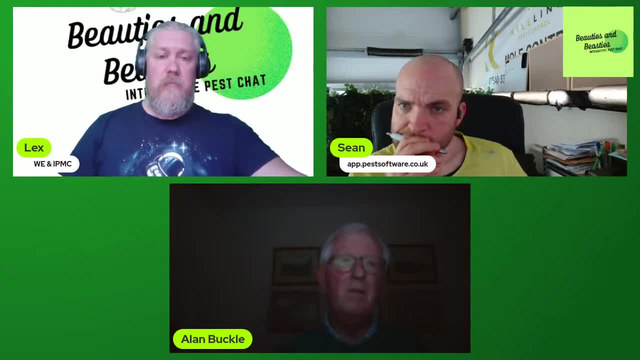 courses that deal with rodent control for for everybody, and everybody can take them, but they are there for farmers and for game keepers. so the answer to your question- and i'm now i'm being long-winded sean- that there has been for the last years. 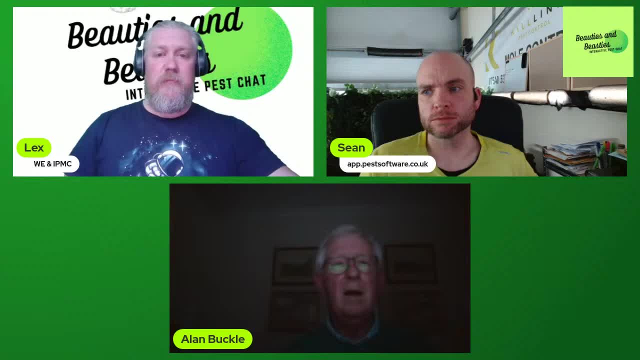 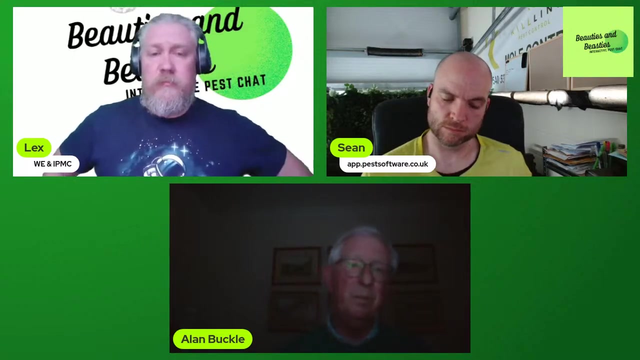 a way for farmers to buy these pest control, um, these professional rodenticides, without taking a formal course, um, and that is, if they are members of a crew approved insurance scheme and the membership certificate was their proof of competence which allowed them to use these and buy these professional rat baits. we, we've, we've put an end to that. 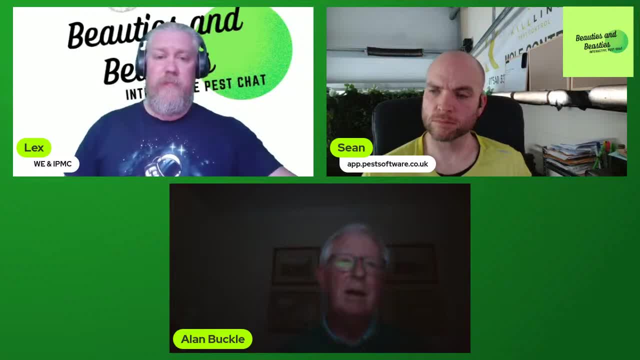 and that is is stopping. we we've given every farmer two years um on the 1st of january this year um to take a course and get qualified or they won't be able to buy a professional rodenticides anymore. but does this not leave us in a position now where i've got 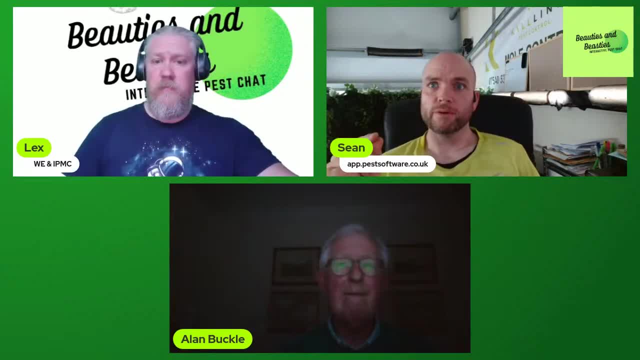 i've got two lads who work for me that the reality of it is i can drop out of a cpd scheme, i don't have to do it, and i get them to do a course- uh, like an 80 quid course every five years. um, so like dale done his, dale done his level two two year ago. so i don't need a cpd. 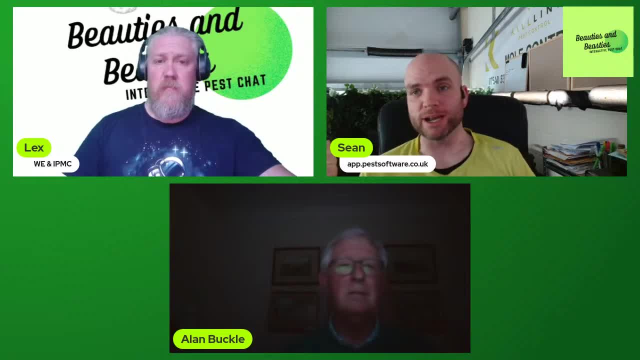 scheme for him anymore. um, alice's will probably be running out next year or something, so i could. i could then put him on basis from them, but then it's only going to cost two years, like 80 quid, so effectively over 10 years from start to finish, like my lads could end. 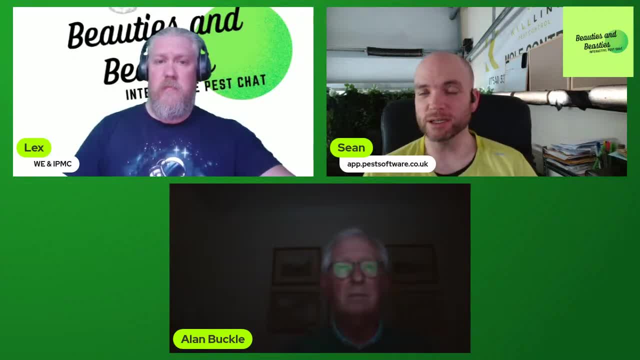 up doing like i don't know, maybe four, six hours worth of training to buy rodenticide, which which to me feels like pest control going backwards, not going forwards. um, yeah, the cpd thing is it is. it is strange to me. um, so you don't want your guys to be kept up to date with all the things that they need to? 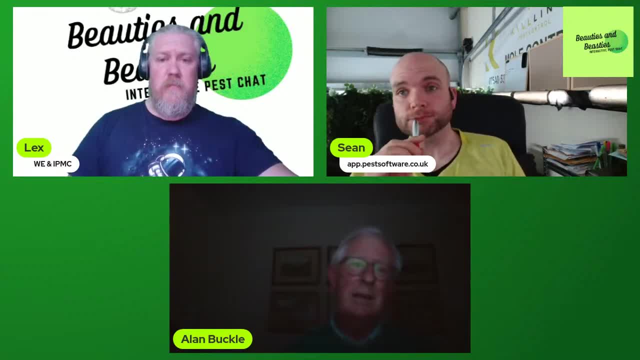 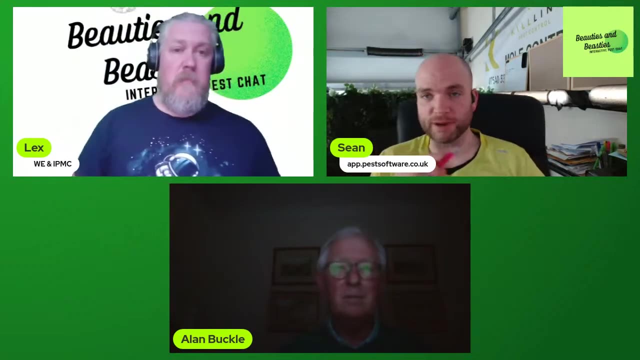 know to do their jobs properly. so you're gonna take them out of a cpd scheme and save a bit of money and they're going to be, um, not doing cpd while they're working for you. i that seems a very short-sighted way to do it, just just to qualify. we will never come out of a cpd. 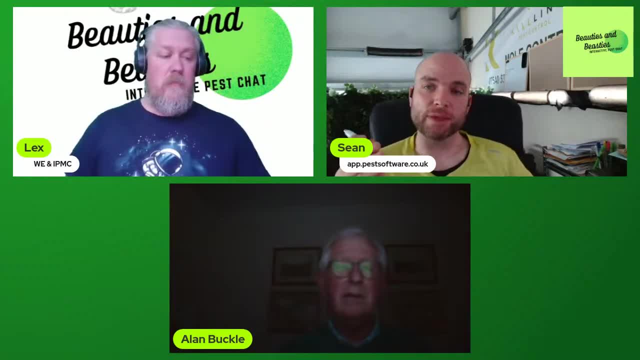 scheme. we will continue to do it, but i think that there is a lot. i think there is a large number of pest controllers who will turn around and go. this is a brilliant opportunity for us. we don't have to worry about cpd points anymore. we don't have to worry about sending. 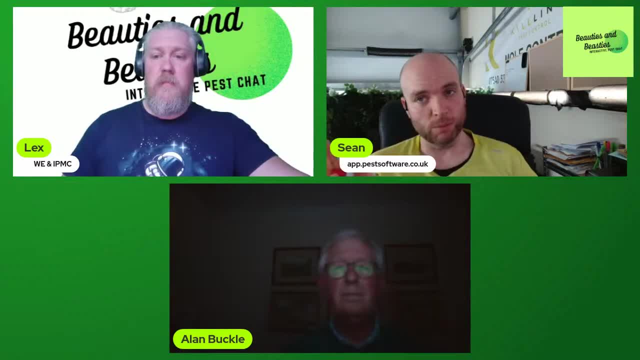 them on things. we get them an 80 quid ticket every five years and we can continue to get them kick boxes, and i think that's what will happen. i agree with you. and if we were all going to continue to do it? but then again we're in the same position where, for whatever, 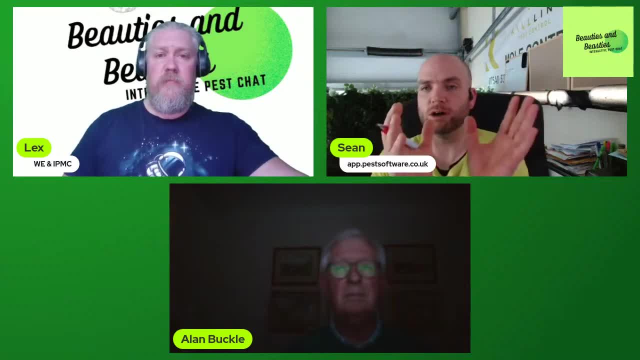 reason we're separating pest controllers or doing pest control. we're separating pest control. we're separating pest control. we're separating pest control on farms and farmers doing pest control on farms. the rules should be the same for both groups. so, like: why i don't? it feels like we are going backwards, not forwards, and i'm sure 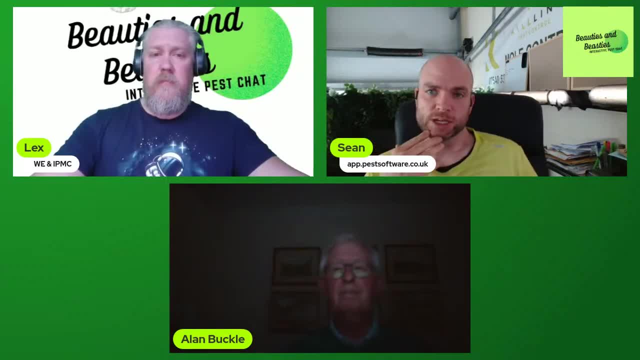 i'm almost positive we will see um firms that turn around and say we'll just get them to do an 80 quid course every five years. i'm almost certain that will happen. um, in fact, i can think of two straight away off the top of my head that will jump at that opportunity. 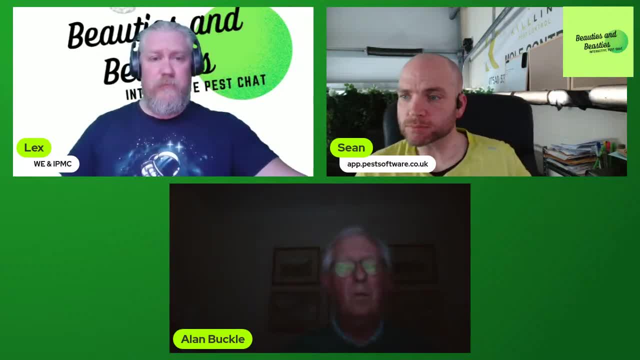 um well, that that um was an unintended consequence of a decision that was made in crew in the training and certification work work group. um that we decided that um. so i mean, who makes um cpd compulsory? then as far as i i know, it's not compulsory. 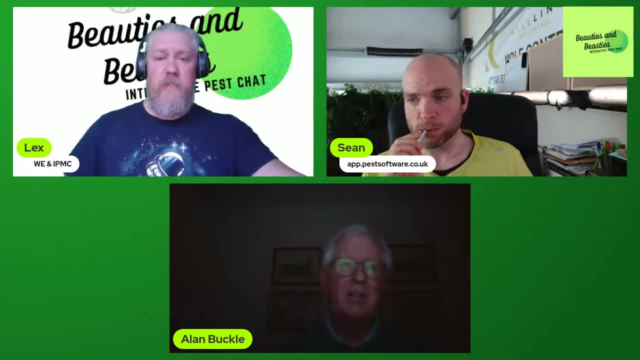 to anyone: um, some of the trade associations like, like bpca. if you want to be a bpca manager, you have to be a bpca manager. you have to be a bpca manager, you have to be a bpca manager member. um, i believe that it's compulsory to be a member of a cpd scheme and i i think there are. 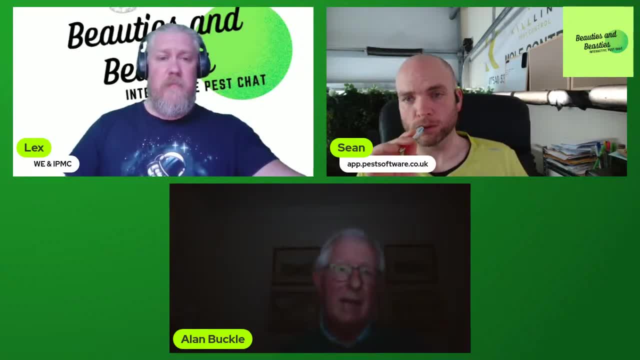 certain parts of mpta, that, that, that, that, that is the same um, yeah, i, i, i think this is something we need to think about very strongly and i, i know, i mean, i, i've heard this, um, i heard it for the first time at pest x a month ago and it's something that we've got to deal with. sean, that that is not a good. 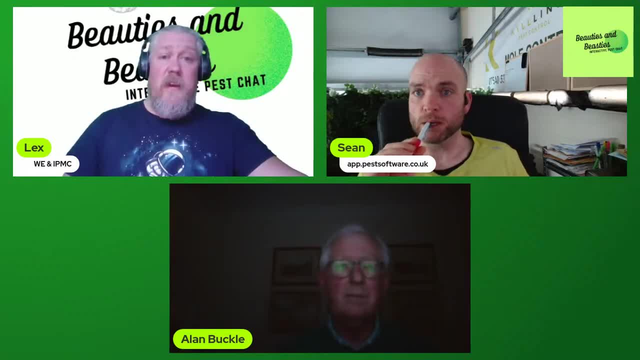 outcome from that. i think it's something that we need to think about very strongly, and i- i know i'm from that process, yeah, and this is it. i mean, um, we are, as an industry, those, you know, those who are wanting to do things right will do things right, but there'll always be an element of um. 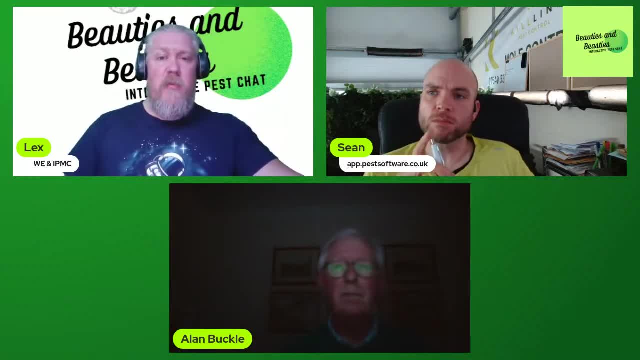 summer grapes is the wrong word, but you kind of know what i mean. when you watch someone else um flout the rules, you know. uh, proudly announce that they haven't done a day of cpd in their life and next week they're going to redo their um level two. and hey ho, um, there we go. 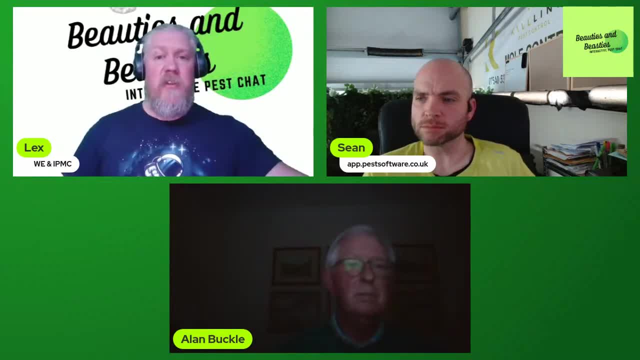 and it's really galling because a lot of us, the majority of us, want to do things right and we don't want to be tarred by the same brush and so, as sean says, we very much feel like we want to have. if there's one rule for us, then it's one rule for all and and we should all abide by it, and 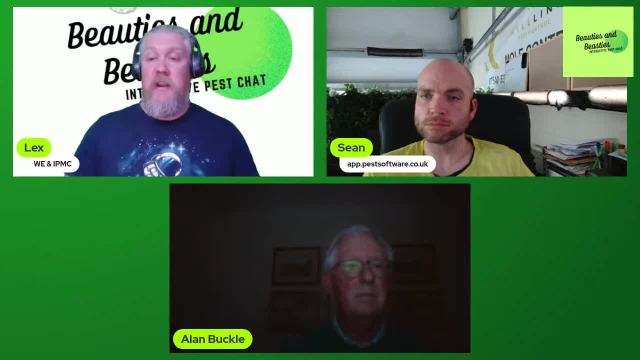 cpd is and arguably, and nobody will, i think, disagree- agree, it's a good thing and as uh, there we go, uh, it does bring on to bigger things, and i will talk about the elephant in the room and, because i want to, i, i i'd like to hear your thoughts on this, alan uh, as well, which is: 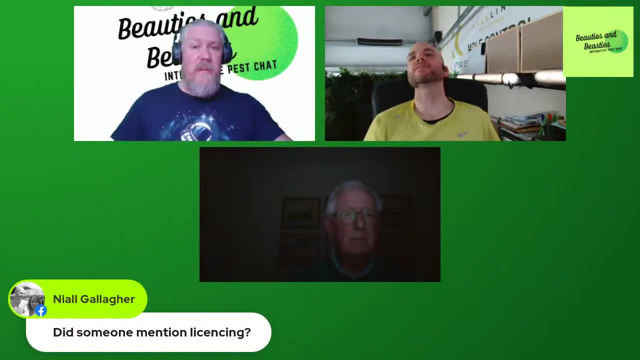 the thoughts around this. did someone mention licensing? there we go. i mean, it comes up all the time, alan, if you haven't watched these- and it always turns into a total nightmare because it's so divided on licensing- just some love it, some hate it, and it turns it. 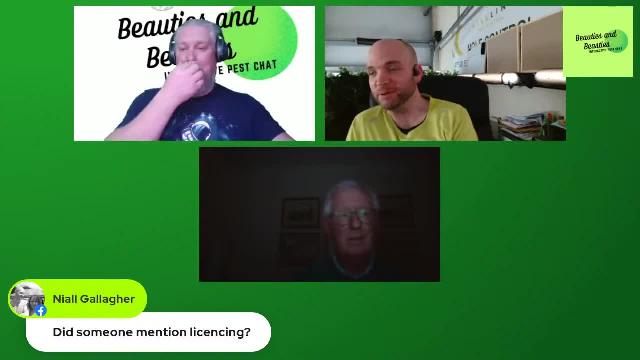 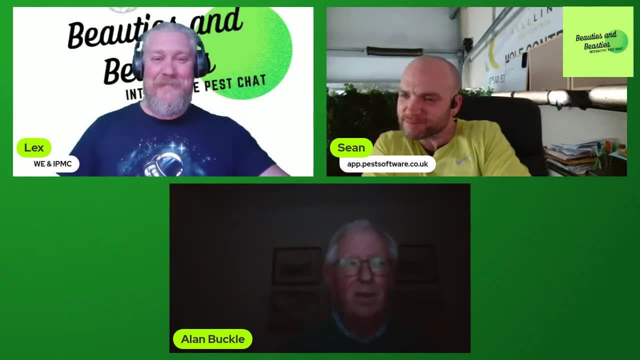 so, whatever you say, just be warned: there's going to be people who love you and people who hate you. um well, i don't really know what to say on that. um what. what to say on that? um well, i don't really know what to say on that. um what, what? 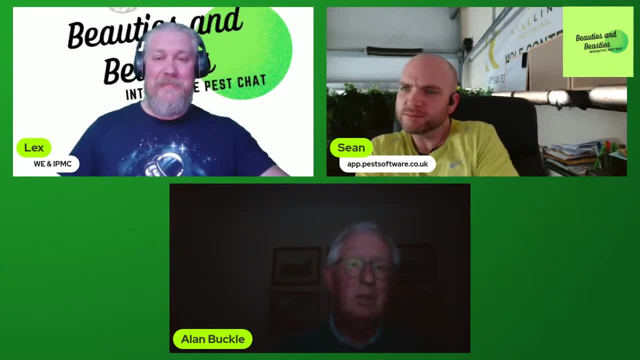 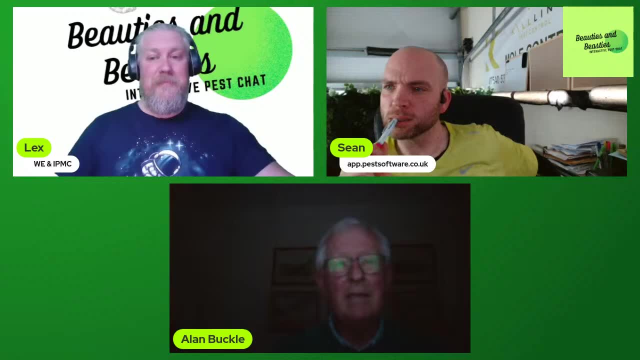 when we started, when we started, um, stewardship, um, we started to have some meetings with with the government side, um, and and everyone was was feeling around not really sure how they were going to put this stewardship regime together. even the government didn't really know what to expect and and so, and so they, they were making decisions on on the hoof. 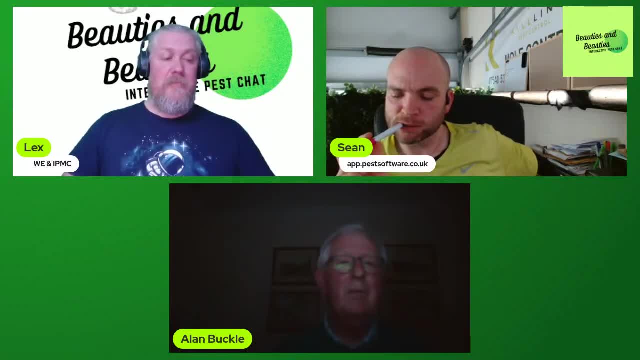 but very early in the play um i went up to london and met some of the top guys in in the health and safety executive and i went with the chief executive officer of bpca and the equivalent of mpta and we said, if you want us to um run a stewardship regime, um the thing. 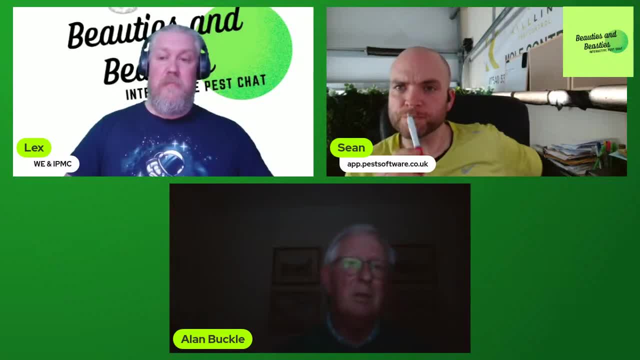 that you can do to help us is to establish a licensing process for professional pest control in the uk. um, we explained that. so many of the countries in europe that you say the same pesticides in the uk. um, we explained that. so many of the countries in europe that you say the same pesticides. 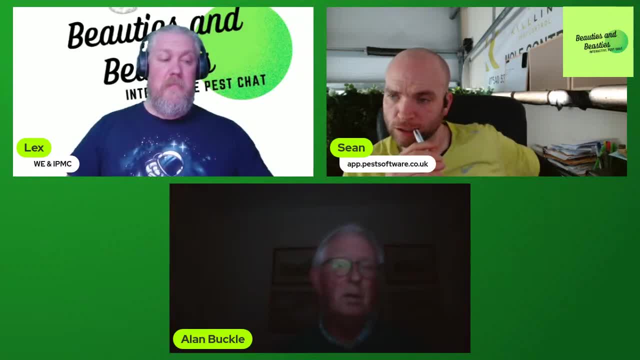 in the same ways they, they, all of their um pest control, um businesses and industries are are licensed um, and we were told at that meeting and we've been told whenever we've mentioned it since, um that government does not want to do it. it's it's an issue um, it's a fundamental, fundamental. 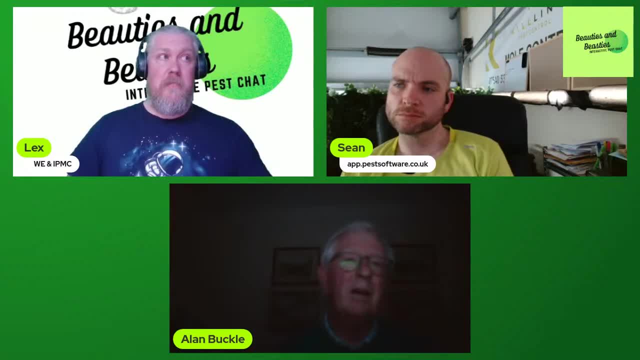 issue in in government um that they are are that they don't want to put more red tape um across um industry and manufacturing and and so on, and so they they don't want to be seen to to be applying more cost and more official red tape into people's lives um. and so we decided um the 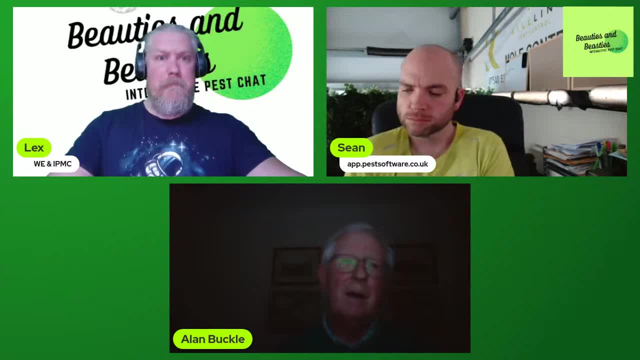 comments. i mean getting obviously- is about amateur use and general public. we can never fix anything but the other thing they do. but the other thing they do is that they don't want to put more red tape into people's lives. um, and so we decided um then, and there right up the start was um we were not expected to deal with. 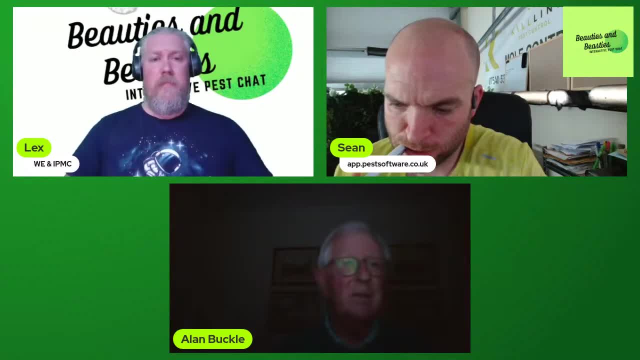 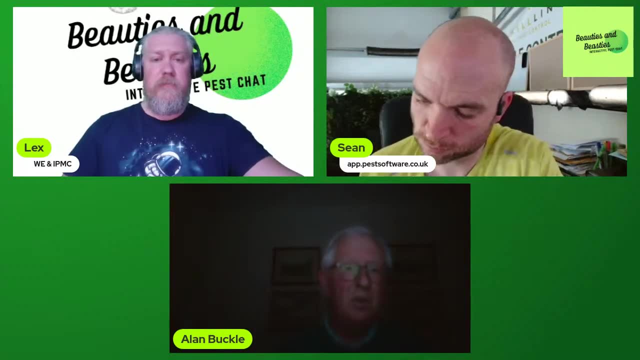 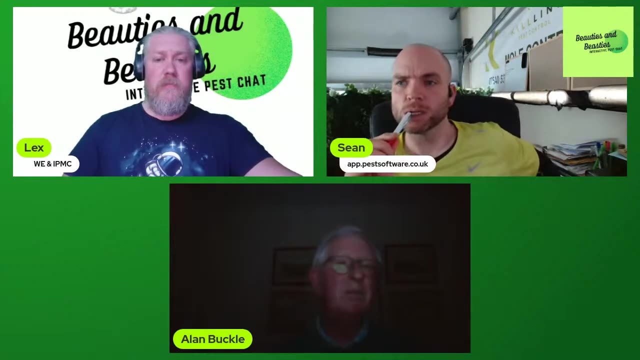 um amateur baits and it was just not our remit. we we needed to keep out of it, and it was also made clear that the government had no intention whatsoever of um stopping amateurs. whatever you want to call them- amateurs, non-professionals- the general public is the. 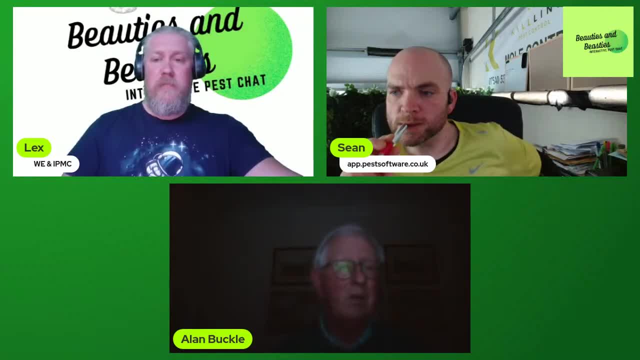 regulatory term. these are the regulations that are going to be put in place. that are going to be put in place these days, um that they were not prepared to stop um the general public buying very small quantities of very to troll infestations of rats. they were not prepared to to to to do that. and each time i go into a review, 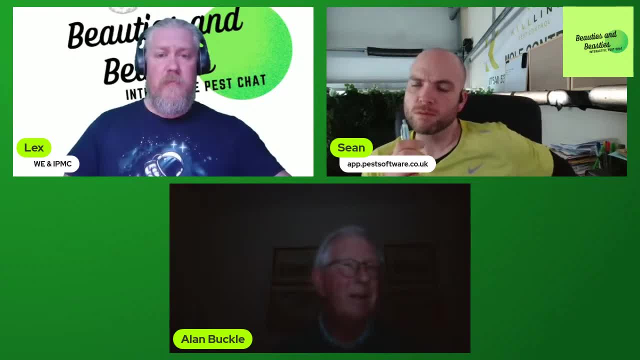 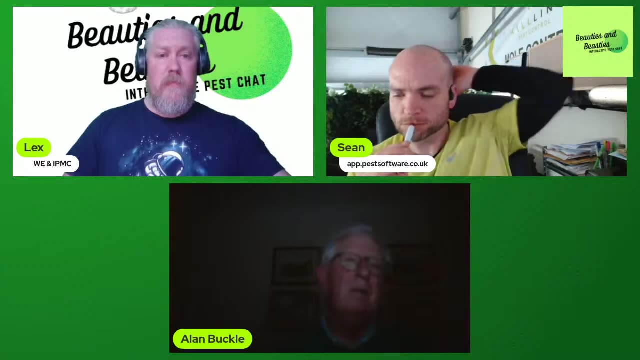 with government and say we haven't met our environmentals, but in fact we haven't achieved anything at all. and i say to them: um, please don't forget that. um, you decided that you didn't want to license professional pest control. you have decided that you don't want us to look at amateur use and 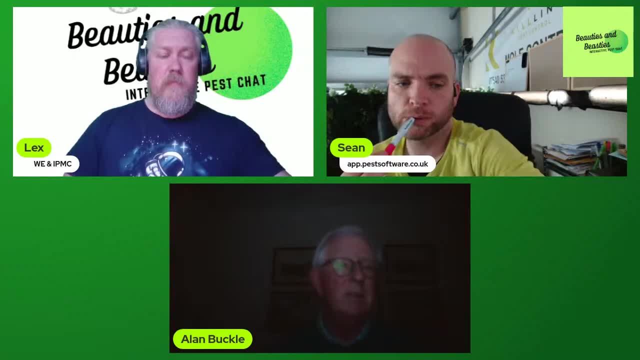 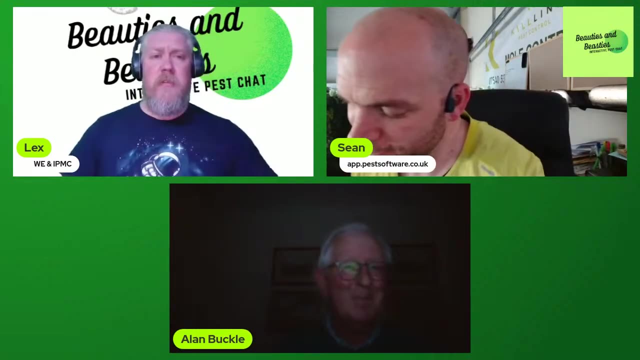 that amateur use is to continue and amateur cells are to continue. so that's that. that's that's pretty much all i can say. can i, yeah, can i, ask you a question? um, um, um, a question? no, no, no, no, you're going to, you're going to. i mean that. that was. 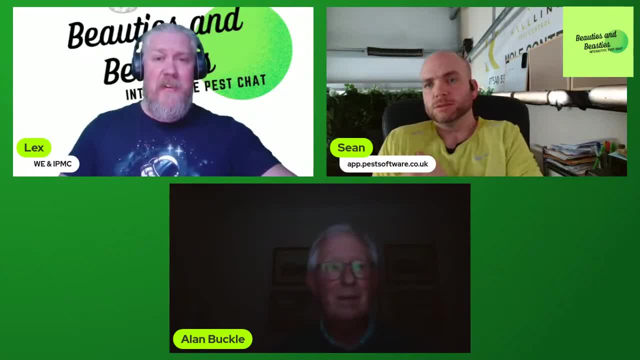 that was quite a lump there, wasn't it? that's a lot to digest, isn't it? so go on then. yeah, i was going to say the amateur use thing. i know everyone's going to talk about it, but the reality of it is it's not in your remit. you know that. if they want to ask people about amateur, 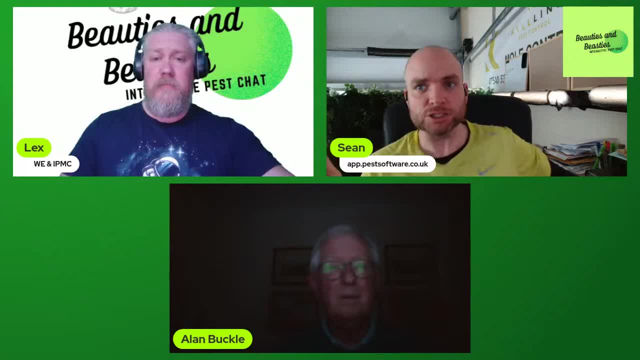 use. you go to the government because they didn't give you that to look at. so you're not responsible for that and i think it's unfair for us to try and haul you over the calls for something like like as an industry- i don't mean me- and lex, i mean as an industry where you're not. 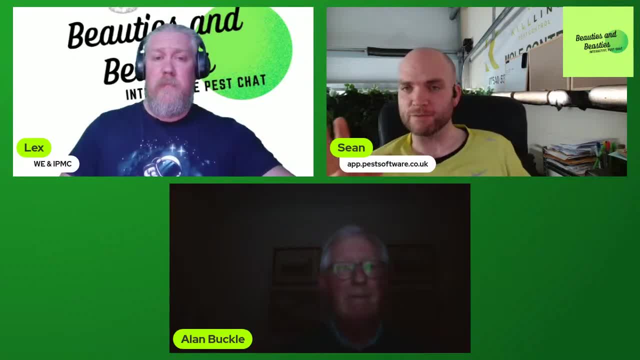 responsible for that. i think we need to stress that, because everyone, everyone, thinks that you are responsible for redentor sites, but it's only professional use, isn't it? it's, it's absolutely only professional, professional organ size. when stewardship started and government decided to keep us out of the general public, what was just happening at that? 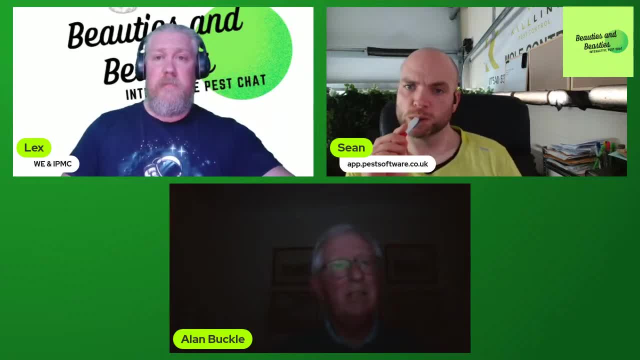 time that they were making pretty massive changes to the availability of rodenticides to the general public. um, the the quantities that that could be purchased were, um, i think was used by a factor of 10. so, um, you can only buy very small packs um, and there are other things they um. 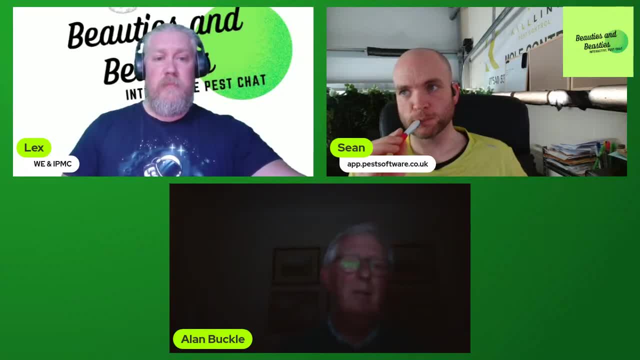 there are other rules about the, about them having to be sold in pre-formed temper resistant bait stations and pre-filled and not refillable temple. you know, all these other things were coming down. so what government's saying to us is: look, we've got this, we're going to bring all these changes. 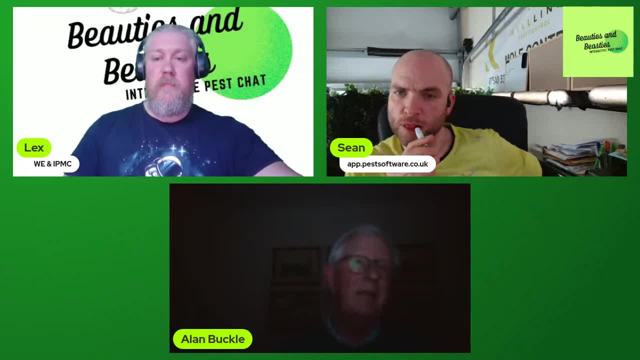 um, and we don't think, or they or they don't think. i think they still don't think that, no matter what your folks say about how badly these products are used by the general public, that that is a significant, a major contributor to the residues that we find all over the uk in almost everything. 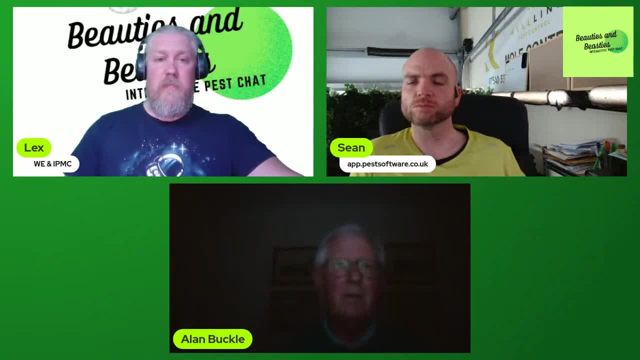 that flies and walks and swims and knows what else. um, there's just one other thing to say. crew has always, um, suffered really from not knowing who uses the most rodenticide. we can't hold any information about sales volumes um, use volumes um, because, um, it's, it's. 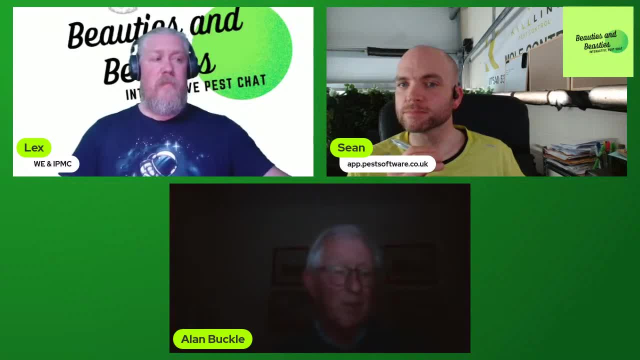 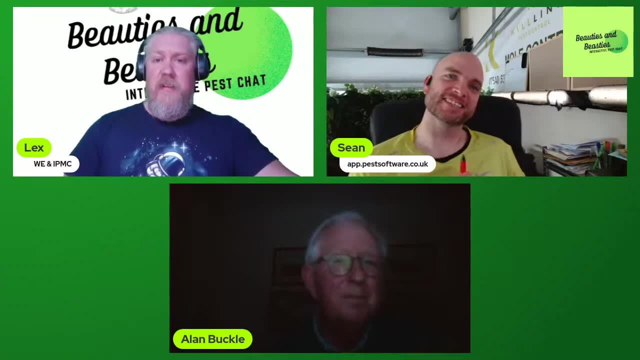 anti-competitive for us to to share that information. sorry, i'm just gonna have a glass of water. of water, guys. i was not able to finish my coffee because i had a little bit at the end of this. um, i actually brought up the concept of uh when i was at a uh m d meeting many, many years ago to try. 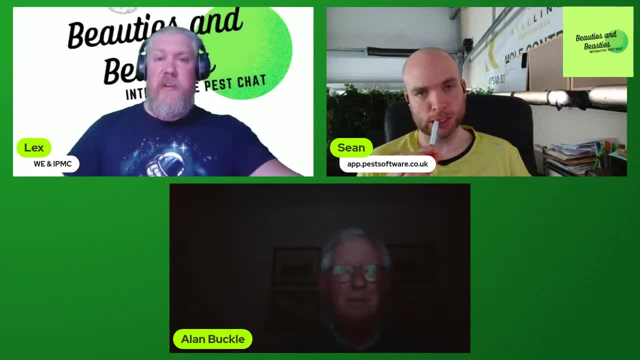 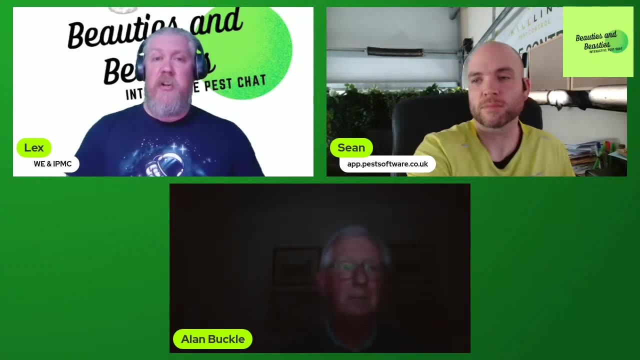 and pull all of the manufacturing distributors there. um, volume of sales are different: rodenticide by postcode, no names, just by postcode and almost unanimously, all of the manufacturers and contributors that distributors said, no, absolutely not going to give you my data on how much i sell to. you know these areas and i think, um, it sounds like alan, you, even in crew, you've come up against. 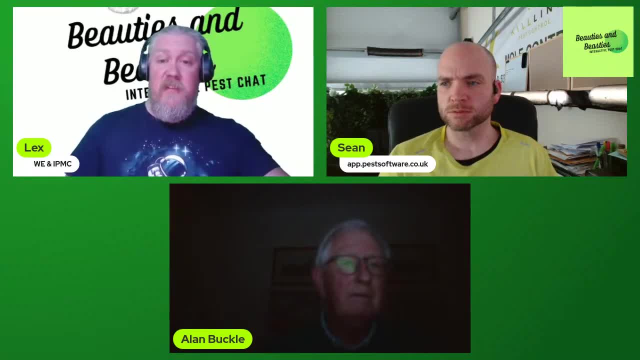 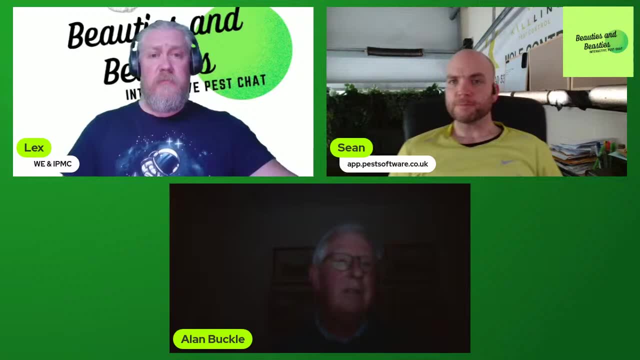 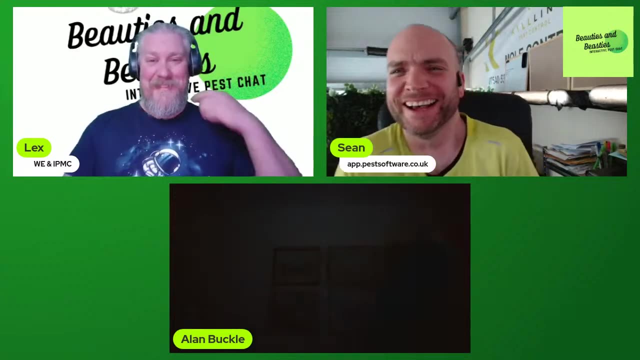 very much the same roadblocks, as nobody wants to share that data because it's considered to be commercially sensitive. um, information, yes, um, i'll say. i'll say just one, one more thing, but i'll go and switch my light on. i'm disappearing into the dark here. hold on i i, to be fair, i had. 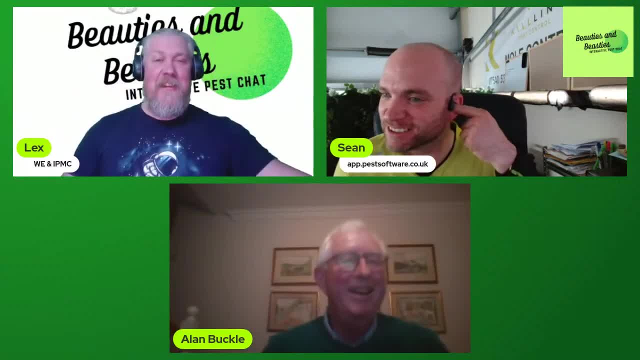 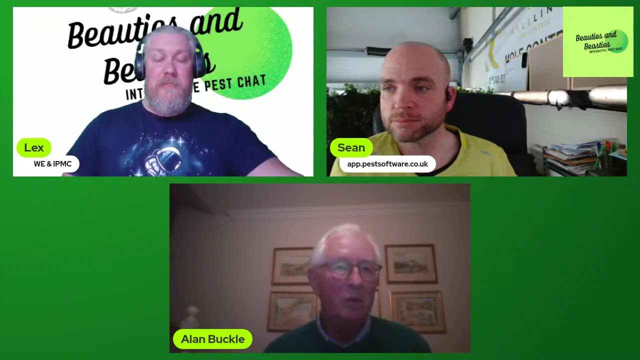 noticed that, slowly but surely, you were receding into ether. yeah, like um. so the, the stewardship regime, is under government review and it's it's in its third year of review. um, and still um. they haven't completed that review, but um, some while ago they decided to um, set up four new government. 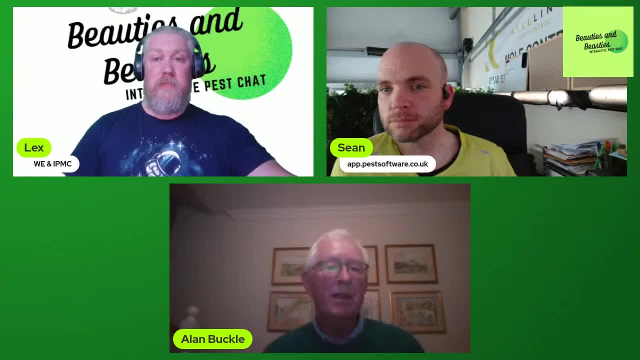 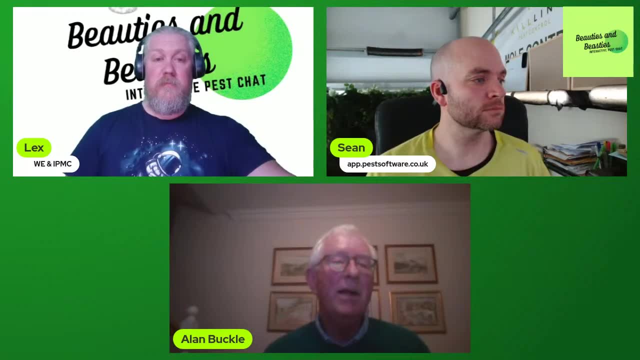 subgroups to look at different aspects of the stewardship ratio regime. one of them was to get to the bottom of this problem of knowing how much of these active substances are being used and who's using them and where they're going. so there is um work underway. 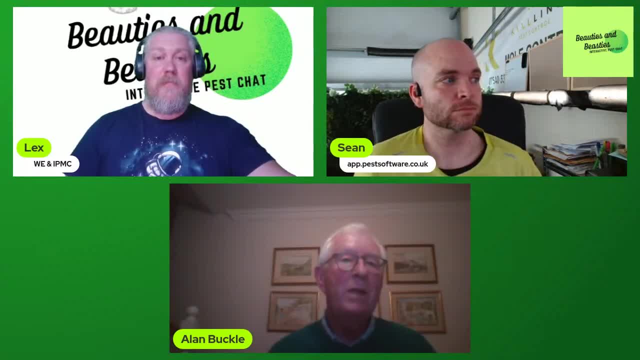 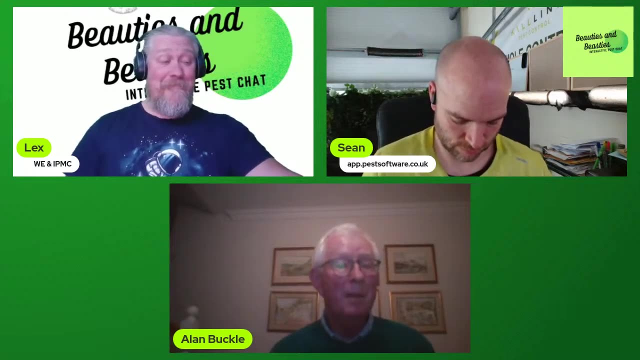 um driven by the government um where they will ask formally for this information form. industry and the, the crew on crew side, all the crew manufacturers- said, yeah, you write to us, you ask us for that information, we will provide it. um promise us that you won't share it with anybody. 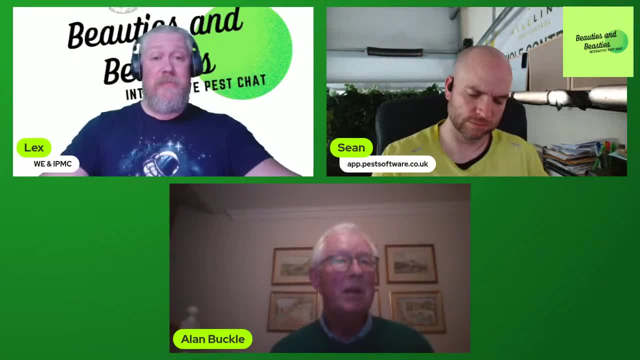 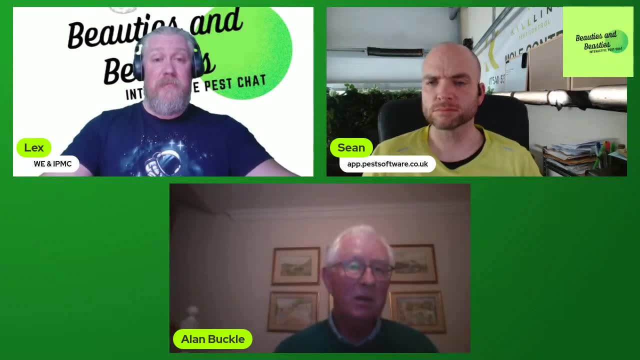 and at least tell us how you're going to use that information. but it's, it's useful, it's important information so that we can try to work out where these residues are are coming from. are they coming from general public use? are they coming from on-farm use? are they coming you? 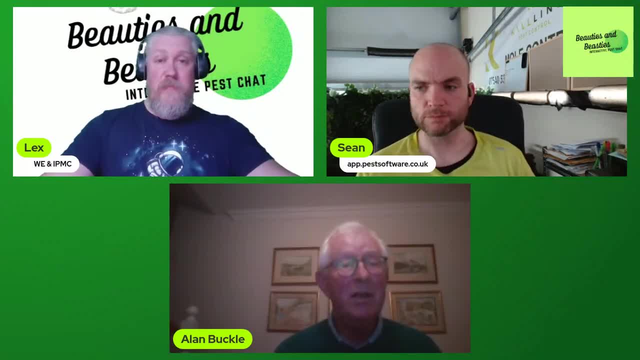 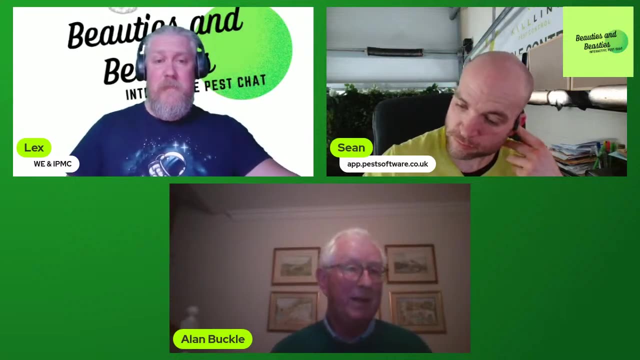 know we, we need that information and what i think is changes in the in the residues in barnhouse we've seen a big increase in bradifer and a decrease in bromodon and diphenicum and we don't really know. i mean, we can guess some of the reason why that might be. 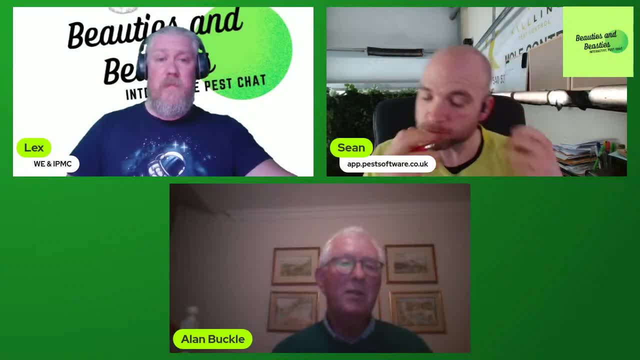 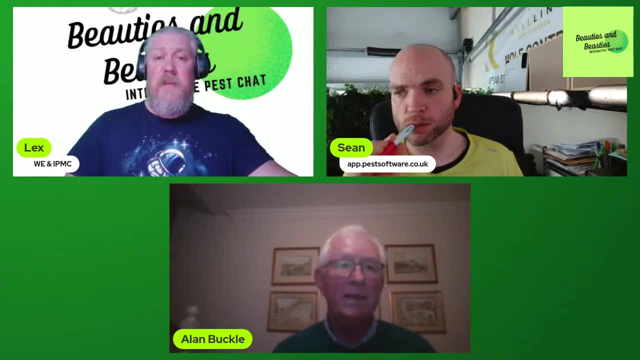 but, um, this government subgroup wants to understand about the volumes of active substances um going into the market and hopefully we will find that, find that out. so if i need to be back with it, sorry, sean, i'm just gonna- you go, you go, you go. yeah, you're going. this leads me back to a 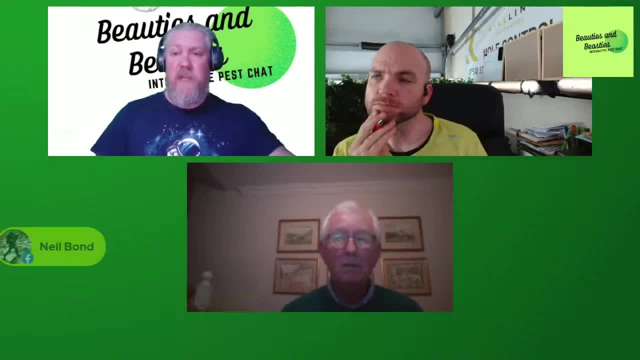 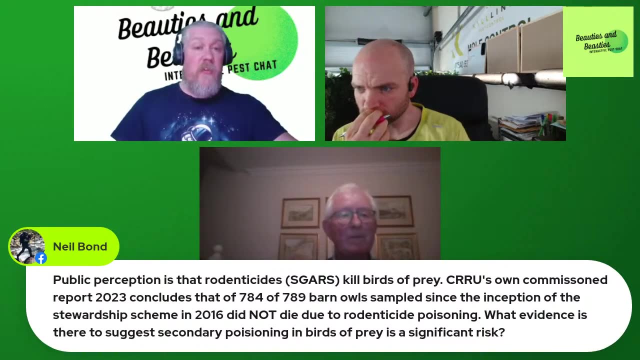 question that was asked very early on by by neil- i think this is the perfect time to bring it up- which was, um- and this is from, i think, um, the the crew, um, the crew paper that you guys put out uh, every couple of years, the update, uh, the 2023 report concluded that 784 birds out of 789. 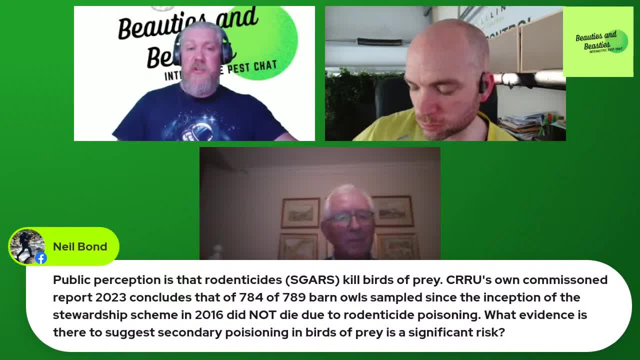 are now, specifically, um that have been sampled since the inception of 2016, did not die due to redenticide poisoning. so therefore, and it does beg of the question, which is actually, how much risk is there to wildlife, to things like birds of prey, to buzzards? 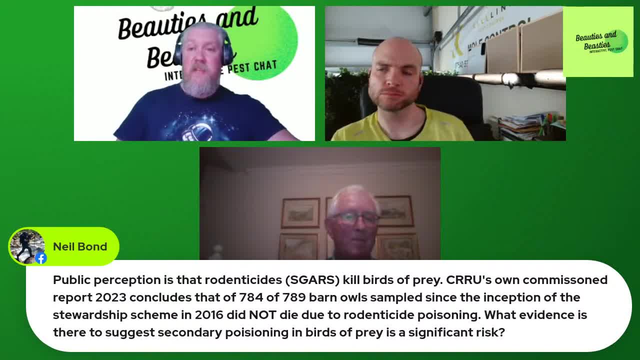 to kites, to barn owls, from these, uh, it seems like- and again i'm playing devil's advocate here because i want to have a conversation around this- but it feels very much like a storm in a teacup. we're finding some residues, but they're not necessarily ever approaching a level where 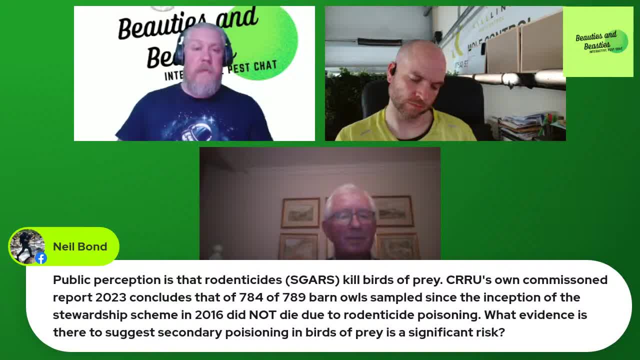 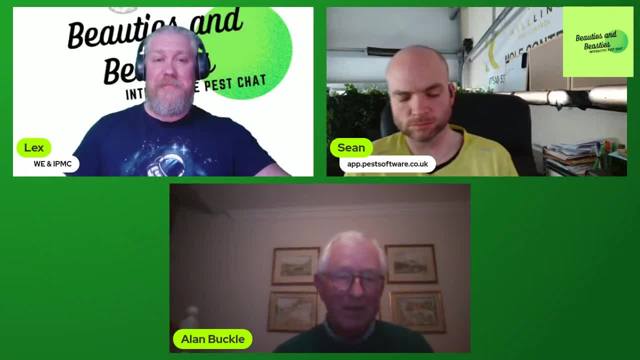 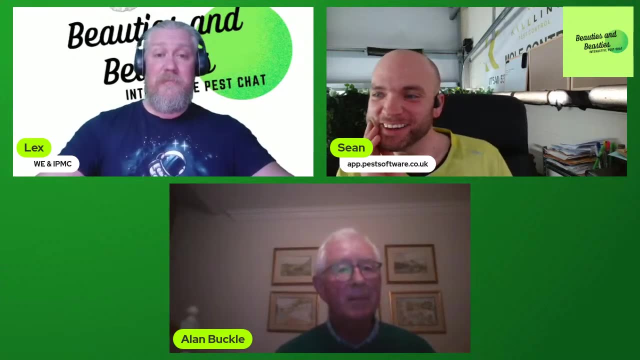 they could consider to be dangerous to the wildlife. so what's your thoughts on that, alan? well, i wrote, i wrote those words about the 780, 84 and seven and and so, and i, i did the the arithmetic by going through every one of the seven years of reports to to add them all together. 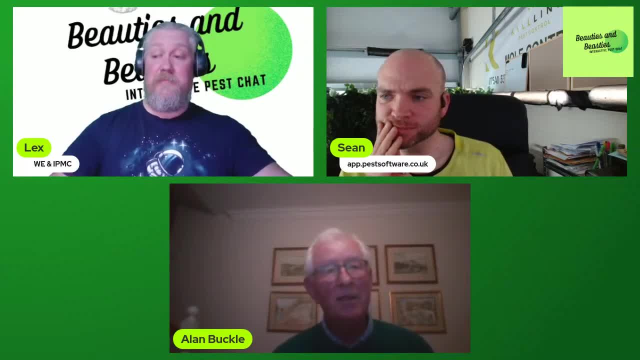 so we could put that piece of information out and i think it's fairly important, interesting information. um, it's an incredibly difficult and complicated thing to to get into, alex. um, and you know i i don't want to sort of escape the question by saying, oh, it's all about the birds and the 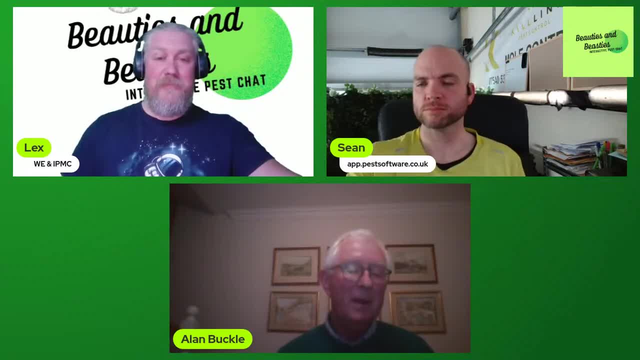 birds and the policy and the, the, the oligarchy, and just to maybe lay a line and you know, just to put it at least a bit more, into what's going on in other countries and and the, the politics of what's happening in europe and in many places and in many other countries. but 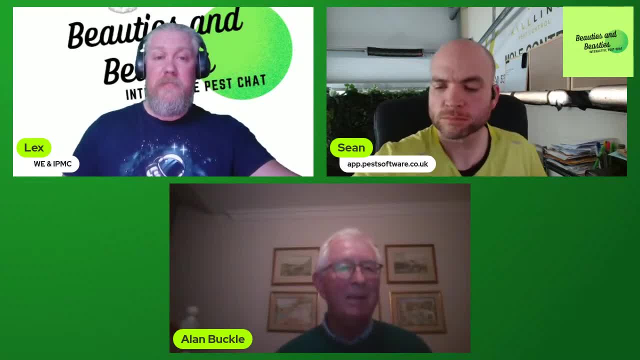 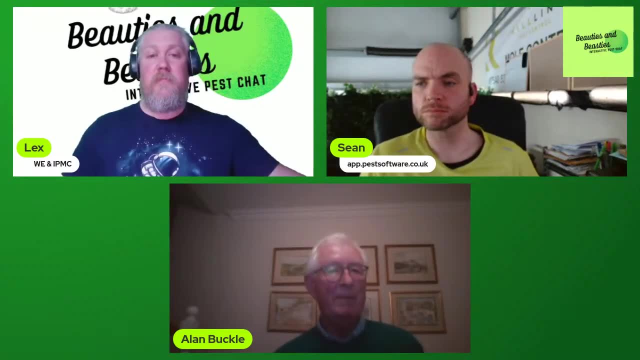 it can be a journey and it can be a long journey, but i do want to share with you that i do think the any individual is going to be eligible to do something that you have to do for them, because, again, it's an either. you know, and i think that you know, those are things that we can all do. 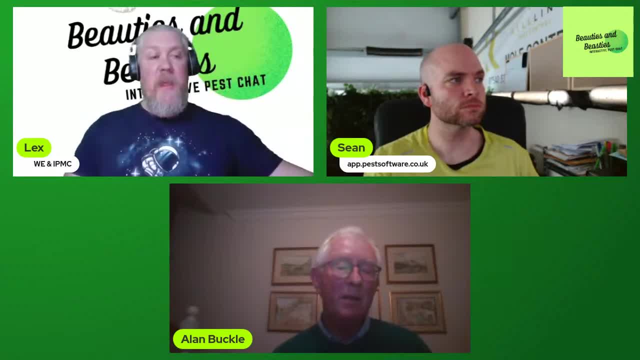 but then there's definitely someone who's going to have to do something where you can access this, because it's a very important piece of information and we can all do a lot of things at a time and we're candidate for substitution label. all of the regulators they see that their only job is to 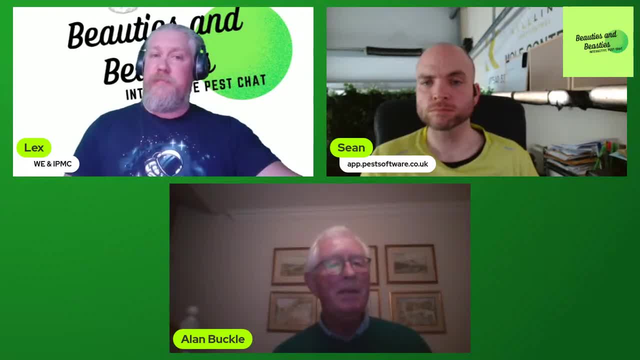 remove those products from the market. Now many of these many substances become candidates for substitution because they tick something which is called an exclusion criterion. And they just need to tick the exclusion criteria and they become candidates for substitution. All of these escars. 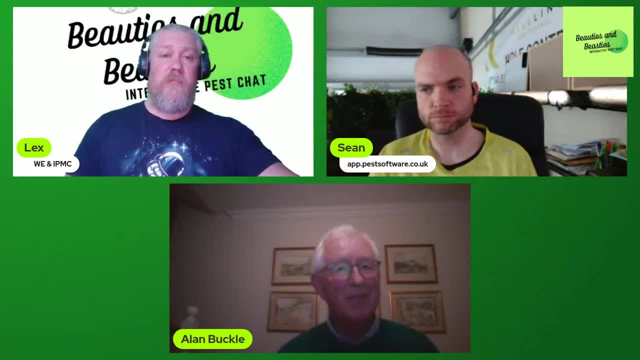 tick three. So there are three different reasons why all the regulators hate these products, And there are three reasons different that these should not be on the market. So this rings every regulatory alarm bell in the world. So that's where we start Now. 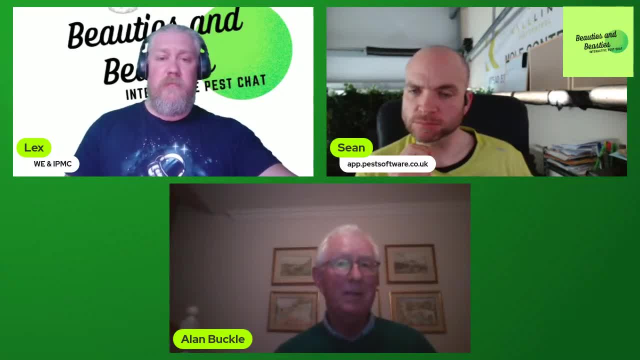 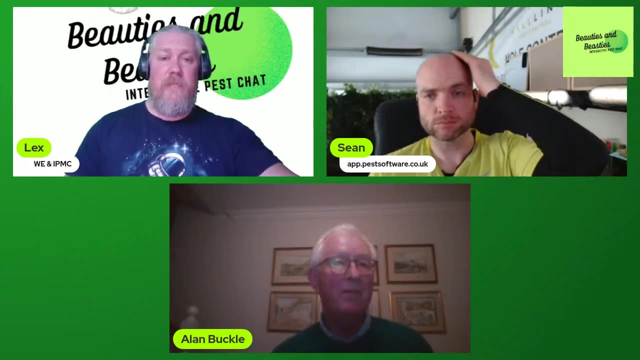 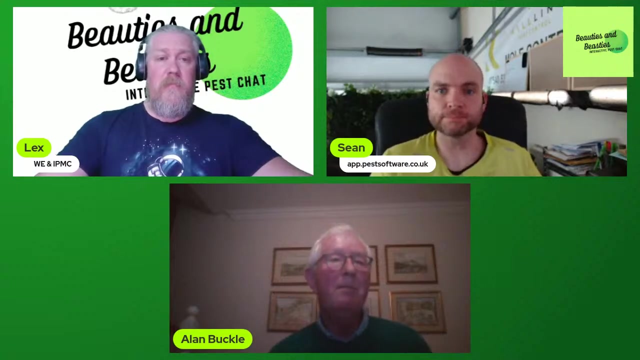 we know these things kill things because we're finding they're dead the whole time. That's a complicated thing because we have this wildlife incident investigation scheme that tells us hundreds of birds are killed by these things every year. But many of those are criminally and purposefully exposed and people 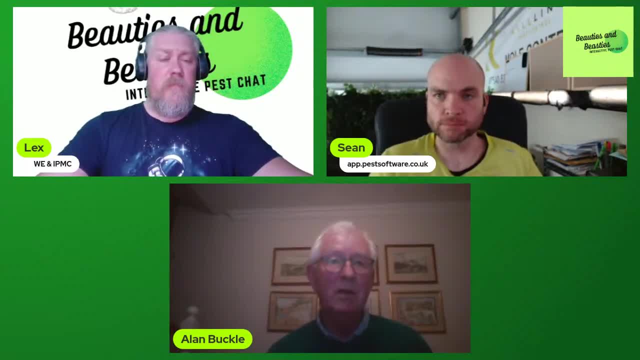 do bad things and birds get killed. Now I put out that barn owl information. To go beside that barn owl information, if you go into the website of the British Trust for Ornithology and look at what the UK barn owl population is doing, I worked on the one and only entire UK barn owl. 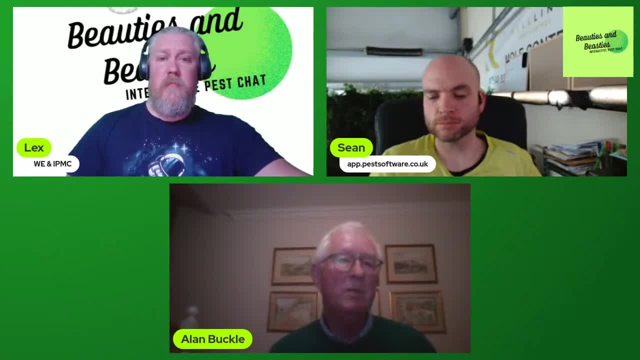 population measurement. It was called Project Barn Owl. It was done in the mid-90s And the answer was that we had 4,000 pairs of barn owls. We now think there's about 12 or 14,000 pairs of barn owls. So the population has increased almost three-fold since the 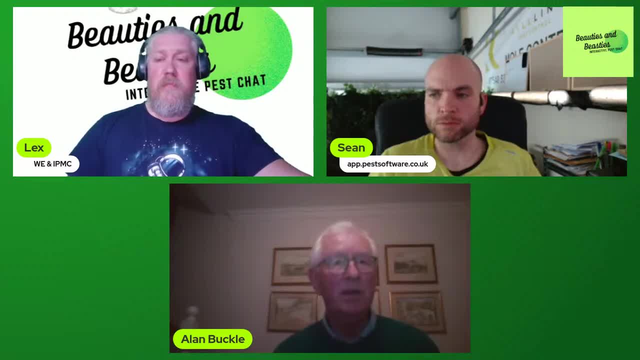 only population estimate was done right through a period of incredibly intensive and growing use of second generation anticoagulants. So we've got good news that we don't think this kills very many barn owls. We've got good news that the population is. 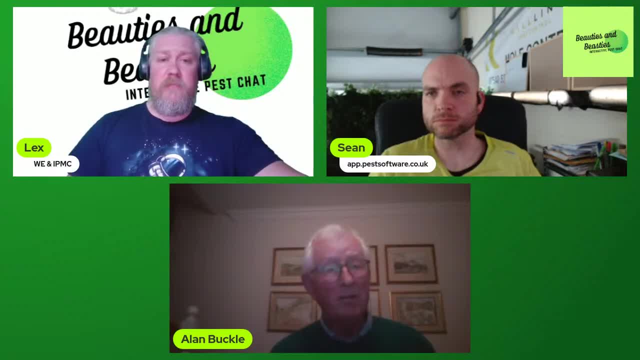 increasing, And that's true of red, of red kites and buzzards also, and these are the three most exposed birds, bird species, all their populations are increasing. so those are points that I try to make whenever I write these, these reports. in some of the reports I 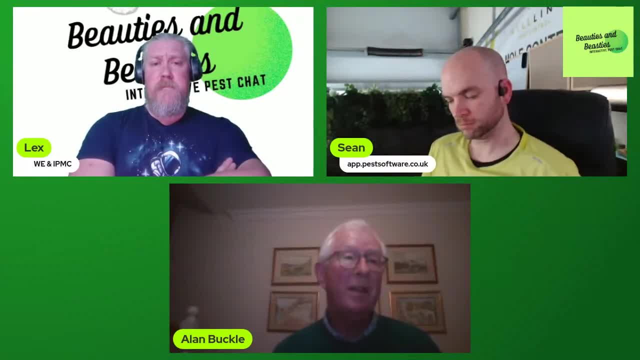 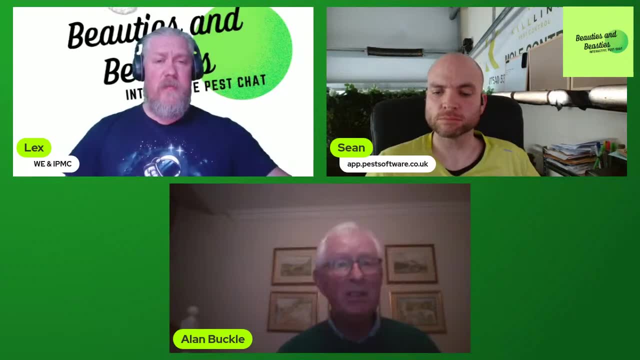 actually put the population graphics at the back of the report so people can see of buzzard over the. you in the last 30 years use ruspos and buzzards from a rare bird found in the far west of to something we see all day all over the. 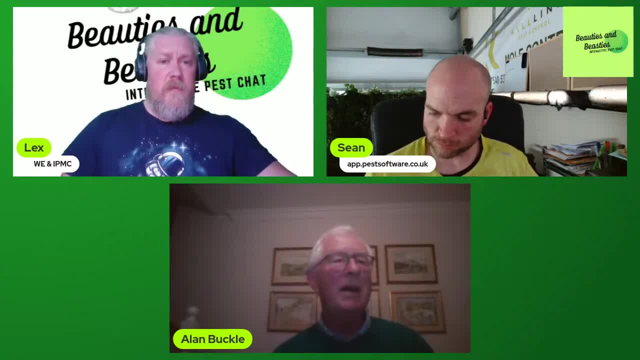 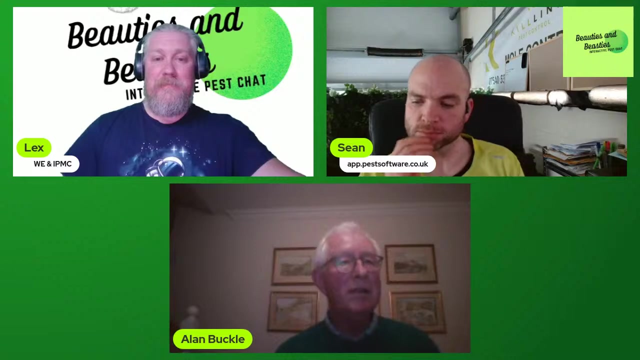 whole of the UK. so I think, does it matter? and the issue is, it matters because of these regulatory conditions, as a reason why a várias? well, come on, we lost Alan. no, I'm not calling up, it's coming, so I'm just coming to the very last thing and when I say, okay, we've got 90%. 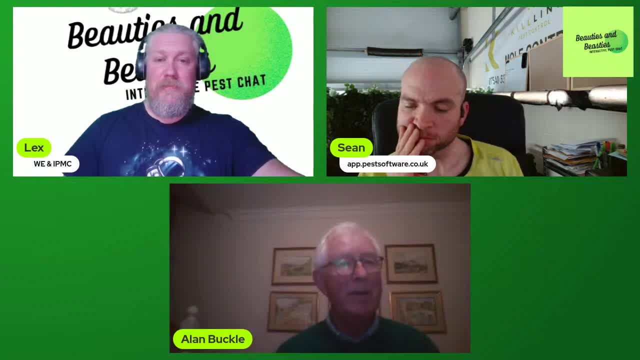 of barn owls carrying very low residues, but we only kill 5 out of 800. what comes back to me immediately is that we just don't know if those low residues are issues that we really want to answer now. I think I probably. I think this is a 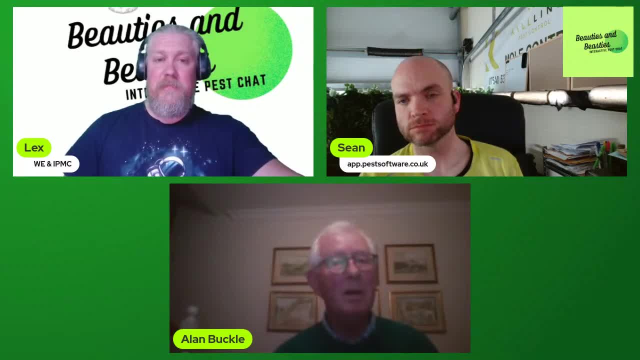 bit of a more today. it seems to me it's a bit more of a surprise, so I guess I'll are having any sublethal effects on survival, on breathing, on behavior, on predatory behavior and so on. We know they're there, We actually don't want them to be there And we've been set. 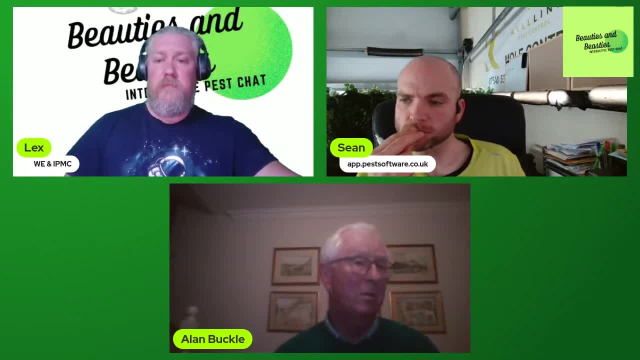 the task of trying to stop it happening. So that's the story. And I might tell you a slightly different story in two weeks' time, when I'm not the chair of crew anymore. but that's the story. I'm sticking with you guys tonight. So one question I have. Go on, Go on. I was about to. 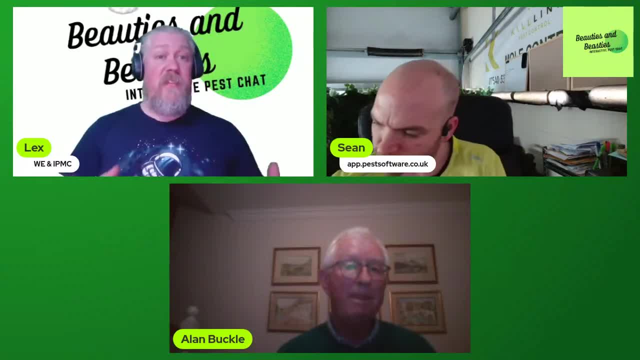 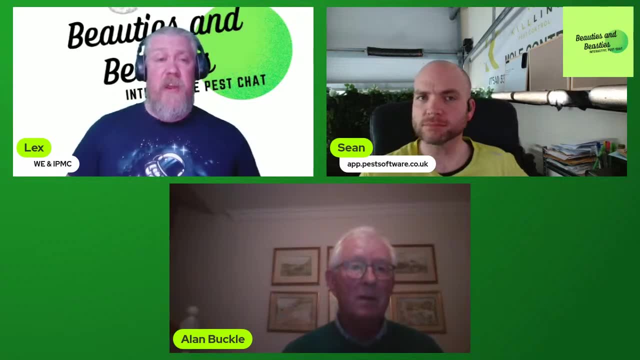 say. there's an interesting bit of statistics that you've just highlighted there, Alan- I don't think anyone's really picked up on it- which is the number of residues in barn owls is increasing for each barn owl that we take and we take out of that. But theoretically as well, if the population 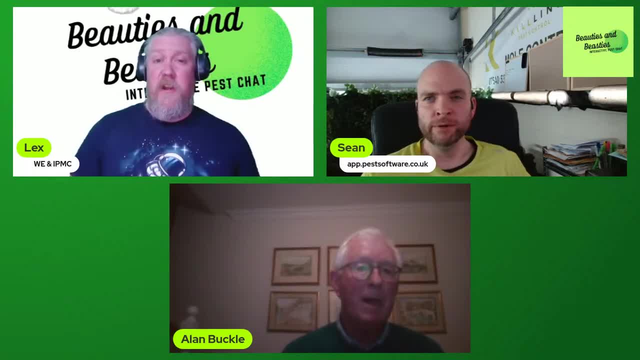 has increased by three to four times the number, then you would expect By dilution, almost by that fact, if the population had increased by three times, the residues should have gone down, Because if that residue is being spread equally across the whole, 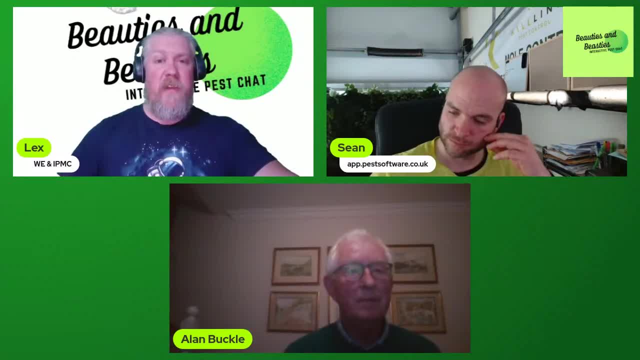 population. if you've got more birds but the same amount of poison out there, then you should have less poison per bird. The fact that we have more birds and a higher level of poison per bird being recovered, to my mind, that is the really worrying thing. That's the startlingly worrying thing. 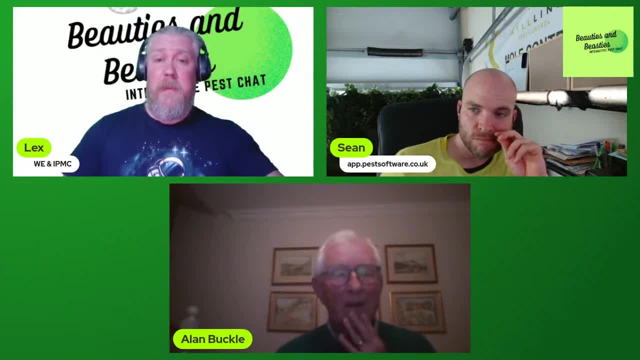 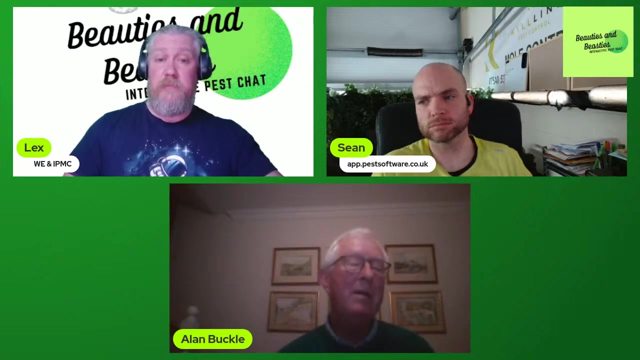 Well, let me just put one thing right there, Alex: The concentrations of residues are not going up. They are virtually flat and have been flat all the way through sewer dip. Now, we did, to begin with, take that as a plus, Because when diphthylone, flocumafen and brodiphyllum were finally freed up, 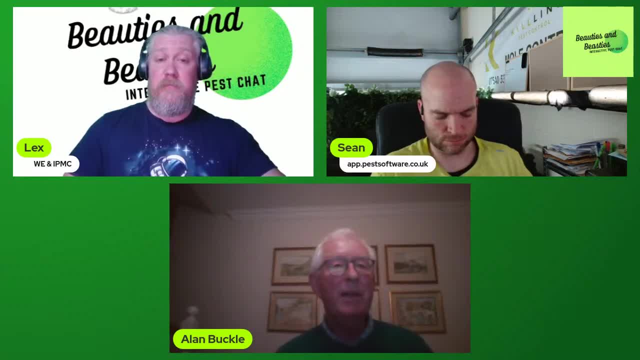 to go Yeah in and around buildings instead of being restricted to indoors only, which meant they could not be used for rat control everybody When we managed to get the regulator to make that change so that we could use these potent resistant breakers for resistance management in rat control. 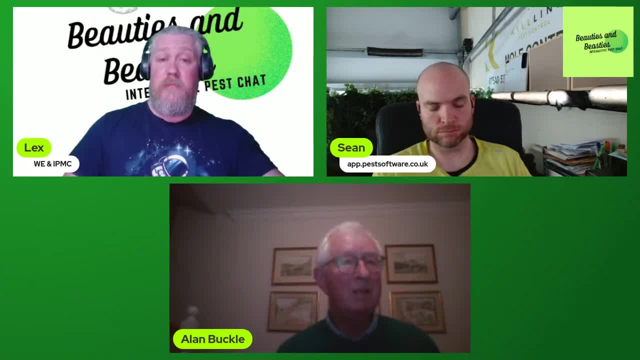 in the UK everyone was terrified that when that happened there was going to be a wildlife apocalypse And in fact it didn't happen. And for many, many years- five or six years- we got pretty static residues, So there was not a sudden. 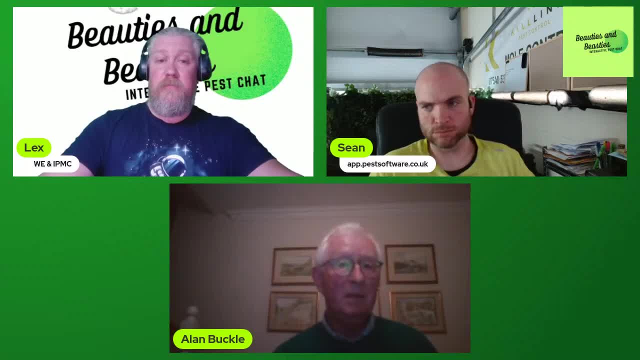 jump. What's been happening lately is, as I was explaining before, that the total concentration of all eschar residues in our barn owl livers is pretty much the same year on year ever since we started stewardship in 2016.. It's flat. 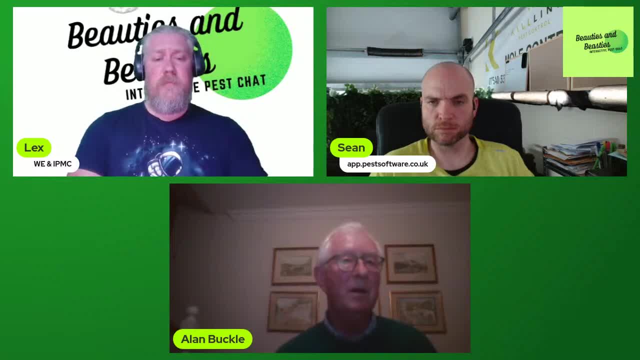 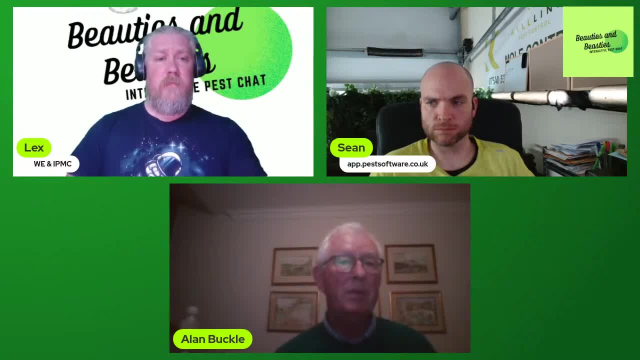 total eschar load per barn owl is pretty much the same. Now, when you said about the dilution question, I'm going to have to try and get my head around that a bit. What I would say is: I think you could probably double and treble the barn owl population in this. 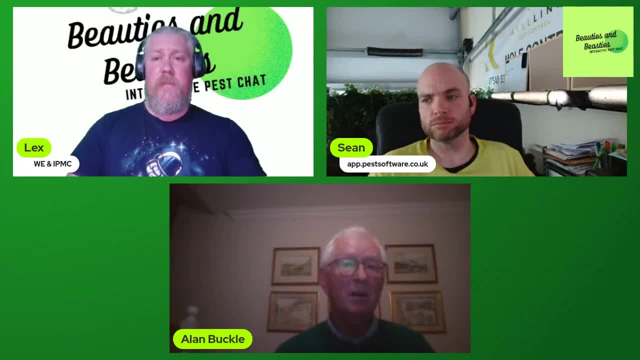 country again and there'd still be plenty of eschar residues. I think that it's worth using the additional amount of eschar. It's quite a lot to go around to contaminate the lot of them, So I don't get the point about the dilution at all. 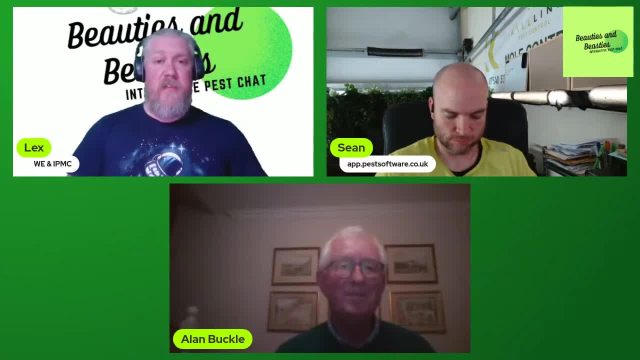 The point being that if you know, if you have 10 birds and they all have a static residue in them, then if you have 20 birds and people are using poisons, you know. the same way. then if you have 20 birds, then theoretically, the concentration or the number of birds that should have it should be on the lower side of the barn owl population. 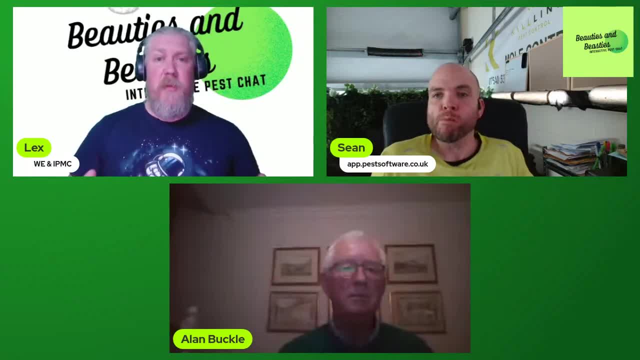 Thank you, Thank you be less because you've got double the number of host birds but the same amount of residues going out into into the wildlife. the fact that you've doubled the number of birds and you haven't half the number of birds that are detectable or half the number of uh residues in there means 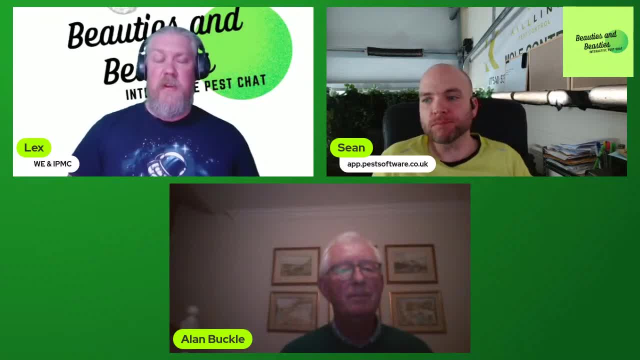 that where you, with more residues, are getting into the the environment to get to the additional 10 birds. um, that was the point i was making with that and um, i, i, yeah, alex, i, i don't, i don't think it works like that. i, i, i just don't go along with that, that, that that thesis at all. um, but barn owls. 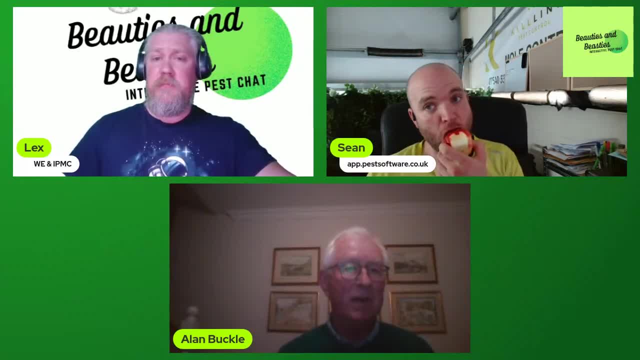 um have territories and and they and they segregate themselves and separate themselves, and so there's, there's, there's, loads of open space where there's no barn owls, and if the barn, our population increases, you don't get two barn owls sitting in the same place. um, they, they. 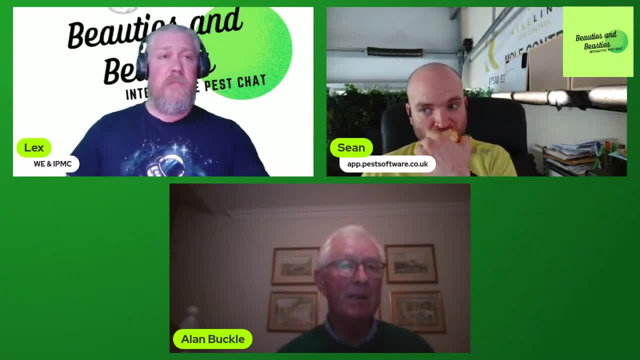 off into another territory and that territory is contaminated in the same way as the, the, the all of the other ones. so i i think i'm pretty sure that, um, if we have more barn owls, it doesn't mean we're going to get less, less residues in the barn owls that we've got. but anyway, let's not let. 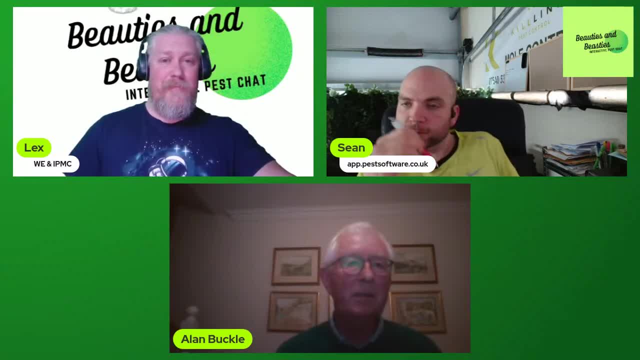 a labor. that point is, it's probably something for a pint at some point. um, could i? could i go back to something you said at the very start? because this is this is my thought process. so please tell us which bits of this are right and which bits of. 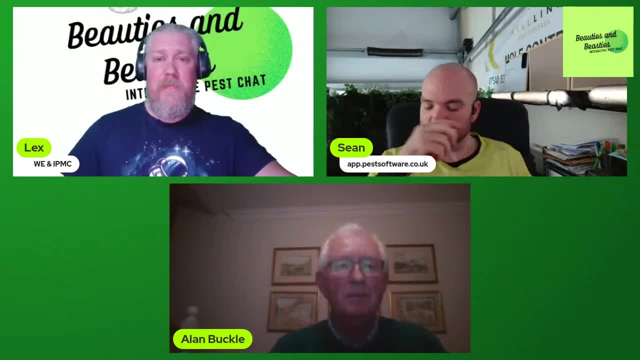 this are wrong. um, when you mentioned the, the summit, you said at the start about politics and satisfying the regulators and managed to placate them in relation to them being candidates for substitution, etc. it feels to a little old, lonely pest controller who's on his own down here that what's actually happening is that there is pressure from the 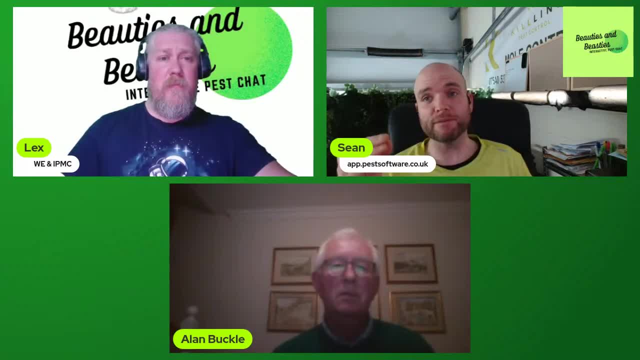 agricultural sector to basically mean to allow their farmers to continue to use poisons, because, fair play on the farmers, they've got that much pressure on them doing so. as you said, when the audit has come in, they've got a million and one things. the pest control is like that much of their. 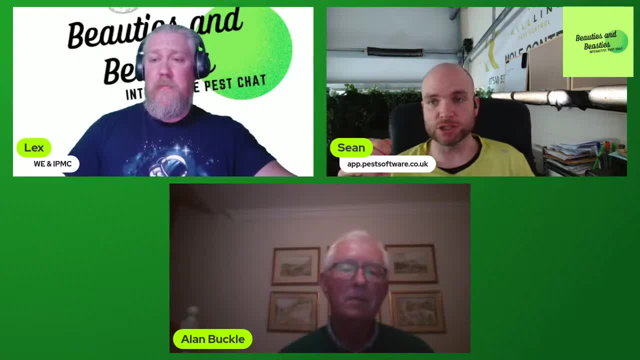 day, isn't it? and they do. they're already strapped for cash because they're just getting squeezed all the time, so they don't want to pay more. we get it, but it feels like that crew is definitely getting a lot of pressure from the agricultural sector in order to, um, make sure that they can continue to. 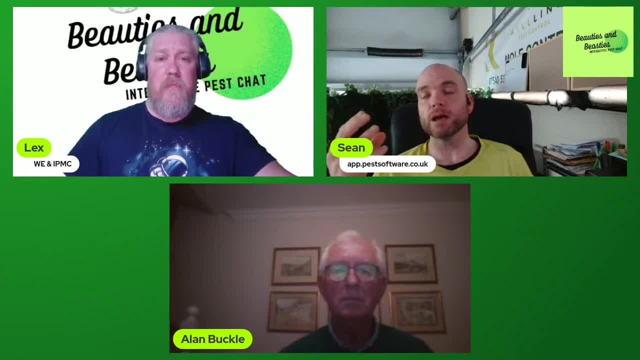 use poisons and through someone who does agricultural work and knows a lot of farmers, um, when you speak to them, they haven't changed what they're doing, they just do the their 80 quid course and they carry on um like the broad, difficult, broad difficult being in and around. 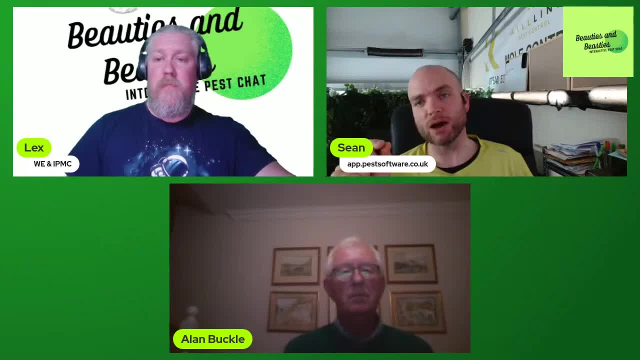 buildings. i'm sure that that change is probably the reason why we now find lots of issues. i'm sorry about that, but so it's just that i'm saying we're not just thinking about the nature of agriculture, because there's a lot of companies and there's a lot of job opportunities. 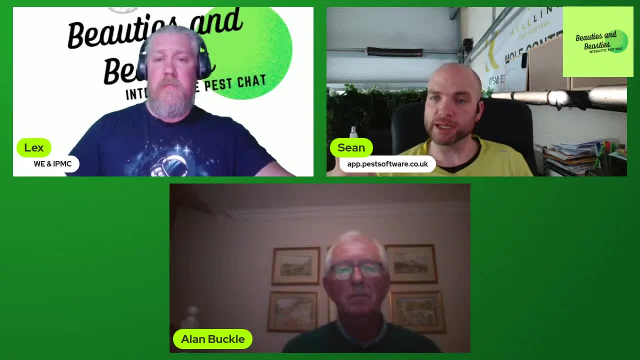 around agriculture and there's lots of procedures and things to be done about it and, of course, it's got to work at the right time and, yes, there are jobs. but i think that we need to start thinking about these cases in order to to deal with them and to think about the important. 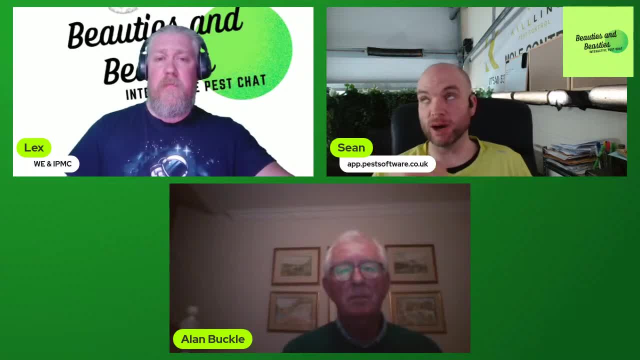 and important role that you have to play in the agriculture industry and why we have to take the risk, and we need to take the risk for us to go out there and do the right thing, and i suppose that's the point. i was just at the beginning of the video and i think an important point is that you know, as we don't have to. 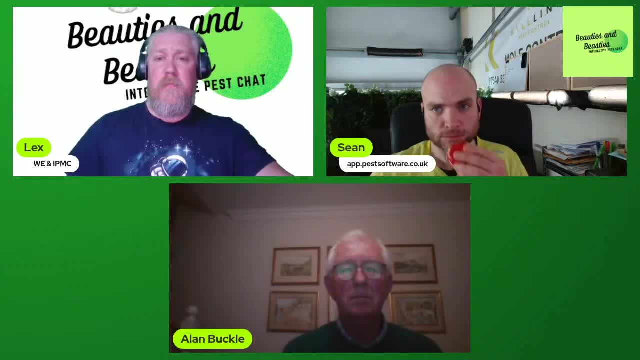 agricultural sector, if that makes sense. when, when you say you, you take the brunt, Sean, what, what, exactly what? what do you mean? you know, I don't quite know how to respond to that. yeah right, so so as a professional pest controller, I feel like rodenticides turning up in barn owls. 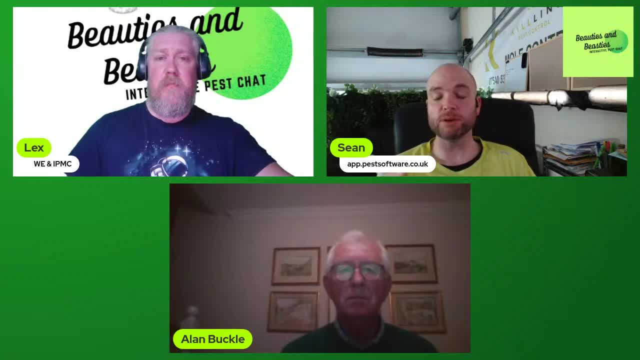 means that the fingers get pointed at us because people go: oh, pest controllers use rodenticides, so when they turn it up, it's very much. it feels like the public perception is against us. they don't stand there and think our farmers by. you know, there's 30. there's 30 times more farmers. 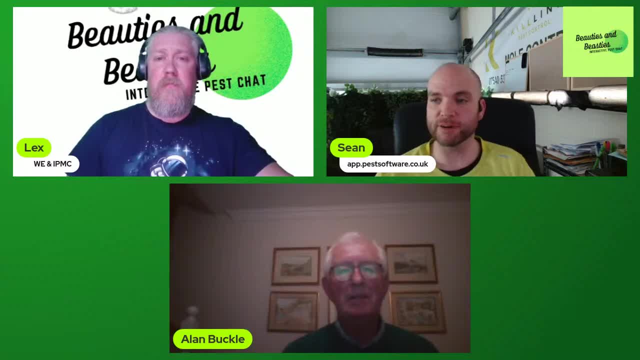 and there is pest controllers and they're all banging out poison like it's going out of fashion, as I've been in the farm shops and we've seen them, so I feel like that whenever there is a problem with rodenticides, it's pointed at, you know, the fingers firmly pointed at the professionals. 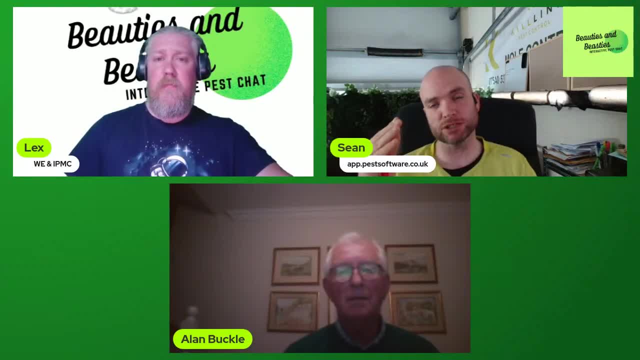 because the vast majority of people outside of this industry don't think of gamekeepers and farmers as professional users and just say: there's us. and then I stand, I think like, and this is quite an interesting point, isn't it? what is the role of crew? was crew, was crew's role to reduce residuals? 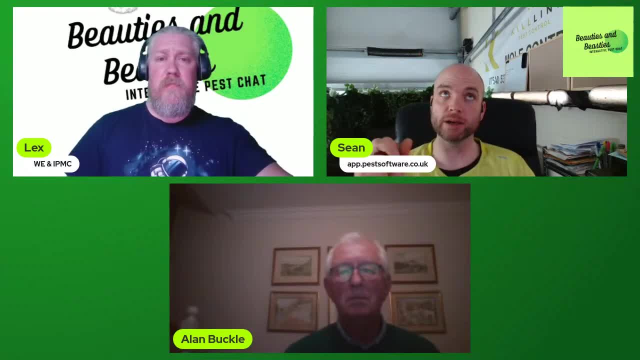 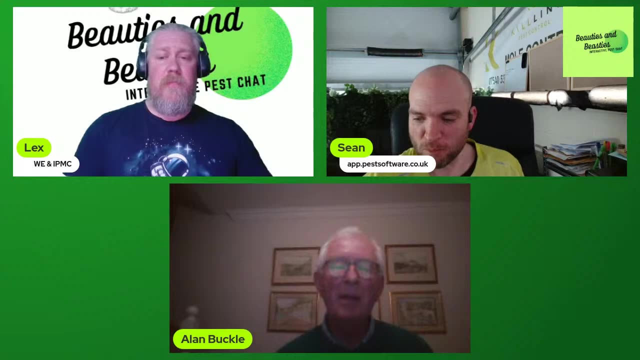 or was it to keep rodenticides as an open, uh, available to us to all professional users to use? okay, so, Sean, um you, you've, you've entered sort of two points. yeah, yeah, slightly different things there. they're both incredibly important. I can't keep one thing in my head for very long, so keeping 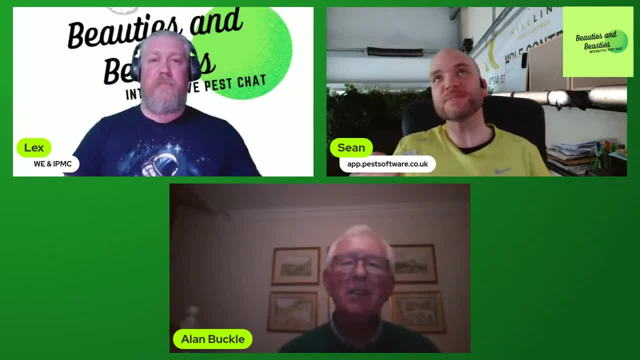 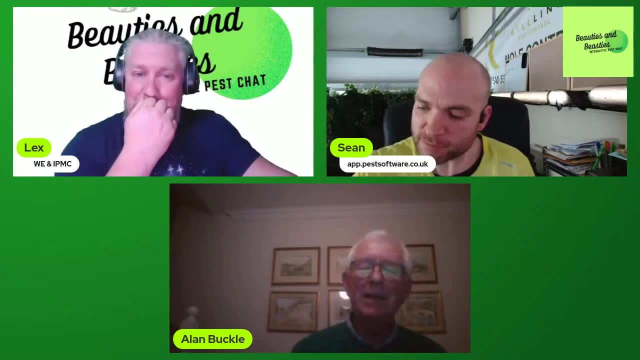 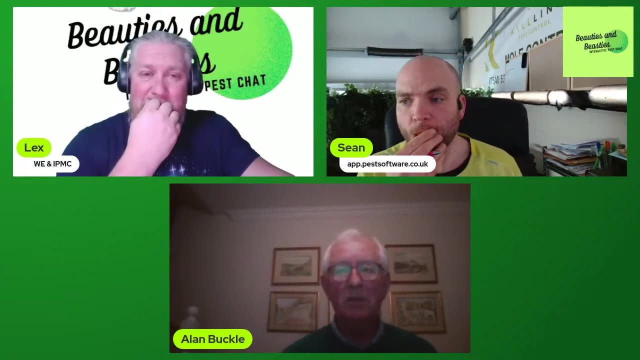 two keeping two things, yeah. so the first thing is: it's true, it's true, yes, I get it, so it's. let me answer them. let me answer the finger pointing one. first of all. you were saying: we get, we, as professional pest controllers, get the finger pointed at us. 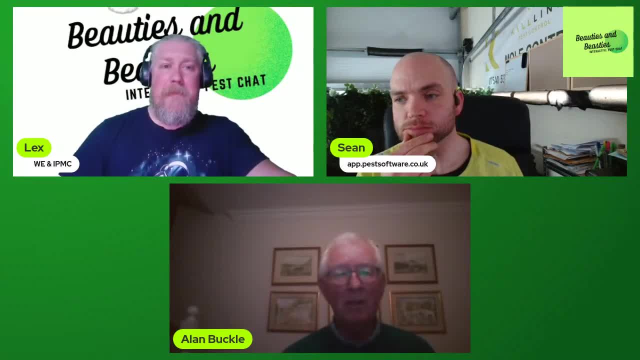 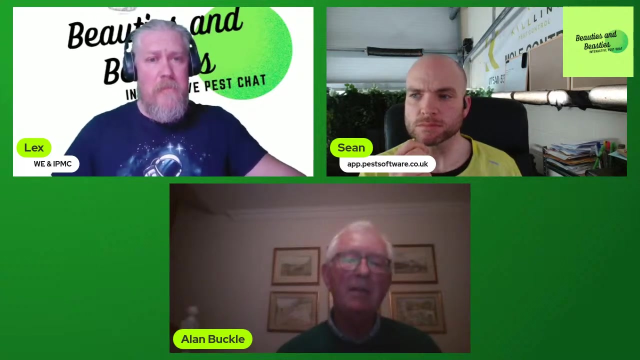 i. i could only try to assure you that is absolutely, absolutely not from from a crew point of view, nor is it the case from the regulatory point of view when i speak to the people inside hse. um, so these um every two or three years when we spoke at test sex. 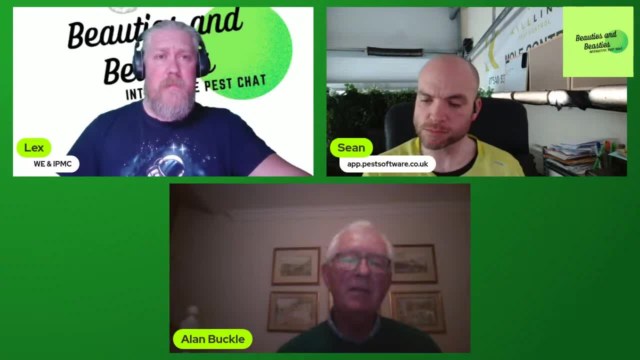 um, they're called caps- knowledge, attitude and practice- and we do these massive surveys and we have some calls of farmers, farmers, farmers- what they know about rodenticides, how they use them, and the industry comes top of the class every single time by a country mile, and we make that clear to the regulators. they see the data and so they think, and i can think. 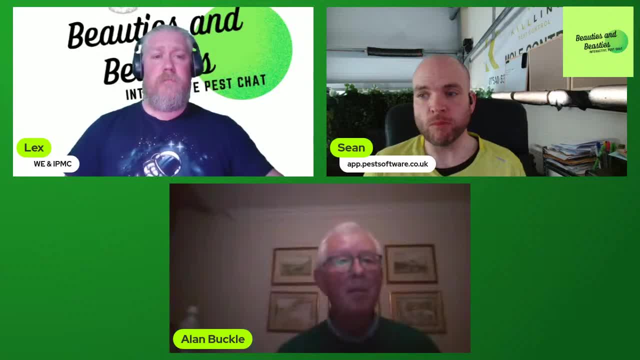 um that you guys um know more about these products, know more about how to how to use them. now, you know i i know there are baddens in in every single sector, but but that data that we publish, um shows that you, you folks, are streets ahead. so, honestly, i don't believe anyone into the finger. 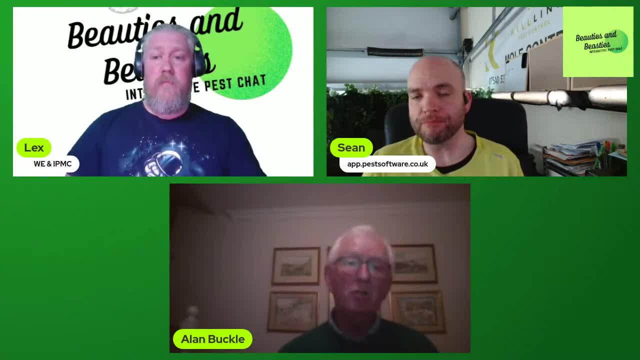 at professional pest control are the opposite. but crew has to work and try to these three sectors- farming, professional pest control and gamekeeping- and if we started to point the finger at anybody in any one of those sectors then we would be in deep trouble. we would, we would. 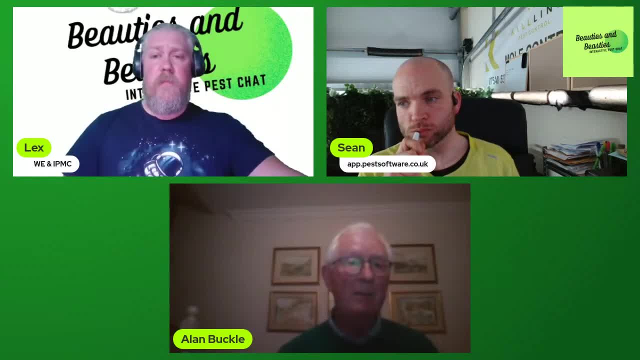 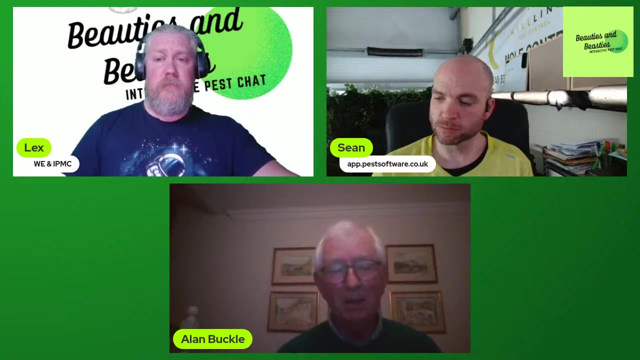 lose friends and influence, and it's absolutely something we try not to do. so we try to point at pretty much um, at no one we- we don't blame anyone for for for this, but we try to work with one to try to reduce these residues. so that's the finger pointing. quite a question now tell me what the 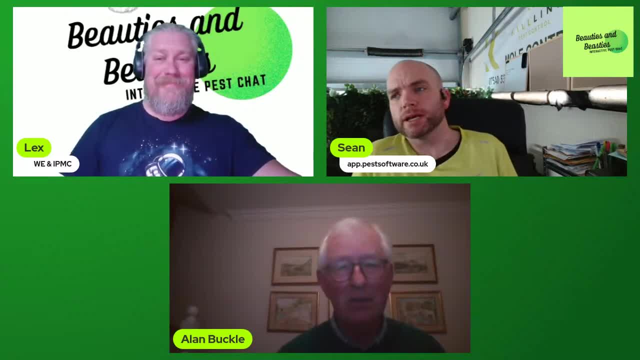 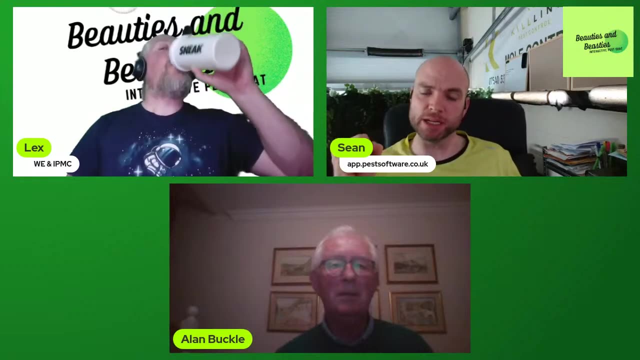 other one was: please, yeah, it was, um, yeah, you know it was. it feels like the agricultural sector, um that the other almost have, have this power, this lobbying power. i don't know if that's the right words to describe it, but it feels like the agricultural sector have this ability to put. 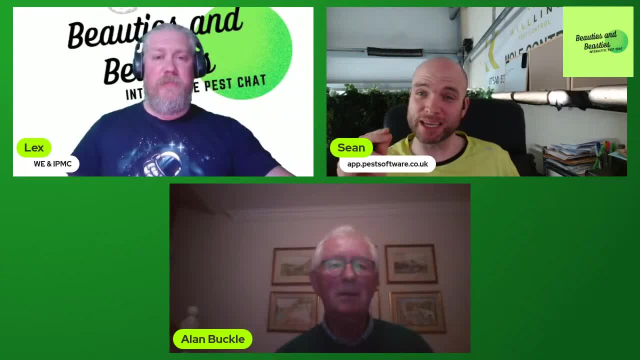 pressure on crew to make sure that they are basically given the least amount of things that they can do possible in order to continue to use it. but i'm going to point the finger- me personally, and this is just my personal beliefs- it feels like it's the agricultural sector. 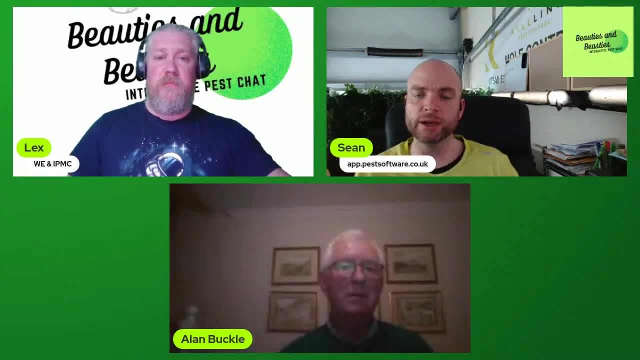 that's causing the residuals within the birds of prey to me. i know other pest controllers disagree, because i never see a barn owl in a council estate. i never see a red kite. i never see a buzzard. they are always on the farmlands. that's where i see them regular and you're right, the numbers have. 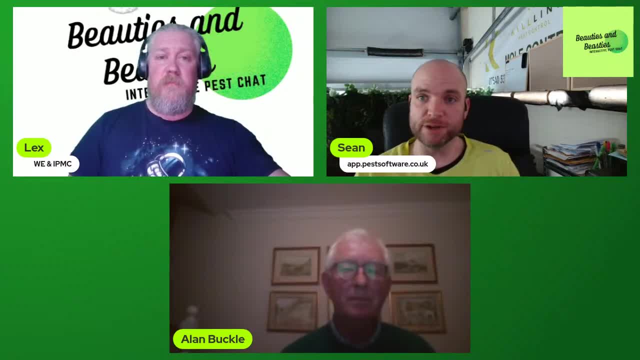 went up astronomically. i see them every day, but they're always around farmland and it just seems like it's. there's this rule and, going back to that, this is how professional pest controllers are supposed to behave. farmers have to do a course every five years, like a however many hours course every five years in. 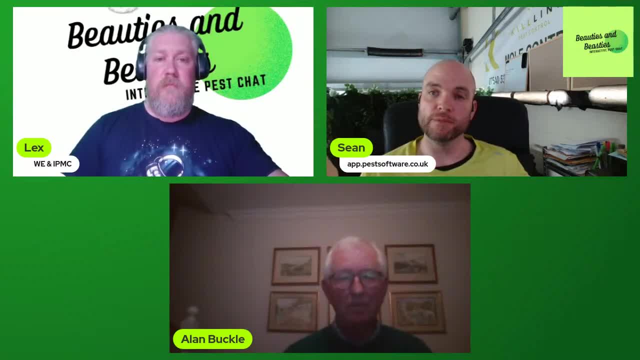 order to be able to do it, and the course that they do, in my experience, doesn't change the way that they behave. they simply do the course and then they go. they revert back to what they've always do: chucking bags, every bale on the first row bales. so that just goes through. you know banging stuff. 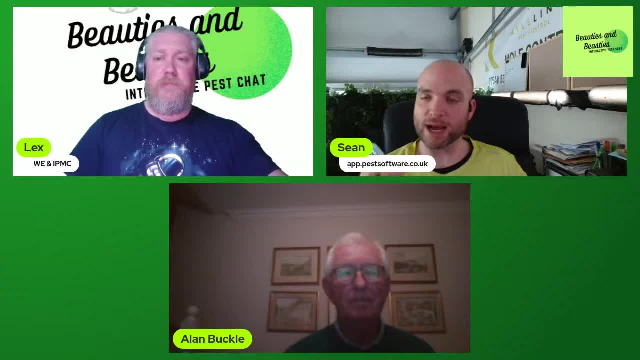 down left, right and center and in fact, when i talk to farmers, i'll speak to them and they'll go: oh yeah, yeah, we're on the single feed stuff now. i'm like: you don't even need it. we don't have resistance up here. i don't use single feeds on farms, i don't. i don't use it, but because it's marketed to them. 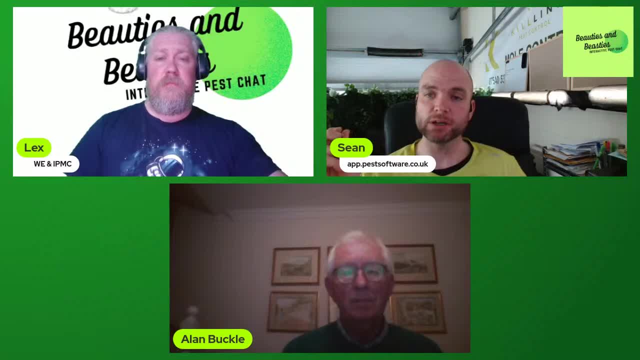 in that way they're like: yeah, so they're. they're walloping out, in my area at least, where it's not needed and they just get this. it feels like they're getting this free sort of kick of the can, and i guess the finger pointing thing is probably just the. 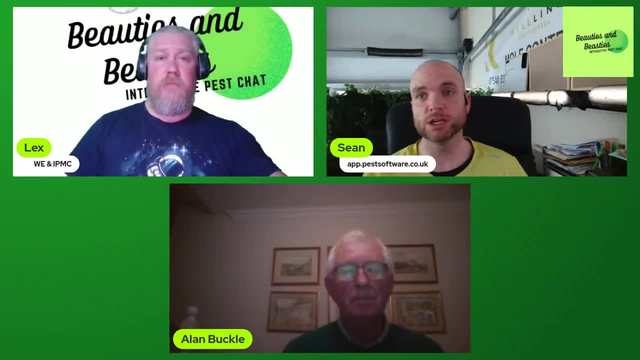 professionalism of profess, of professional pest controllers, who don't want to be in this loop. but farmers don't really care, do they? because they've got that much to do. so it feels like it's the lobbying power that's put on crew in order to be able to continue to sell these products. 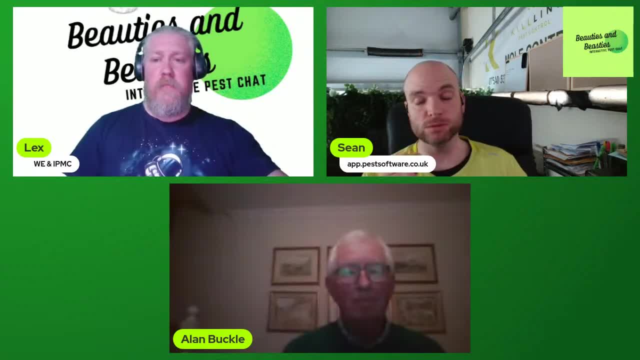 but i do. i do concede. i'd not even concede. i do. i do understand that without crew, we would have lost them, wouldn't we? we wouldn't have them available to us at all. so it is a double-edged sword fight, isn't it? well, the? the other question you asked, sean, is: um, is crew there to keep the? 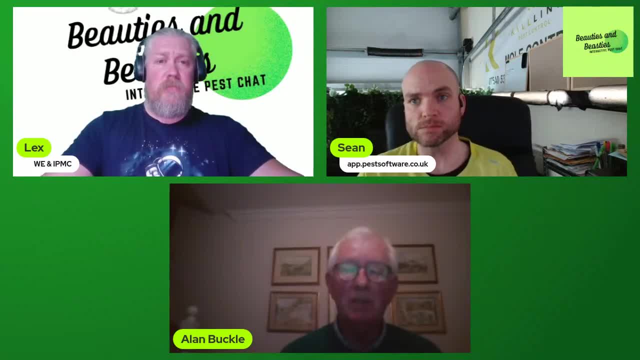 products on the market, or is it there to reduce the residues? um, yeah, and it's, it's, it's definitely both of those things, and i'm not even going to say, right, which is the most important. um, we, we felt, um, and the whole of the industry feels that, um to protect human health and well. 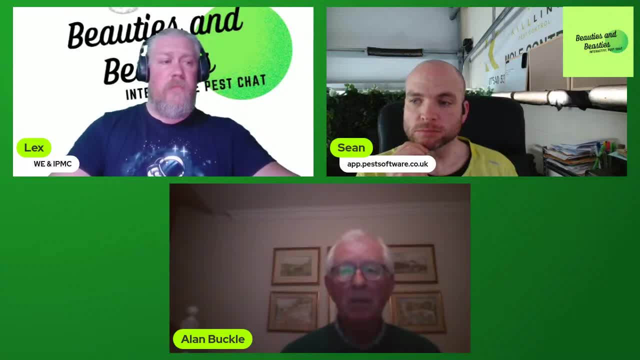 being and animal health. we need these escar products, and and so there was a threat right at the start that we would lose them or that they would be so restricted that they would be all indoors only, and that means that they might be able to be used for mice, but they couldn't be. 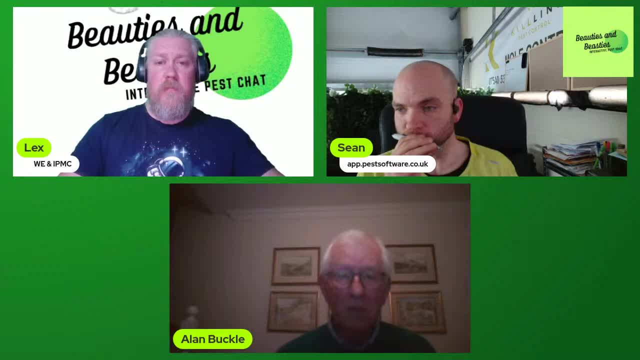 used for rat control in almost all circumstances. so we, we put this scheme together, um, and we satisfied the government that they, they, they, they, and we thought that the scheme was a robust scheme for the stewardship of these things. they set us these environmental targets that were dictated by a single, what they call sentinel. 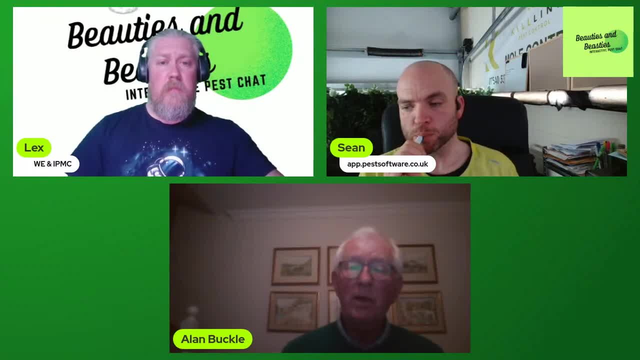 species which is the barn owl, and they told us how we had to bring down year by year residues in barn house and they wanted to see it come down year by year the ground, and we came up with this solution that was kind of attempting to, kind of 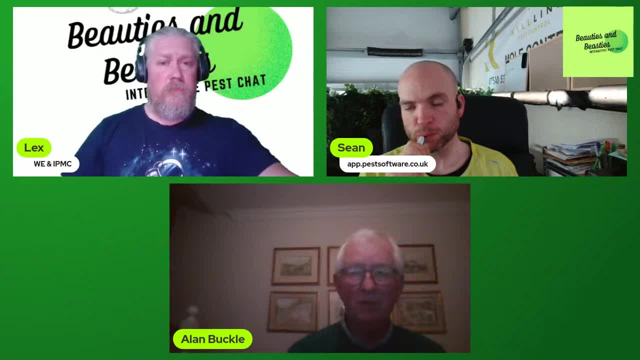 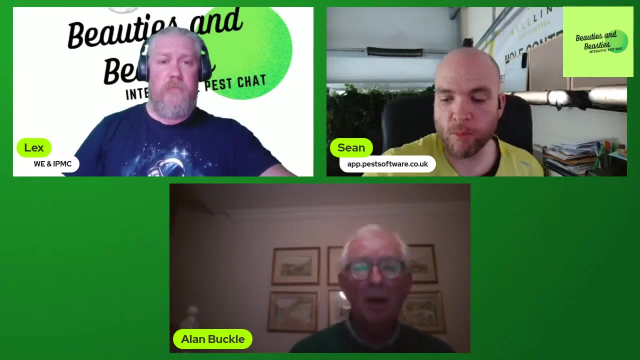 joyful, but a样 what when theатели say that Crisp causity was going down year by year? just started like a miracle? yes, about about six years ago. there was more than one. Keith are Estonians. how should others be told? the story is horrible. 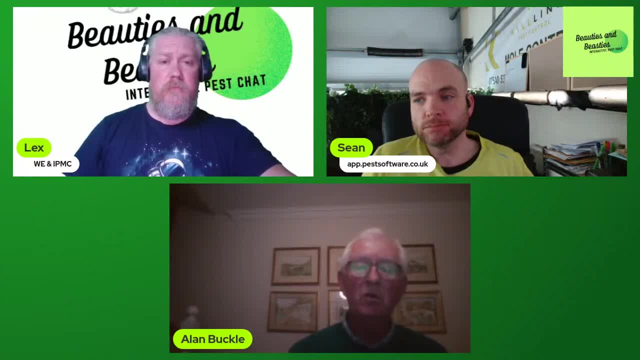 This is absolutely a terribleutan Cause. it's horrible, Yes, Absolutely other This acutely review, review, and so the government regulatory authority, hse, will decide what they want to do now, and it looks as though, um, they will not be able to. we will not be able to show them. 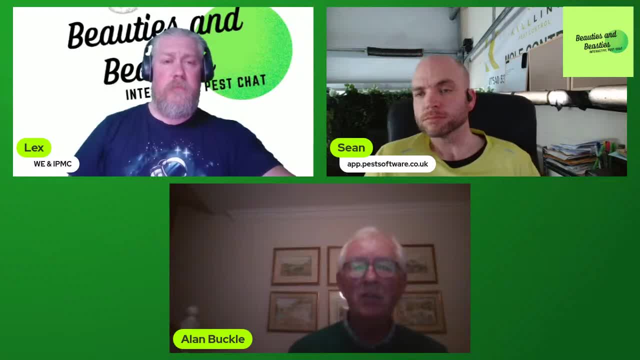 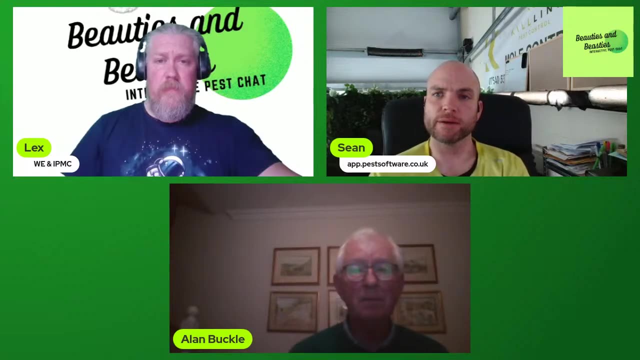 that we've significantly reduced the total residues in our sentinel species after all this work. now, why, do you know? i think, sorry, do you know? i think once pest control has realized that your fight was to keep those products available for us, um, i think there'll be a lot more of them. 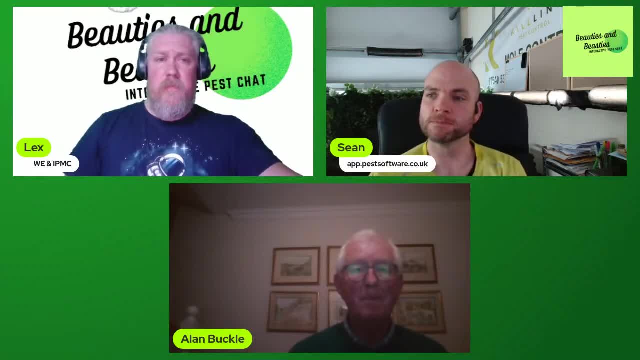 favorable to crew because it felt like it was sort of getting walloped with both- um, with both hands, for want of a better word- that were getting told it was about bringing residuals down, but i think that's the first time i've ever heard anybody say oh, no, no, it's both: we've got to bring residuals down and we want to keep these. 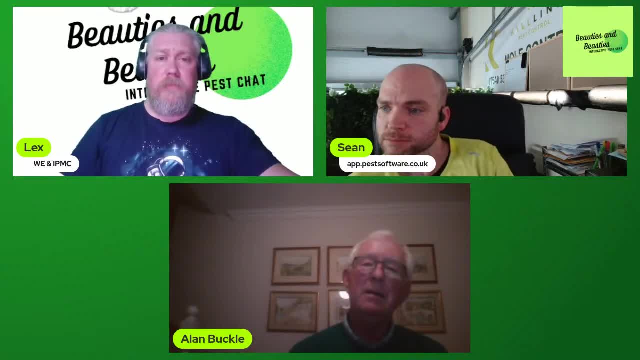 products for you, um, but that's very interesting and i i i'm absolutely sure that that that is the same purpose in the regulatory authority, sean, um, they, they absolutely want to keep these products on the market. they know that there are no good alternatives. if there were, 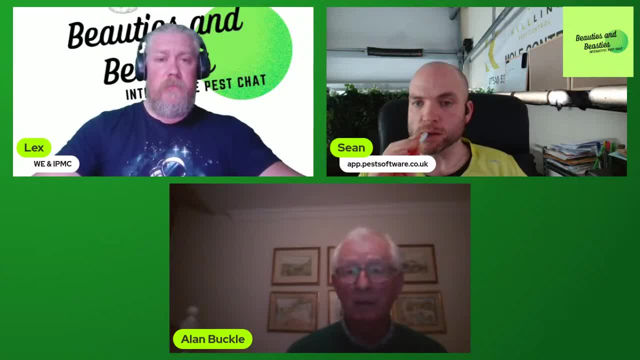 good alternatives, the things would not be on the market. let's, let's all clear about that. but the regulators are perfectly savvy people and they know there aren't good alternatives and we have to have them, um, to protect human health and animal health. um, and so they they are, they ask. 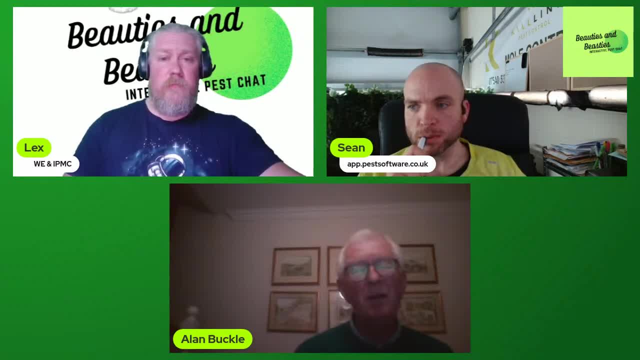 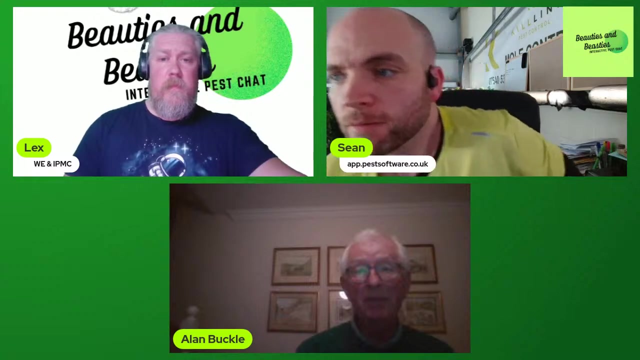 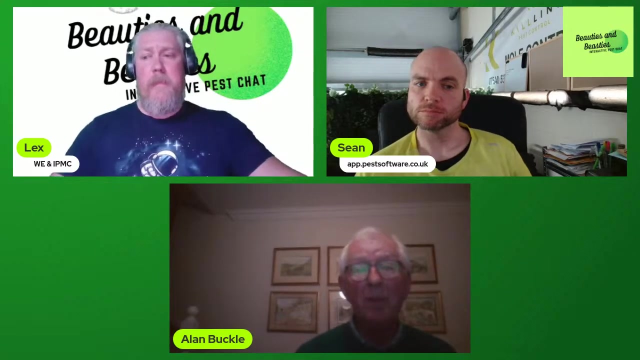 us to set up this regime. i want to be careful of how i use my words here, but it just the world in reference to the, i mean i, i know in the concept of gehört. so i'm a, i, i am a leader Traveller in Europe um Phi, Phi, Phi, Phi, Phi Phi. so 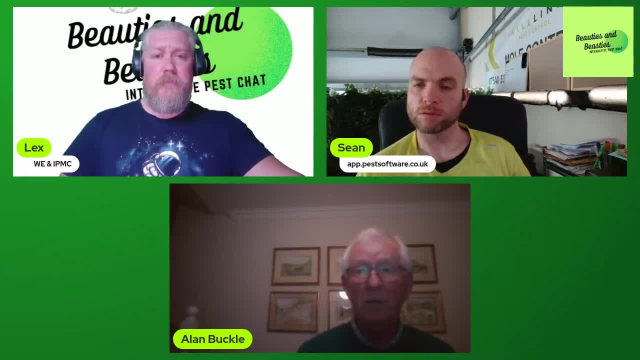 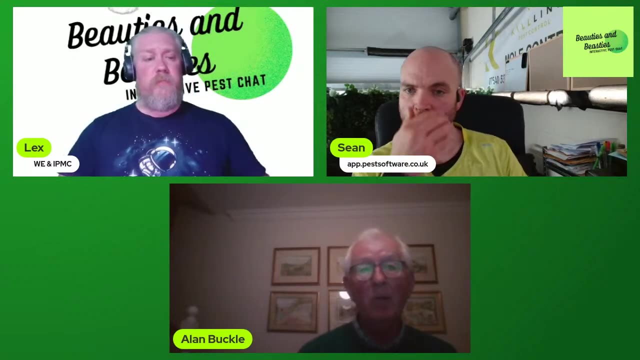 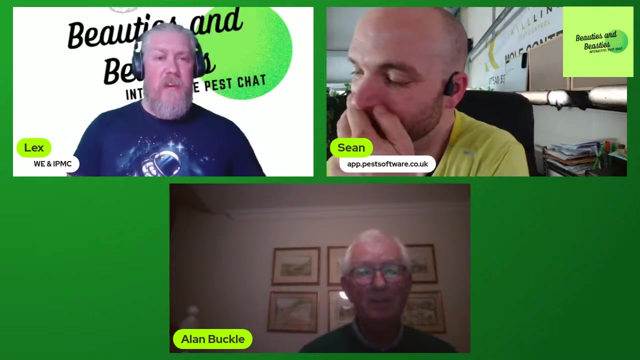 um, all sort of as a jury, an oversight group sitting in judgment, and I believe we'll probably find the judgment towards the end of this year or very early next year, when I'll be on a deck chair somewhere with my feet up. Alan, my understanding is in certain regulatory circles. 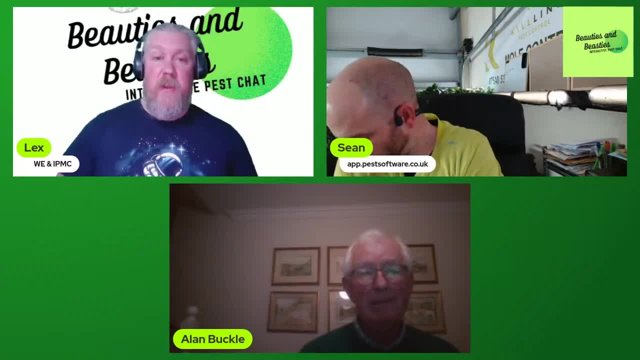 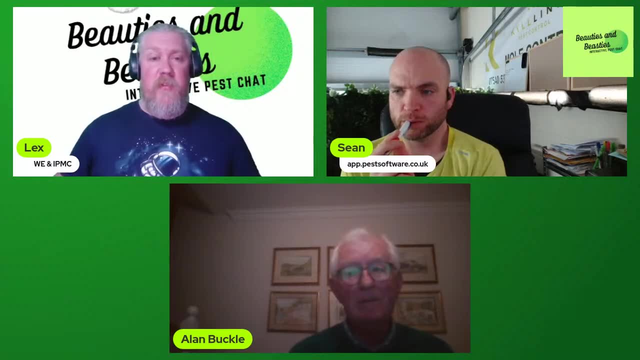 things like coeli calciferol are very much lumped together with the eschars And in other instances they stand apart. So of course you're saying you know stewardship has been focusing on the eschars very heavily here. 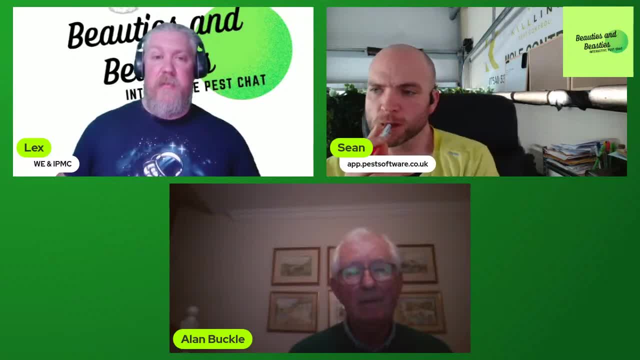 But will this review look at all of the biocides, all of the rodenticides to be used to control, Or is there a distinction between, you know, the calciferols and the eschars and the alpha chloraloses out there? 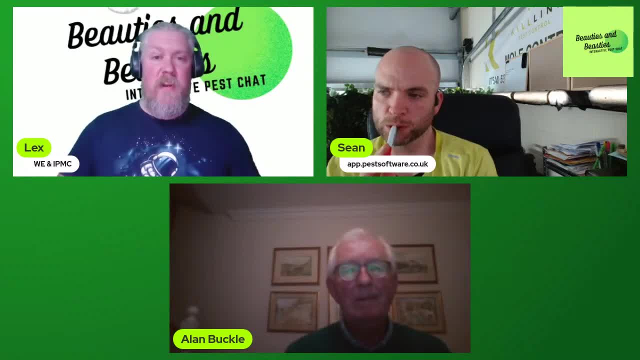 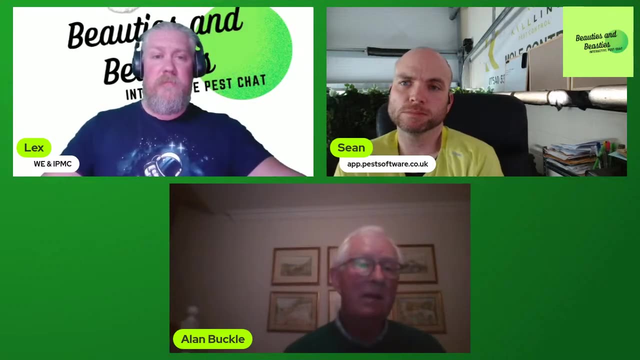 What will happen? Is this a threat to all of our chemical rodenticides or simply just the eschars? So there are two. There are two reviews going on pretty much just exactly at this moment, Alex. The one that I've been talking about and the one that I have been working on is the stewardship regime. 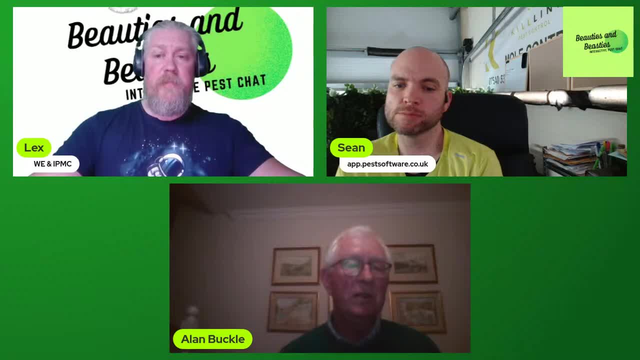 And that stewardship regime has been charged to reduce eschar residues And it will make a judgment on the success or failure of us to do that And that's purely to do with eschars. But in parallel to that process there is another review program happening and that's happening pretty much all the time to almost every biocide. 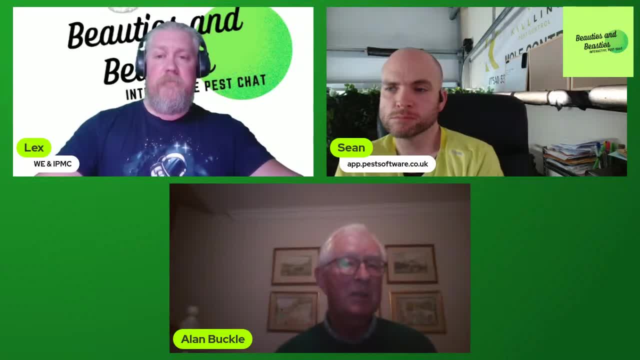 It comes around once every 10 years if the substances are not candidates for substitution, And it comes around once every five years if they are. So every five years all of these substances get a really thorough regulatory bashing. Now colicacinofrol will get that bashing in its time. 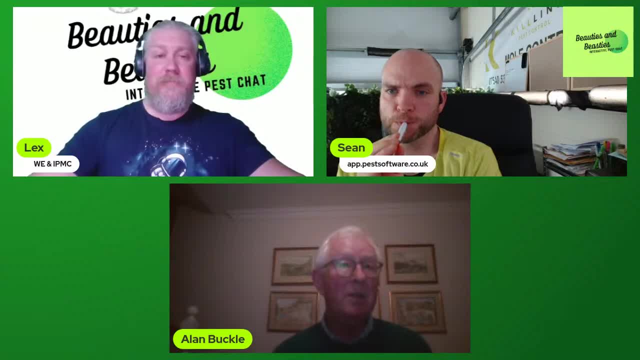 And, incidentally, colicacinofrol is a candidate for substitution because it ticks one exclusion criterion box: It's an endocrine, It's an endocrine disrupting chemical, And so it has got a cloud over it, in the same way that eschars have got three clouds over them. 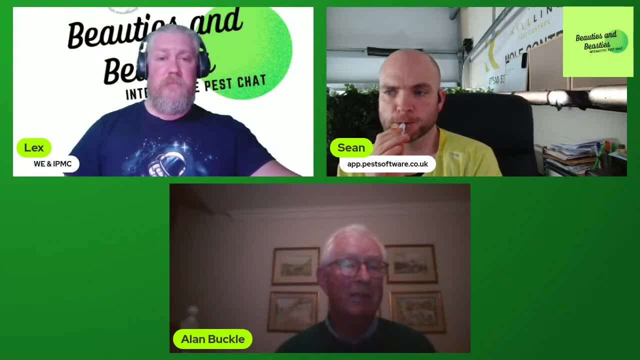 But one or three doesn't make much difference to the regulator. Both of them Okay, And so those are candidates for substitution. So it's those two reviews going on at the same time. I just happened to notice. I looked at my emails today while I was waiting for this to start. 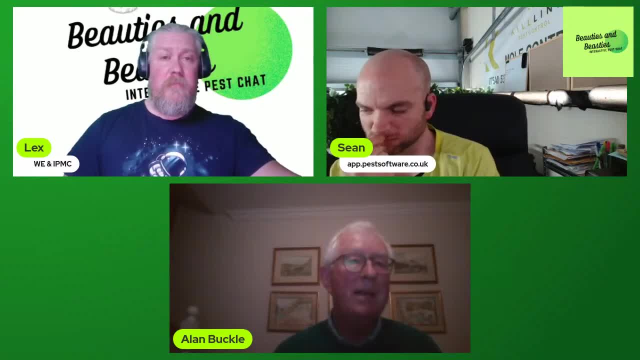 There's an email come out this evening from HSE saying that all of the, that second one, that five year review, they just kicked the can down the road for all of them, the anti-contraindicants, by two years because they couldn't meet the deadlines that they'd set themselves. 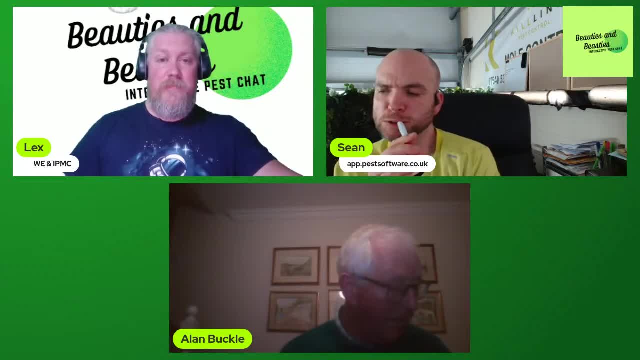 for um. i've got the dates here: um, they were supposed to be reviewed um by the by the end of june 2024 and today the hse said: well, we're never going to do that. so sorry, the commission, the european commission, said that they're never going to do that um and they're pushing it back. 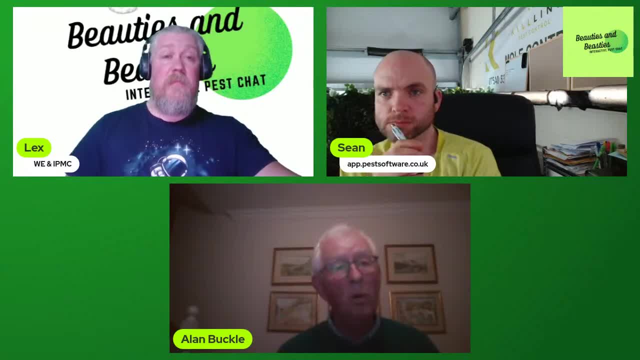 to december 2026 and what will happen in this country. i i don't know, but that's what the commission has has has done for the european union. yeah, i saw that. i saw that email as well, and it'll be interesting to see, um, what happens there, because it's it's like say they're being 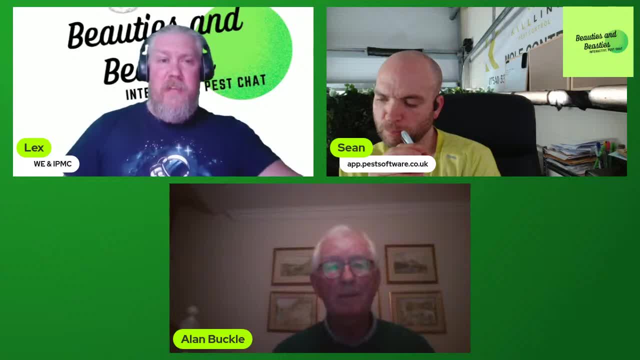 overwhelmed by by the data coming in, but it's, it's. yes, it'll be a case of watching that seat, but it's. it's interesting to see that, um, you know, coley has its own trials and tribulations, it seems, um- and i think hugh speaks for a lot of pest controllers here when he listens to this- 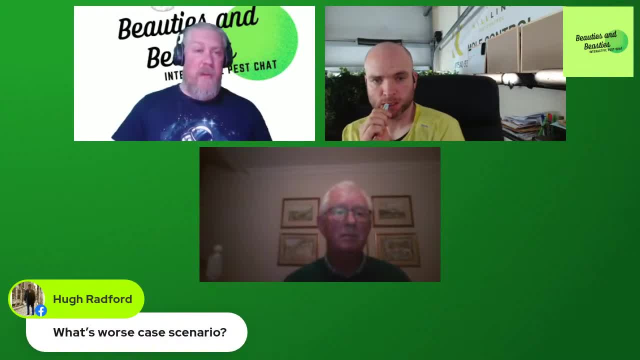 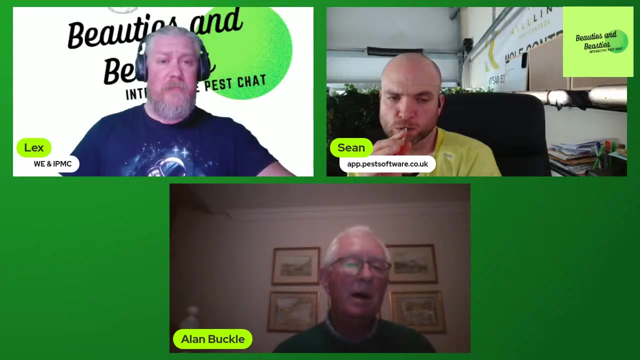 when he says what's going to be the worst case scenario then and i mean, is there? we all sit there and doom and gloom. we're saying you could lose everything, but i mean, what is the actual likelihood that we do lose everything? um, i, yeah, i, i really don't like to sit here looking into. 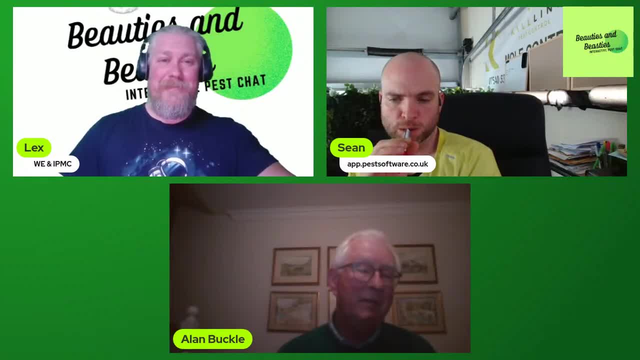 crystal balls like that, because there are so many different things at play. um what what i? what i would say is that there's a process, um called um in in this review and, because they are all candidates for substitution, they have to undergo this process called comparative assessment and what that. 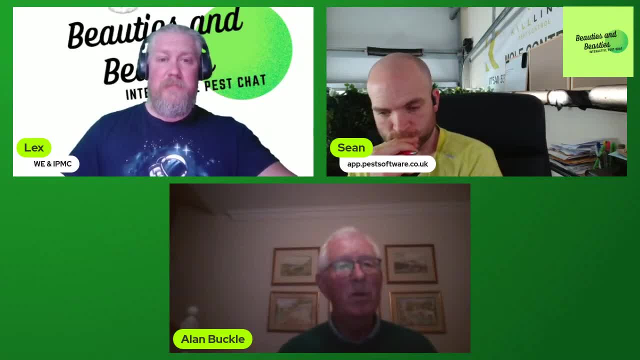 means is that the regulators um sit there with all the different rodent control options in front of them, um and they compare them with the one that they're looking at. now let's say we're looking at- let's just say we're looking at- brody for coon. so every five years someone sits. 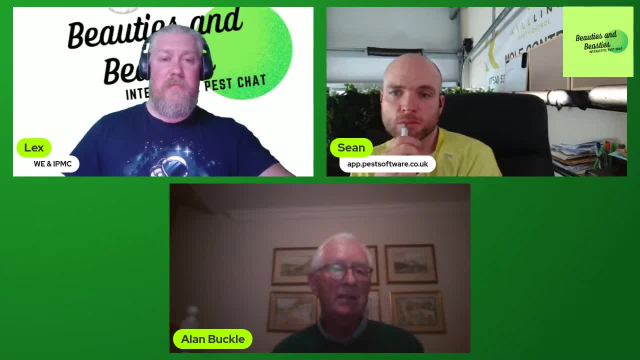 down and says what alternatives do do? do we have to these say, these escars, um, and there has to be a certain, a sufficient number of different modes of action and different types of solution that are sufficiently effective to provide effective rodent pest management. so the chance of losing 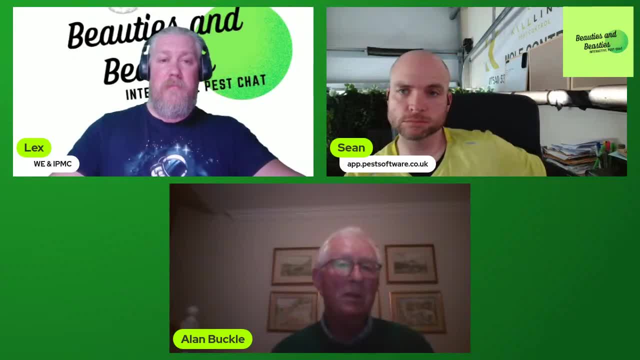 everything is very small, because that would not allow you folks to do effective pest management and that would not be what the regulators want to happen. now, what's what's going to happen to individual classes like escars or colicalciferol or others? that that, that's another. 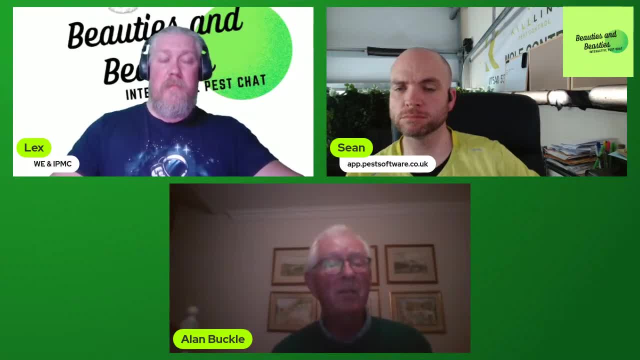 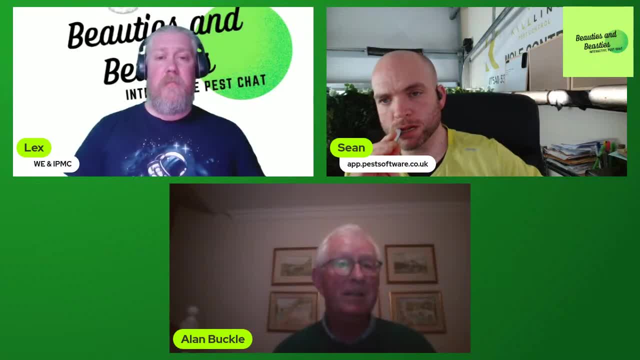 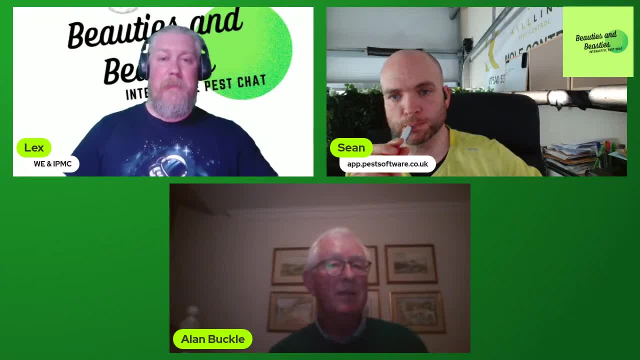 process going on since that happened five years ago, where the european commission has been trying to help prove that traps are sufficiently effective. and if, if traps become, in regulatory terms, a sufficiently effective alternative, then that is one more option. that's there, that um. it stands against the second generation. um, second generation. 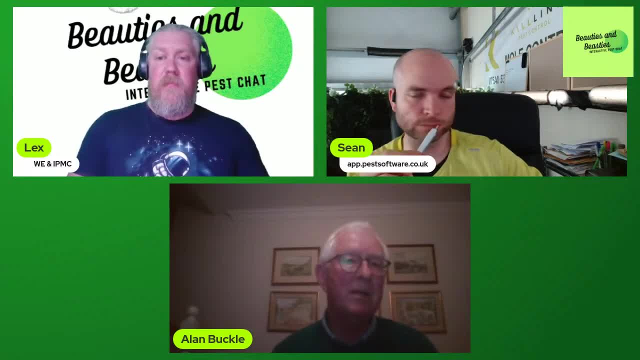 anticoagulants. so that that's. that's something to watch. i might say it's my understanding that, um, it's a uh. with the comparative assessment. it is three alternatives in: i think: it's 12 for rats and it's one for mice and it's one for rats and then the last one is for mice and it's. 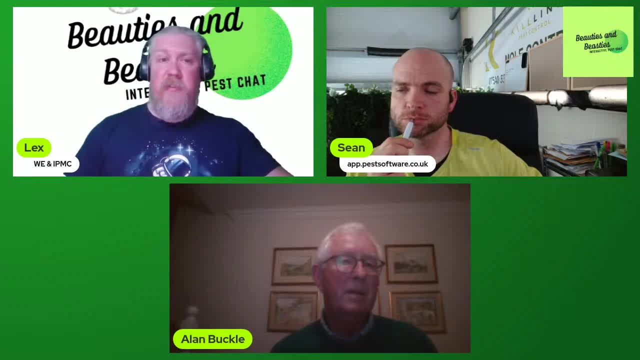 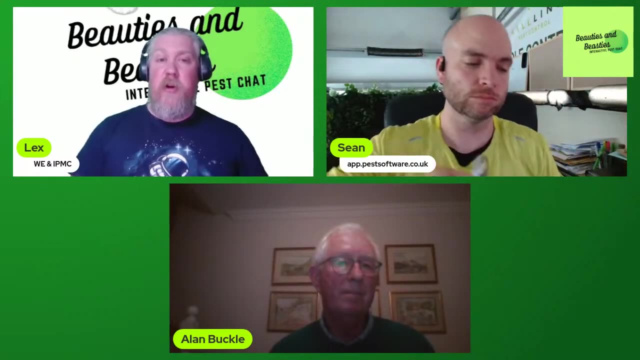 one for rats, and they're either a single-use pattern or an alternate use pattern, then there's two options and then there's three different scenarios that you find them in. and if traps are seen to be a viable alternative or a viable method of control, um, for either rats or mice, then technically that would make house mouse control inside. 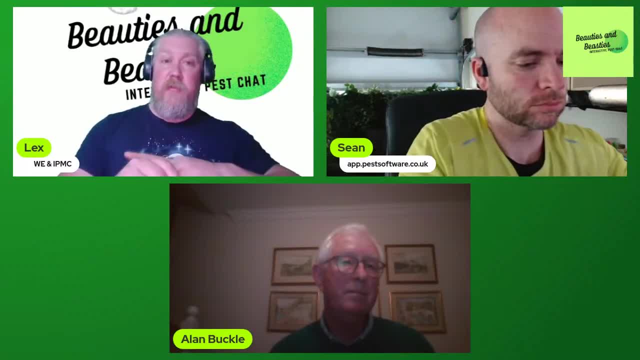 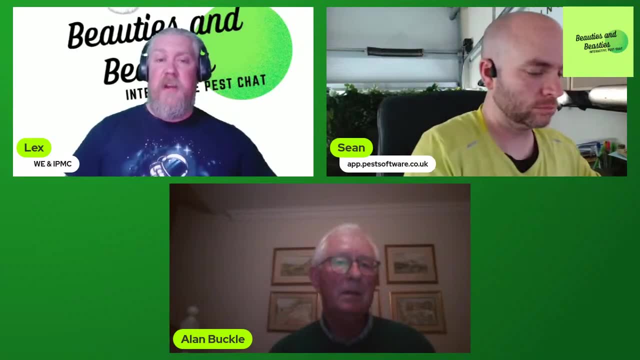 um, the eschars would be dropped because you have curly calciferol as an alternative, you have alpha chlorolose and then you have traps. that is your three alternatives, and therefore we would lose label use of mice indoors. um, that is my understanding of how, how that's potentially 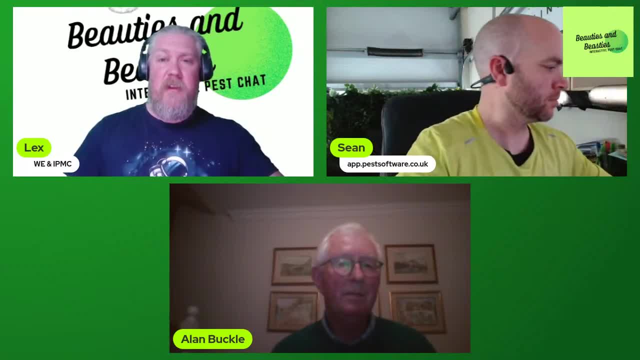 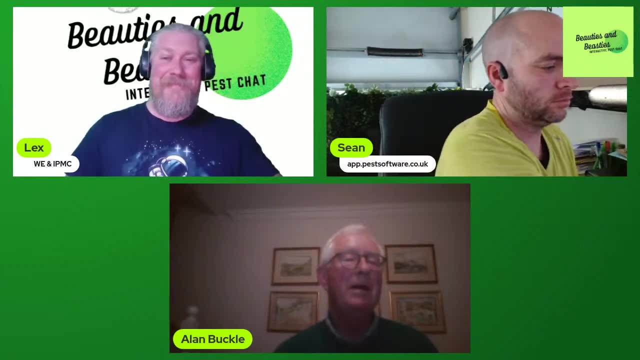 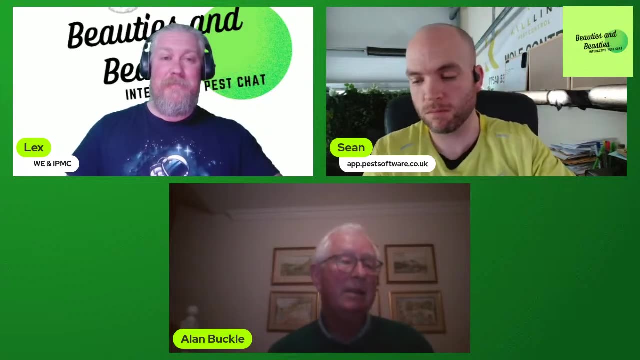 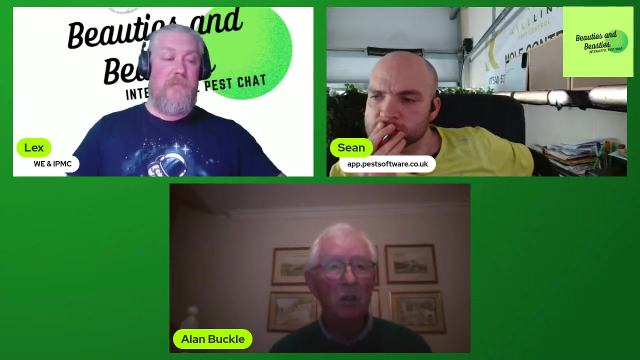 playing out, or am i, um, misinterpreting that in a in a way? um, well, you, you've, you've simplified it, alex, um, but but um, that that could be what, what happens, uh, and that that, that, that that process of comparative assessment is going to be happening. what i now see is they put it back for another two. 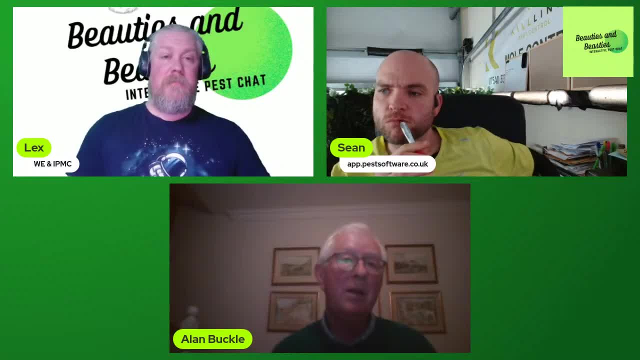 years. i thought it was going to be happening through through through this year, but we won't know for a lot longer exactly what's happened. it gives them another two years to find a whole load more um evidence that traps work than they had before. so that may work for us or may work against. 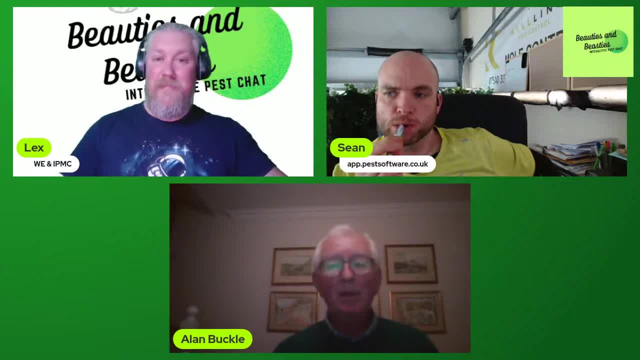 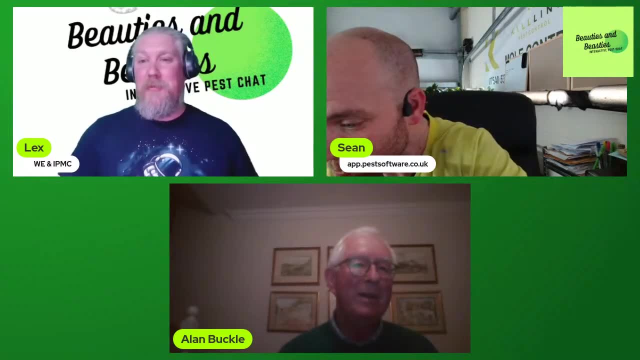 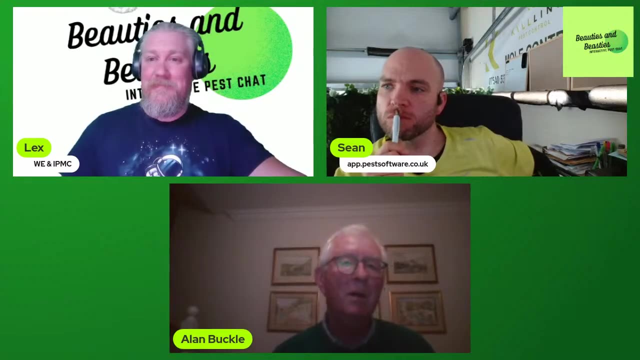 us. um, yeah, i'm, i'm looking down the side, i'm seeing questions going down there and i i pick some out. then pick some out for yourself. which which one do you want to answer? well, someone asked about how many companies um send, send crew, um rat tails. 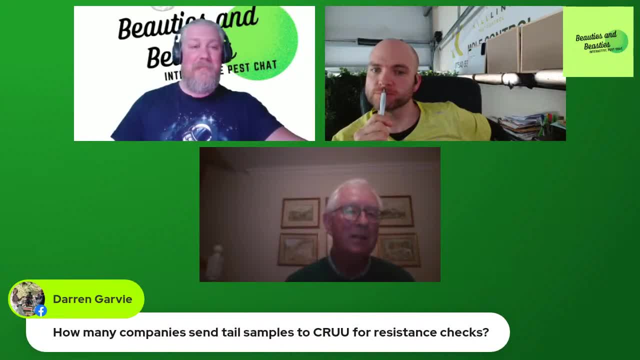 for resistance testing and you know, i'd i'd just like to say that that, um, we, we, we, um pay for a hundred tails to be done every year. um, and so that work is done by the animal plant health agency. um, i would just love a load more tails i'd love to get. 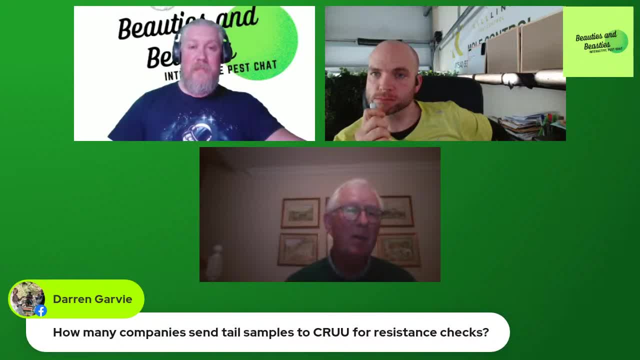 200 cent or 300 cent in. but for some reason we work hard, hard as we work, and we we do try to advertise it and we give out these free collection kits. we can never see the bust. the hundred, hundred and ten number each year, so i can't tell you how many different. 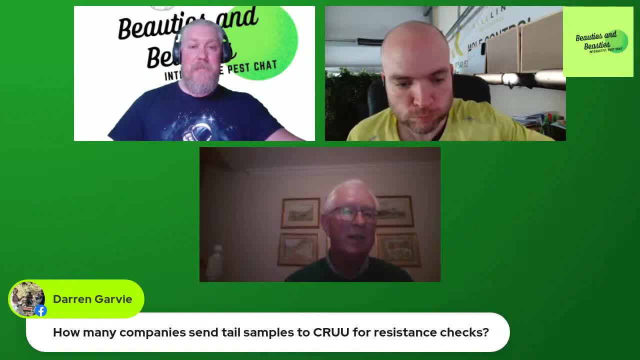 companies send tails. it's dozens of different companies, but we only ever manage to get a hundred to 120 every year. and if you folks want to send more, we would be delighted to get those, because we, we, we want more and more of those. uh, i'm going to jump in there from there, so that's, that's, that's. 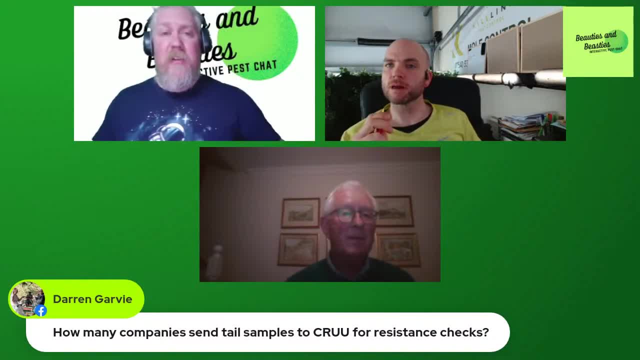 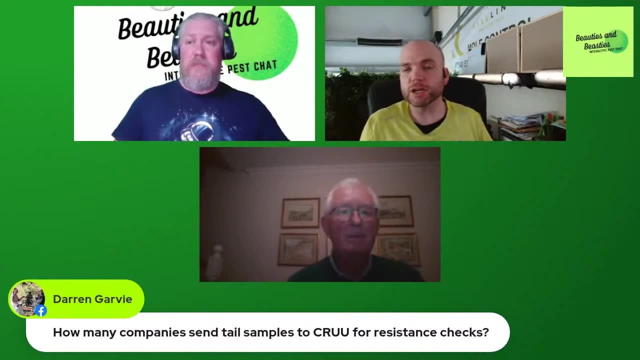 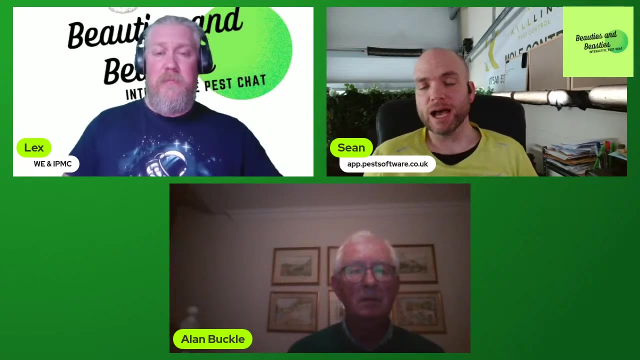 that one. yeah, sorry, go on, john. could you not just say if you want to use rodenticides or or, you know, second generation anticoagulants outside of buildings, um, or on an in and around buildings, then you have to be able to prove that there is a need for them and that those tails need. 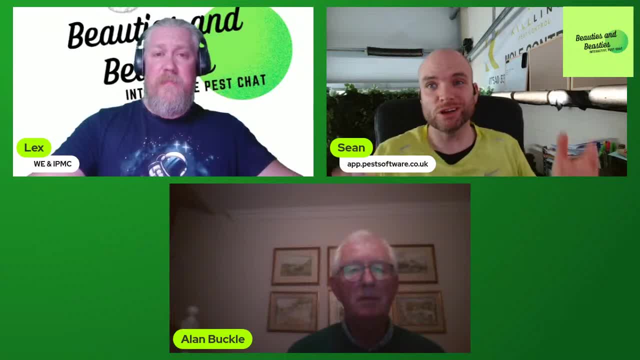 to be examined first, so you don't get people jumping to the good stuff, to the, to the strong medicine as a first case scenario, and then you'll get them starting to understand exactly why poisons are there. because if, if, the label is now law, surely we have that ability to put them in there. 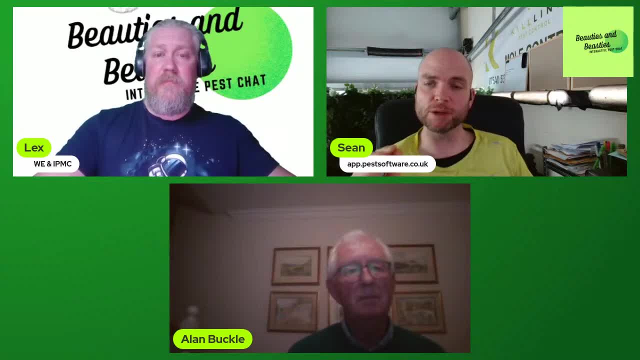 it in that to use those poisons in those circumstances, you have to be able to prove a need for it. that should be part of your due diligence and treatment plan, or already shown you should. and there is the the arag and the arak resistance maps, but you can't qualify that data. 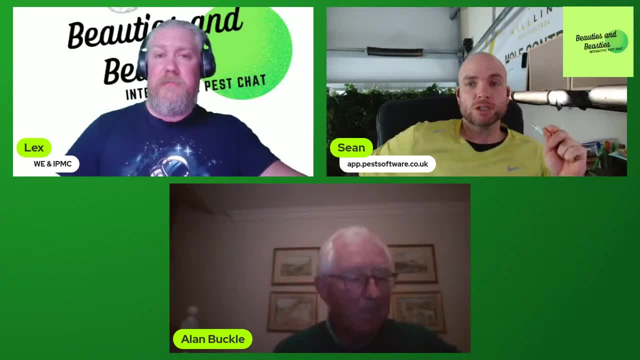 no, what i'm saying is, if you make it compulsory, because at the minute you can use it without the tail sample, without showing that there is resistance in that area, you can, you can drop into brodificum, you can go and bang brodificum on any farm around, yeah, and it's not needed. and 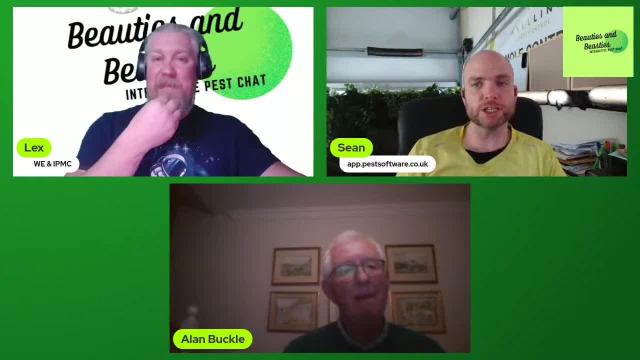 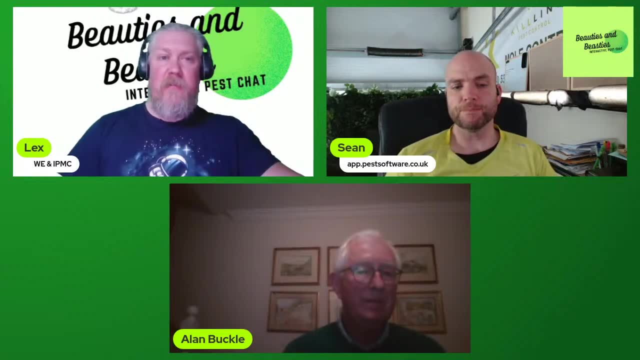 you haven't done anything wrong if you made it actually a stipulation on the label. before use it has to be proven. could that not possibly happen? it would take so long, would it? i'd? i'd love that, sean. i'd love for that to happen. um, but the the turn round type or dna sequencing. 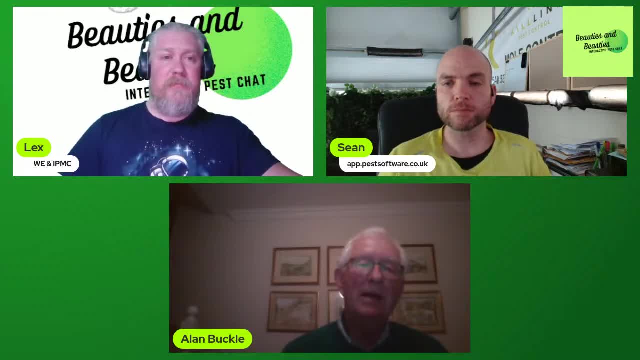 um would would not permit um a safe process if human health and animal health is at risk while we're waiting for a dna result. and so we we do, as alex has just said, um, it's absolutely recommended, guided, suggested, that you make sure you know what the resistance status is of the rodents in the area that you're working in, and 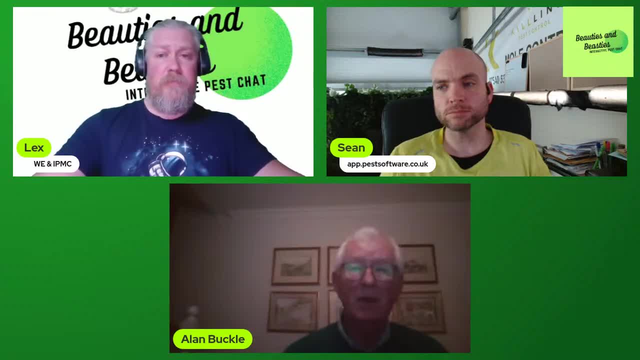 if, if they don't need brodificum and you can use bromodialone, or if you, if they don't need bromodialone and you can use something else. um, that's what you should be doing. i i've just been revamping the crew code of best practice to take out all the records to use warfarin and 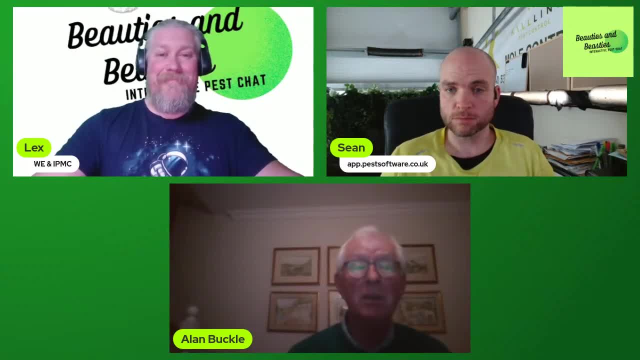 kumatetra, where you've got no resistance to anticoagulants, because all of those products have just have gone, apparently, but there's one. no, i do, i do agree, but the the, the mechanism for making it a prerequisite, is just not there yet. we haven't got the. 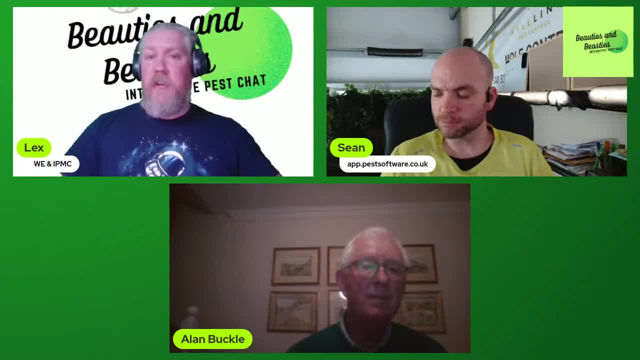 technology there. okay, i'd also like to say to to also augment alan's call for tail samples. there is a huge bias in a lot of the data that we get into crew and r-rag that people only send in tail samples when they're having problems and it kind of creates a bit of a skew in the data which. is if you've got a problem, you'd like to give in to some of the ends you know later on, um but uh, and you help professional determinants in ways that they might not have the have without the schools that things have been and create a kind of indirect unfaithfulness, i think to, whereas respect to what the 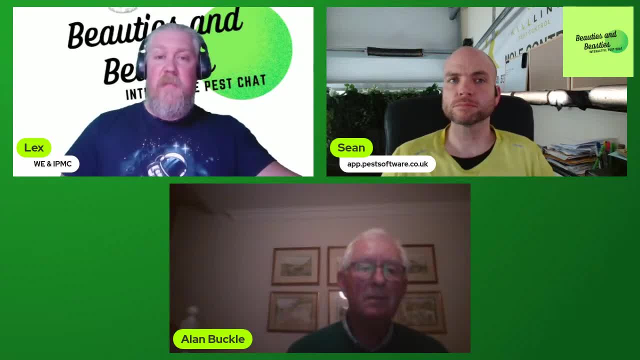 tend to send in a tail sample. you are kind of already um qualifying that. what i'd, what i personally would like to see- and um alan may have his own views on this- is for people to send in tail samples um just as is if you've got a good, nice, juicy tail that's not falling to bits and 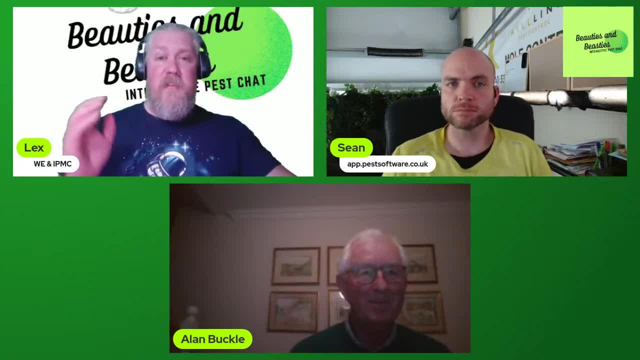 the meat's, not sloughing off the bones like in a good hog roast um to to send it in, because at that point we there's as much information to be had by finding susceptible animals in areas as there is um finding resistance animals and especially when we say this, that people are. 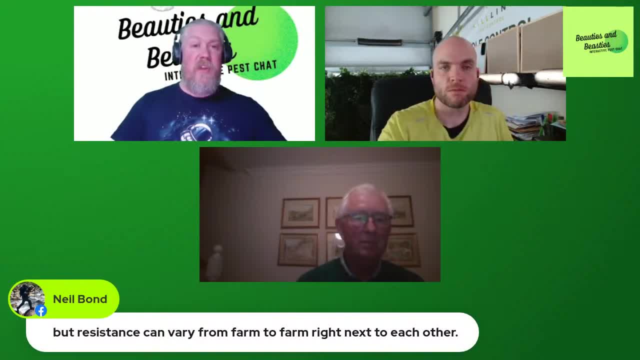 noticing that resistance can vary from farm to farms right next door to each other. but of course we'll send in tail samples for farm a, because we've got control on farm b. we don't send those tail samples in and so it really skews the data. so if you want to send in those other hundred of 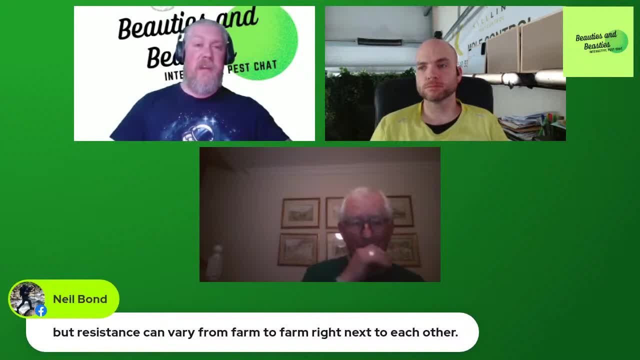 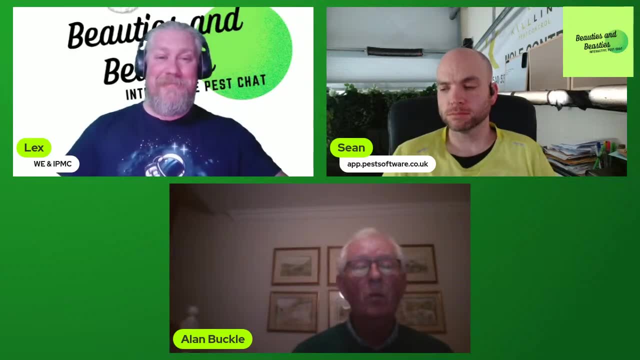 just randomized samples. there is as much information to be had in that as not. don't wait for there to be a problem. that'd be my request, you well, um, so i, i, i couldn't agree more that, um, our process of sampling these tails is is biased, because we strongly believe that we get tails from people who are having problems. 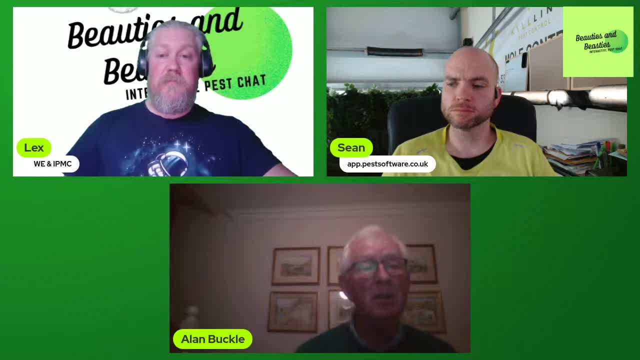 getting control of something. and what's even worse, quite often they would have been trying and applying some some rodent side that hasn't worked very well, but they might well have taken all the susceptibles out doing that and have just the resistance left that they then. 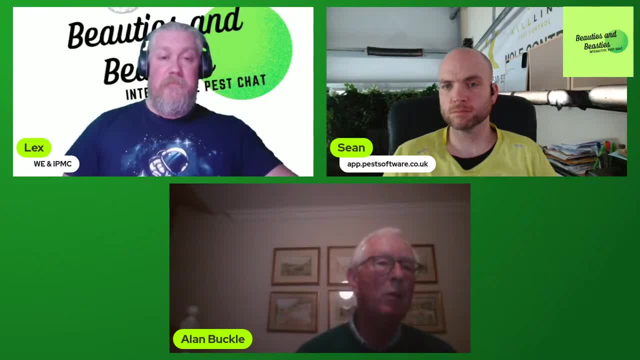 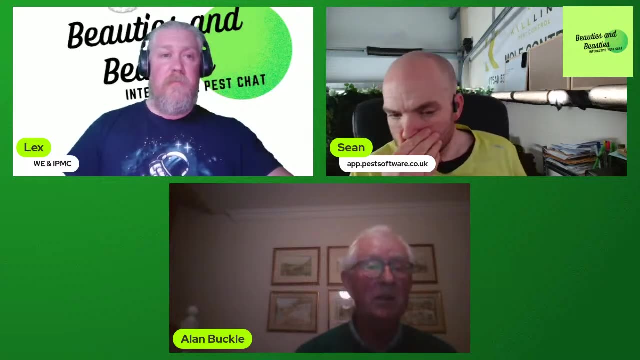 send us the tails off. so it's a double whammy in terms of bias. so completely agree. um, all i could. just if i could just remind you. on the crew website there is a sender tail box. we will send you the kit free of charge within 24- 48 hours of you asking on crew website for. 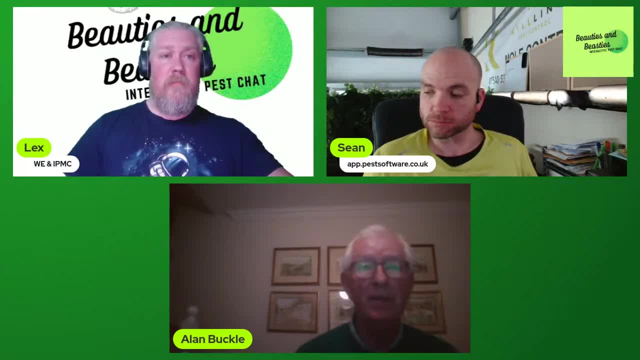 um, a tail testing kit. so, please, please, do that. and, as alec says, we're very interested to get tails of of of our quality and so, um, yes, um, we're gonna do ausuot style uh, maintenance kits. we'll give you our hodgepodge are our practice kits. we're very interested in, um, uh, our practice kits. we do uh. 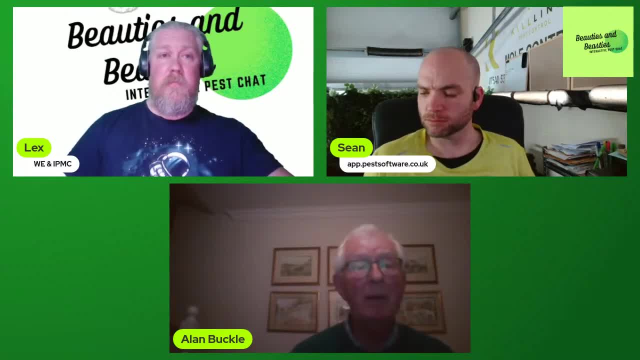 all kinds of things. so we'll give you, uh, other types of tools and um, um, we've got some347 Kelloggs of both rats and mice from absolutely anywhere, and not just because you think you might have resistance. yes, um, i mean, i'll be more than happy with that. we're coming up to the one, would you? 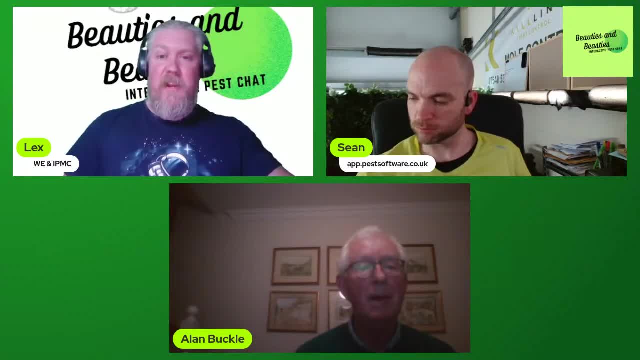 believe we've been talking for an hour and a half now now, alan, and it's absolutely flown by um. so with that i i quite like you know, because we're trying to wrap it up around about the one hour, but absolutely, um, if you wouldn't mind just picking just one more, one lucky contestant from 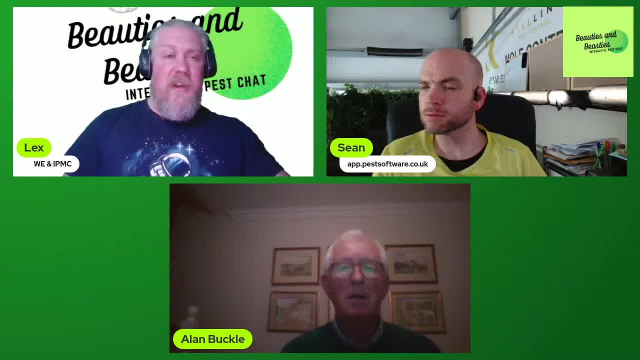 the um from the comments there, just to answer the questions of and um, just while sean and i think of any any others. i've got two questions, i've got, i've got two questions left and that's it, and then i'm done. well, i've got a million, but i've got two. i'm gonna ask tonight, same here. yeah, so so. 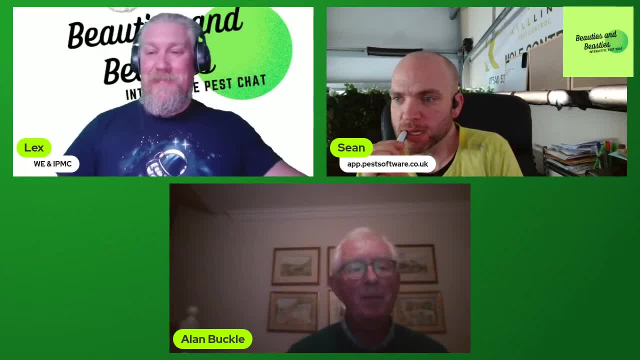 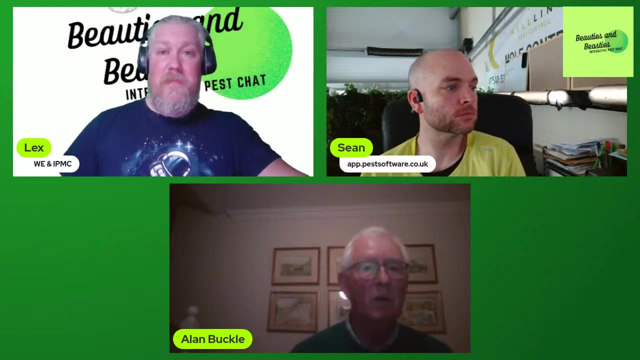 okay these questions. can i just say: and um, there are a number of ways that people can get in touch with crew um. crew has an office and it can be contacted via the um info um web's um email address and every single email that comes into that address comes onto onto my desk and what? what happens? 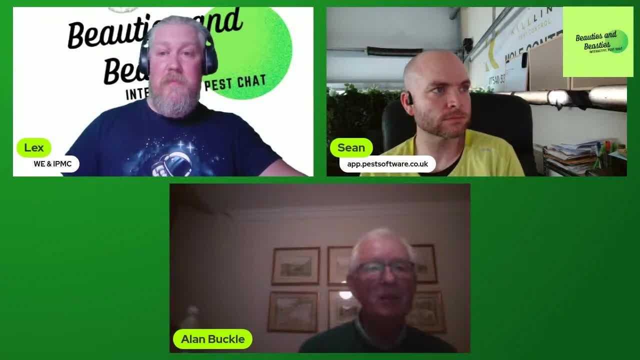 there's a sort of a triage in the office and if they're to do with training and certification, it goes to one person, if it's to do with point of sale, to another. but every single one of those questions will get in touch with the crew and they can get in touch with the crew and they can get. 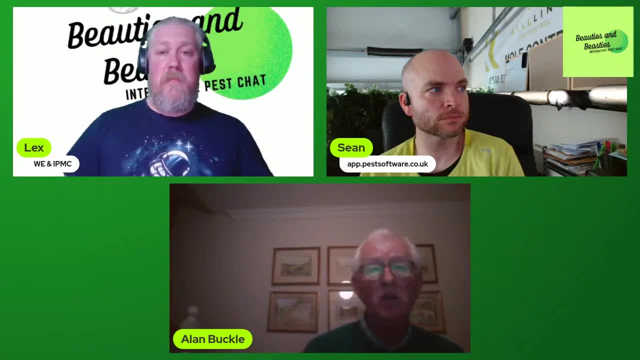 answered by crew, and i get quite a lot of them. so, please, i'd like to make sure that if you don't think that, um, we don't want to hear um, please do send your questions in and we, we will do our best, and we do our best to answer every single one as quickly as we, as we possibly can. so, um, 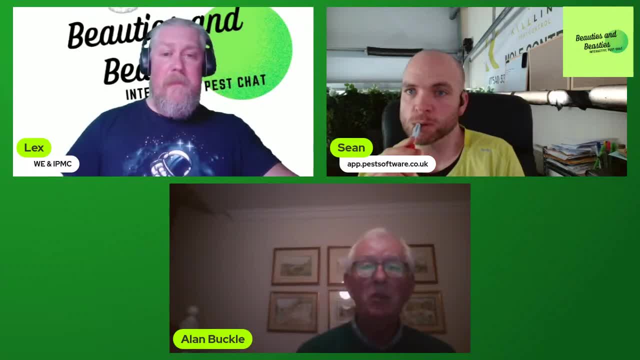 please, please do that. so but, sean, you, you, you had two, two questions and i have one. what so? the first? I didn't. obviously my question was rubbish because I had far too much in, but there was one bit was missed which I'm really personally, I'm really interested in. 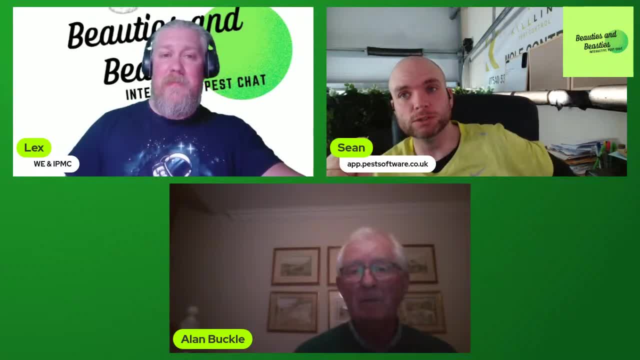 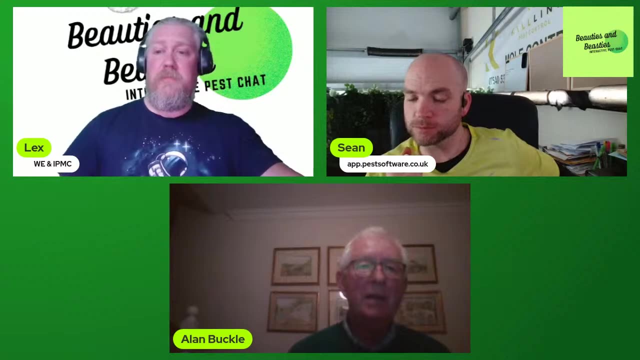 What pressure does the agricultural sector put on crew, if at all? So it's one of our three sectors and it's no more or no less important than the others. When we set up the stewardship regime, there was pressure because the intention with the stewardship regime right at the start had been a level playing field across the board, that everybody would have to be trained. 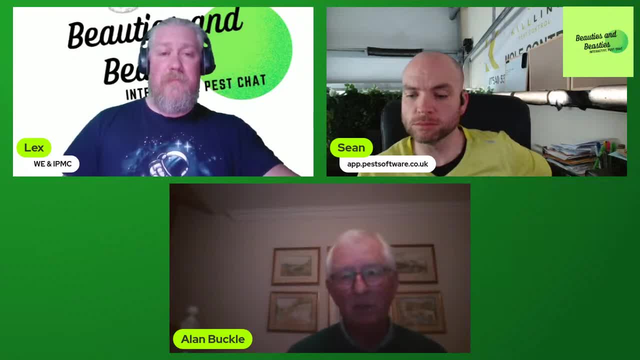 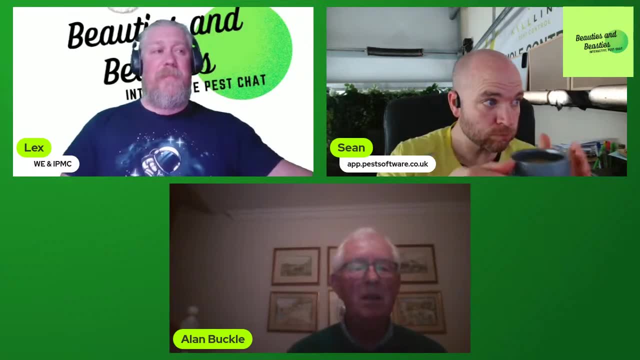 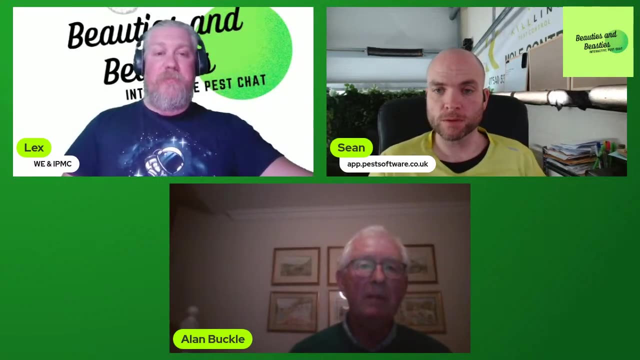 Now, please don't talk to me about the quality of the courses and how long they take, but the first step was going to be that every single, every single person who was going to be considered to be technically competent would take a course, sit an exam and pass it. 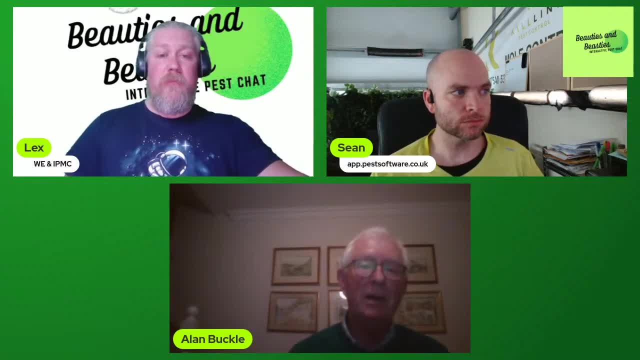 And that was where we started with the stewardship regime. It's taken us almost 10 years to get to that point where we wanted to be at the start. Now you asked about the pressure I got hyped up in front of the minister for the 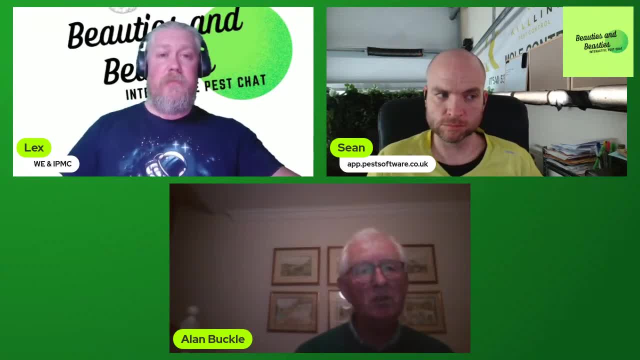 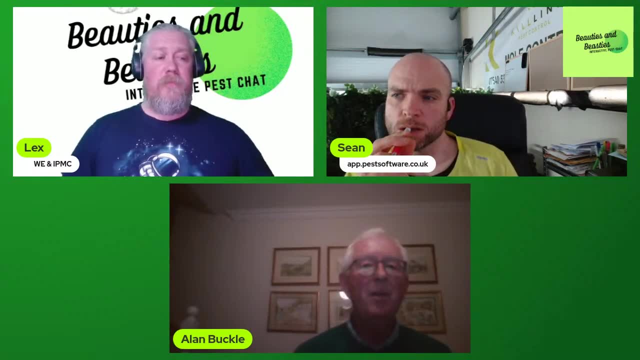 I HSE is in the Health and Social Services Ministry and when we were going to apply that requirement, the farming groups worked out that we were going to have to train something like 150 farmers every day for the for the time that we had left. 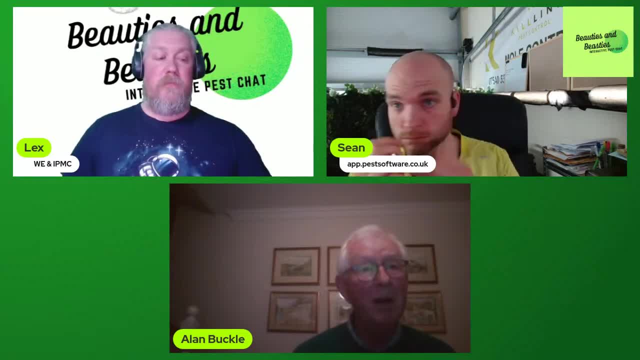 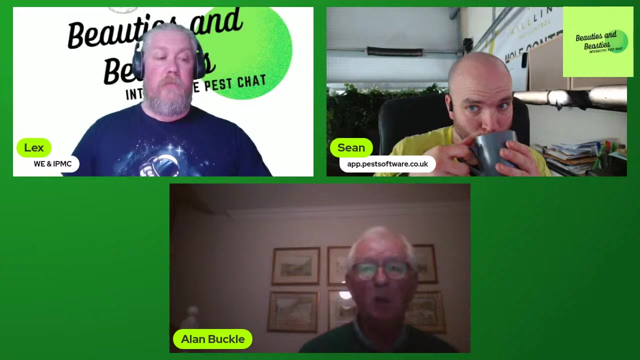 And it was just impossible to do And we got hyped up in front of a government minister and We got told to find another solution in order to get this thing off the off the ground. Now, the other solution was that we had this interim process where farmers who are members of crew approved farm insurance schemes are considered competent. 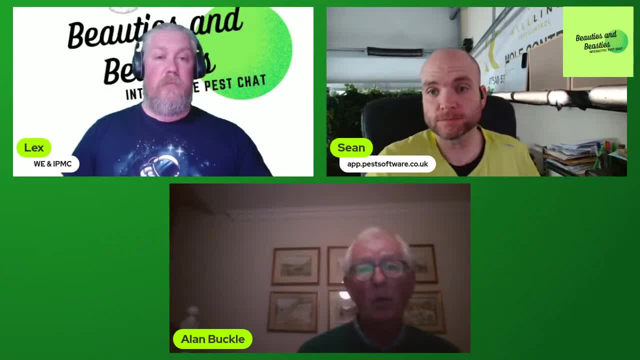 And we decided to put an end to that, that that won't be happening after two years from last January the 1st. I would say that that didn't make any of the farming Sector very happy at all and pressure was brought to bear not to do that and the the the crew directors held their ground and said, No, it didn't happen last time. 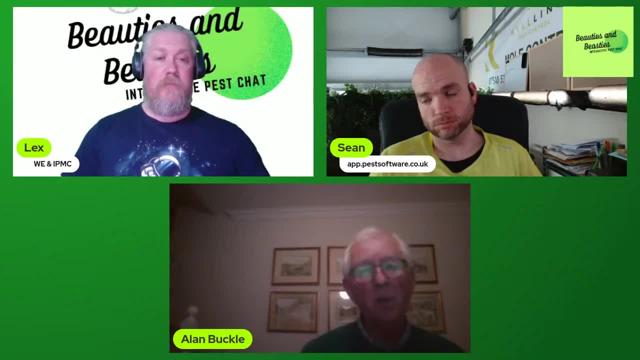 It's going to happen this time around So but we get pressure from all of these groups at different times on different things. Can't count the number of times I've had someone from professional pest control talk to you about amateur For, For amateur products, for example. 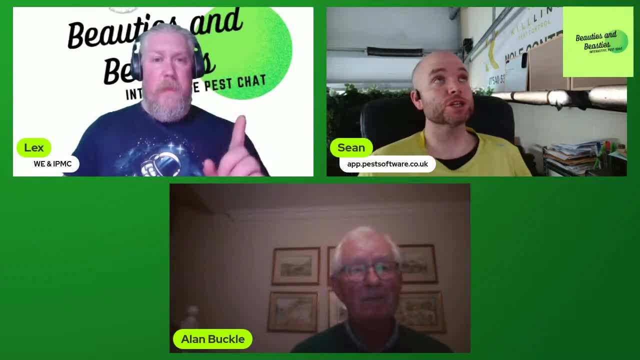 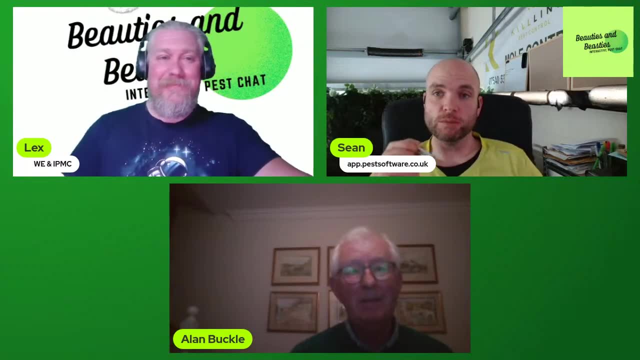 Get it, get it, get it. and then my last question, I promise, because I think this will absolutely blow pest control as minds. You, when me and you were talking to Pestex, we were talking about LD 50 numbers in relation to dogs and you you explained the process and one of the guys I was with he actually got caught into all this, etc. 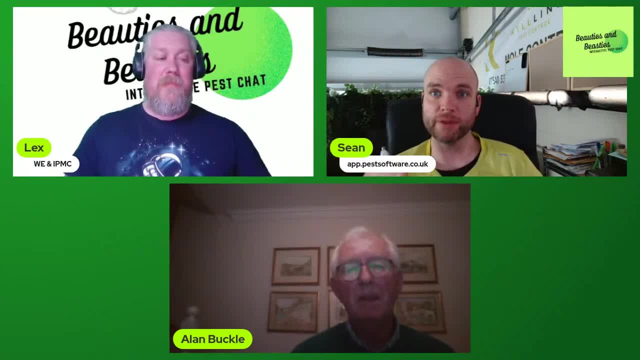 So I would love you to let people know how they come up with the LD 50 numbers, because it was a real eye opener for me. I'm, I'm trying, I can't, I, I can't remember what I said this time last, last night. 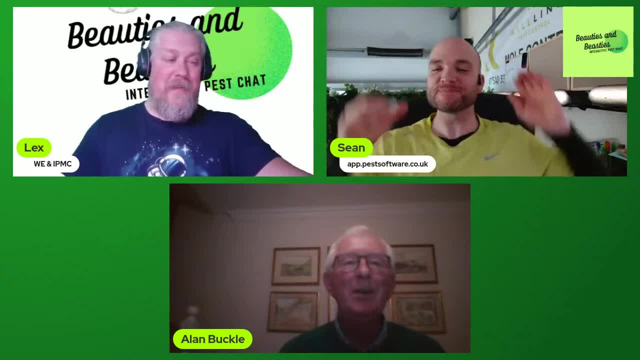 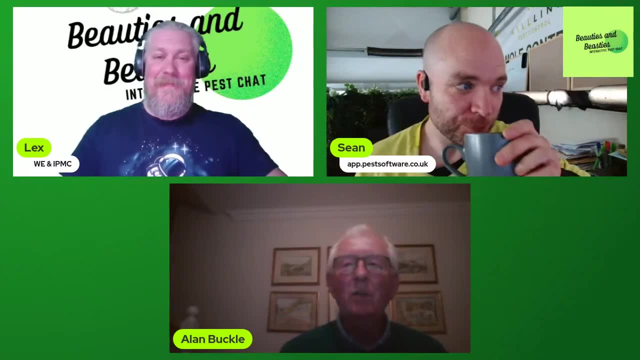 Sure, Yeah, John, John, is there a reminder? the conversation? No, no, I do. I do remember I'm, I'm joking, I'm joking really All right, So I don't want to sort of necessarily. 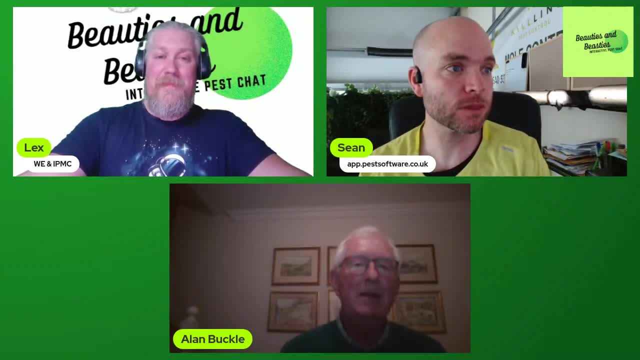 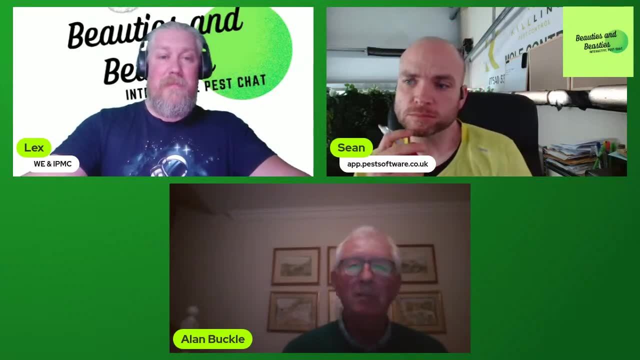 Men? Well, I don't know either. Trans argue, the doctor, mentioned active substances but that there had been some problems with with dogs and some dogs were have been killed and some made extraordinary ill, And Pascal reviewers were letting the manufacturers know about that happening and the manufacturers were coming back with information about the LD 50, Two dogs of some. that's some of these substances. 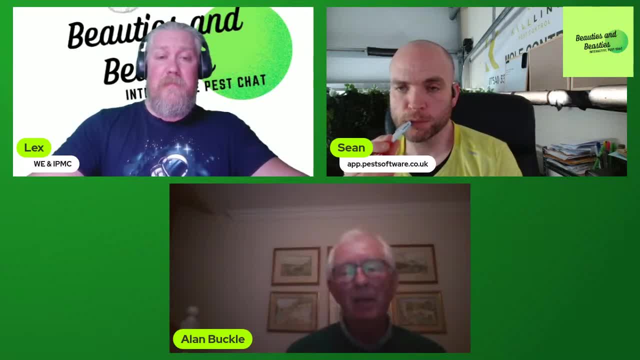 points that i try to make it and um, it's not the nicest sort of science to do and i've done some of it or had some of it done. i haven't done it, i've had people do it on my behalf, which is dog ld50 tests, and that's not something you really want to do. the sample sizes are always. 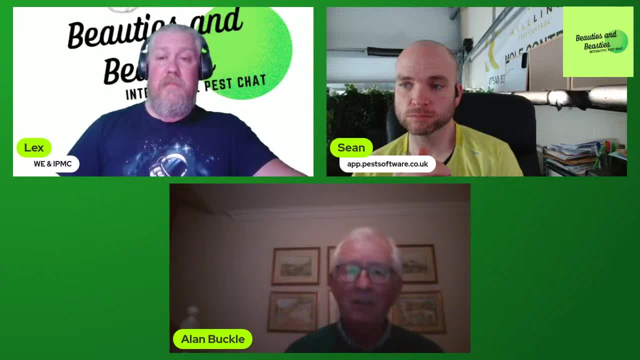 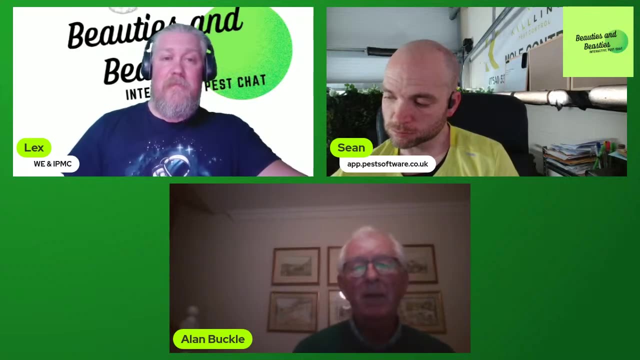 very small, because you can't. you can get 50 rats per sample size to do an ld50 for a rat, but you can't get 50 beagles to do an ld50 for a dog, and so the sample sizes are always tiny and that there are now very strict rules about how to work out ld50s. and the other thing is 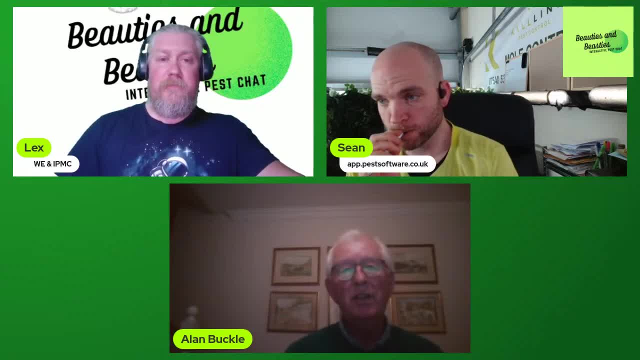 any talk about ld50 means that you've killed half of the dogs and half of them have survived, and that that number is of no significance to the safety of- you know, of the dog's life, and so i think it's important to think about that, and i think it's 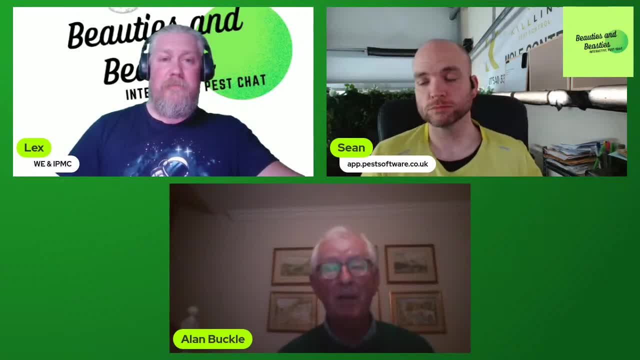 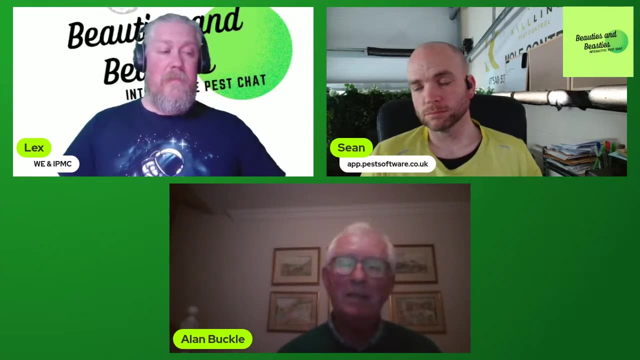 important to think about that. and i think it's important to think about that because you don't want any dogs to die, so you want the ld1 or the ld none. so the ld50 figure high or low is is important, but it really does doesn't help. professional, professional pest controllers. 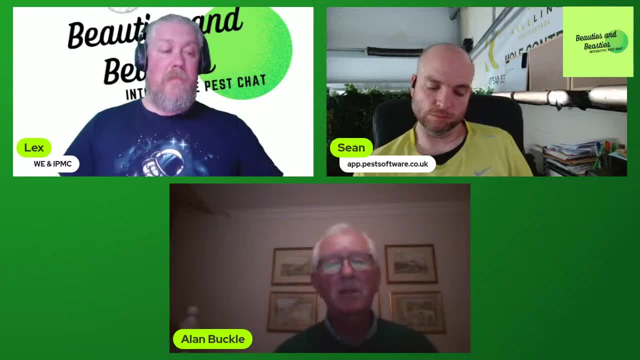 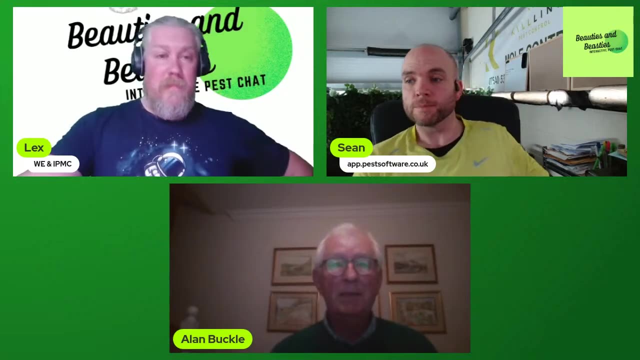 i know this was um- was being talked about by a particular active substance, and that particular active substance just has just come back back onto the market and we will. we'll have to just wait and see what happens with it. so what, what? no, what are? so sometimes i pick things up wrong. you probably guessed that. so my understanding of it is and: 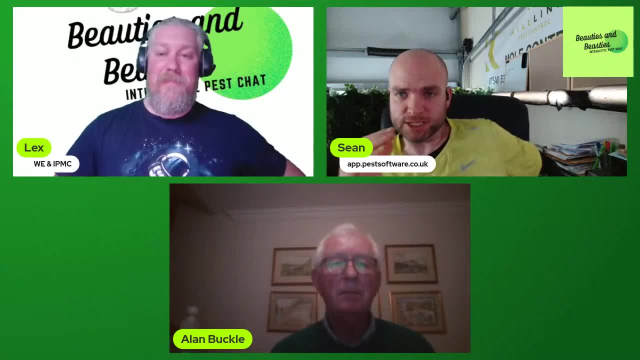 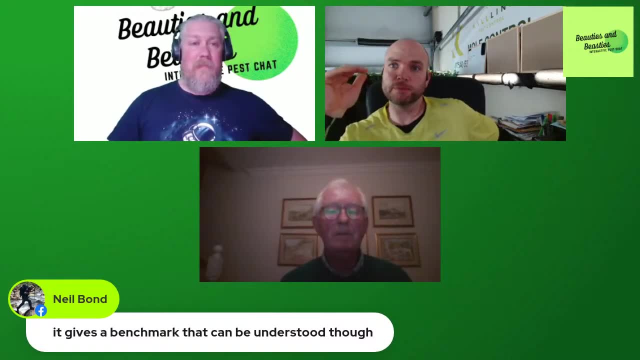 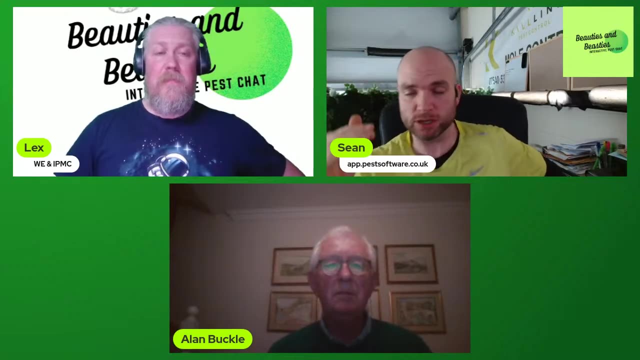 correct me where i'm wrong. when they do ld50 tests for all actives, so without picking on one for all of them, they have a a number of ld5. they're also a number of ld10 allen's. ld10 allen's that we call the dog antlers and the ld20 is the name of a type of animal that. 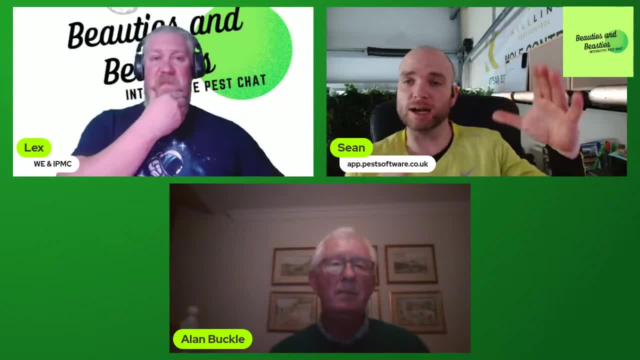 has a ld20 and that ld40, as we said, is a human: ld40, ld40i, ld40i is the animal that can eat half of the ld40i ld40i, and then the dog can't eat all six of them. it's- uh, it's, it's our job- of the animal. we show that the dog can eat half its body weight of this stuff. 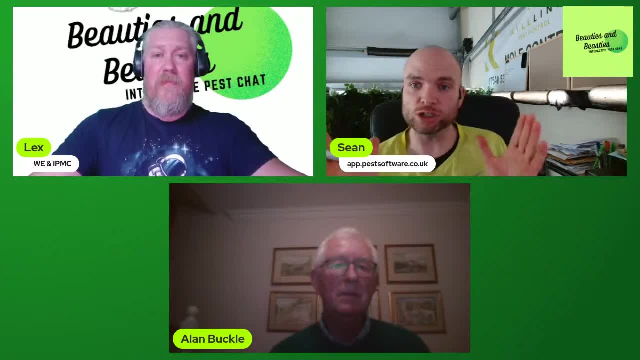 so that's all right, but- and i would take it as gospel- but what you're saying, there is- and i agree with you- 100 of that conversation. we basically have to start thinking to ourselves: they're not allowed to sniff of this stuff, not a sniff like because we, you really can't say with any certainty. 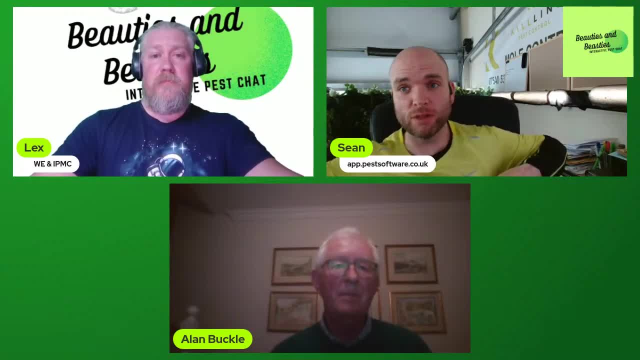 what that ld50 would be for that dog. on that day you can see what happened with the four in the lab or the two or three in the lab, but not the the wolfhound or the the spits or whatever it is that's living in a different environment, getting fed differently, being looked after differently. 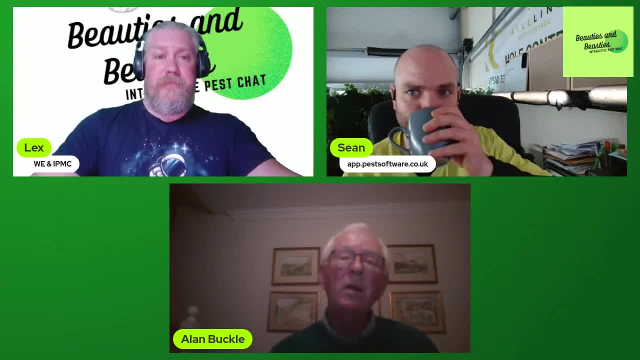 etc. is that right? have i got that right or wrong? well, no, that's that's. i mean, that's that's absolutely great great print principle to apply. i see that somebody in the chat um said they do give some some comparative um information. so if one substance 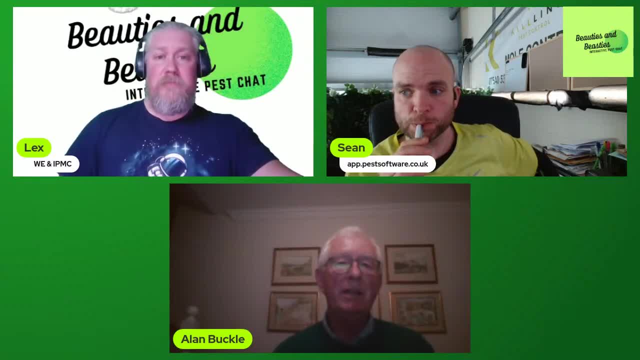 has a very high ld50 and one substance has a very low ld50, then you can take that comparison and that gives you some useful information. um, but what was happening in this particular case? that happened to the guy who was on the stand that we were talking to. someone from a company had said: 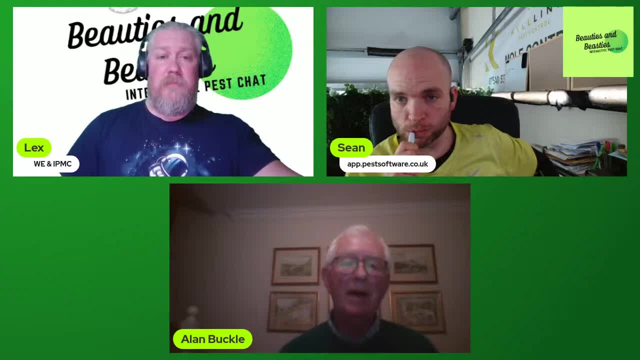 um, well, the ld50 is this, um, and it would have had to eat two kilos or three kilos to get that dose. well, if it'd eaten two to three kilos, um, that would have killed 50 of the dogs if that was what the ld50 was, but often that line. 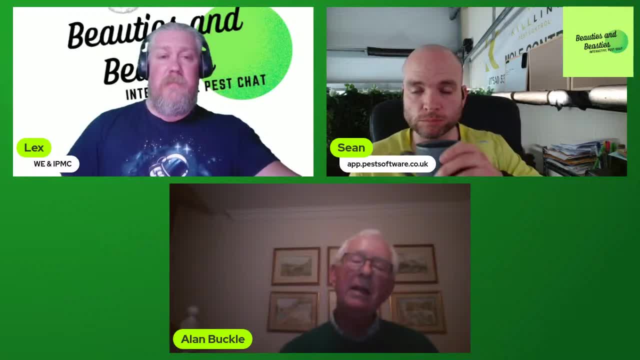 is not a straight line, and and so it may well be that a much lower dose gives an ld10, and so you've only got to poison 10 dogs and you're going to get one dead one, and we don't want any dead ones, and so toxicology and safety um. 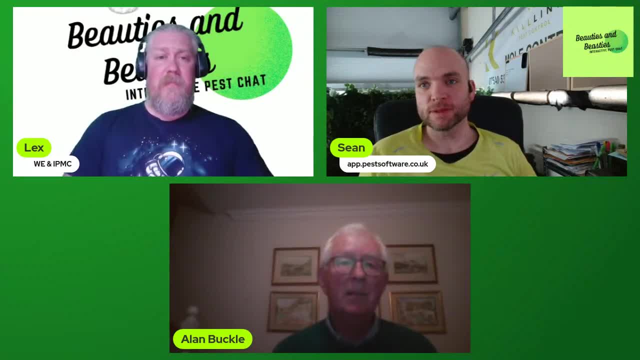 not very good. um guidance, really, um in in that, in that's in that sort of way, i think. i think, sorry that that sums it up, doesn't it the ld10? what's the ld10? because you're working on having that one dog in the ten that would get rolled over with that stuff. so it really is a like. 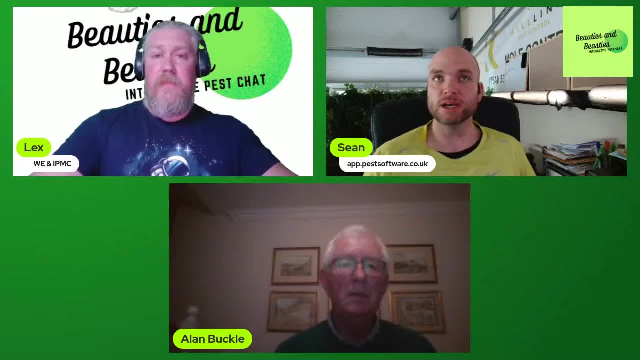 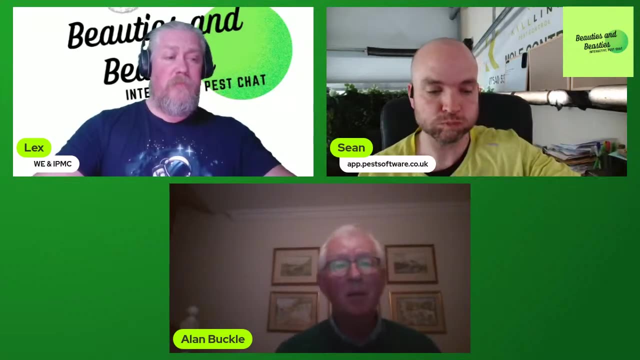 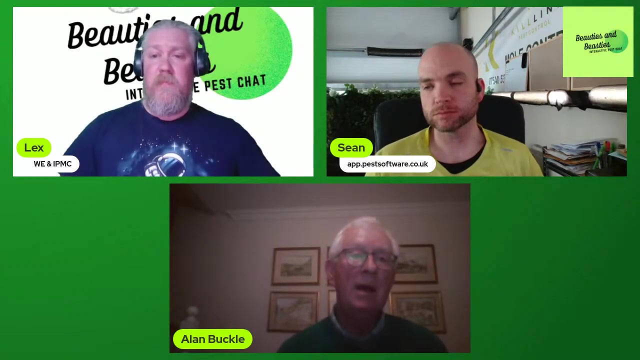 you can't. you cannot rely on that ld50 as a sort of safe level of exposure, can you? you can never cause anything safe. yeah, it's just one bunch of dogs. it's almost always just one one breed that they use and um, breeds, breeds vary, the um how, how, how well a dog is has has lots to do with it. so, yeah, i. 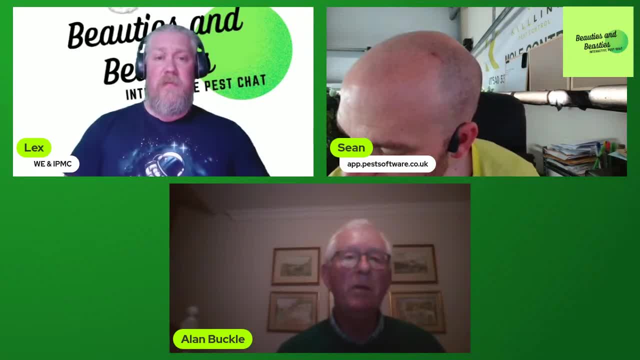 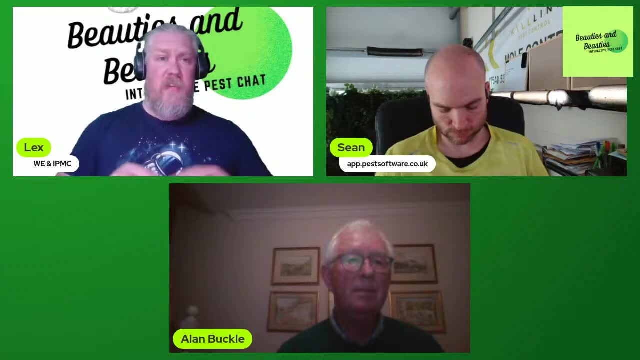 so hopefully, i, i, i sort of came back to more or less where we were when we were: um, yeah, i'd like to chip in for for this for a second, because, um, if you imagine it doesn't matter, even if you imagine a best case scenario that you're grading on a, a bell curve, here you 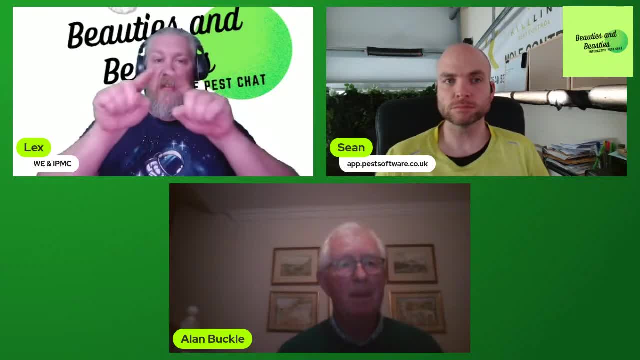 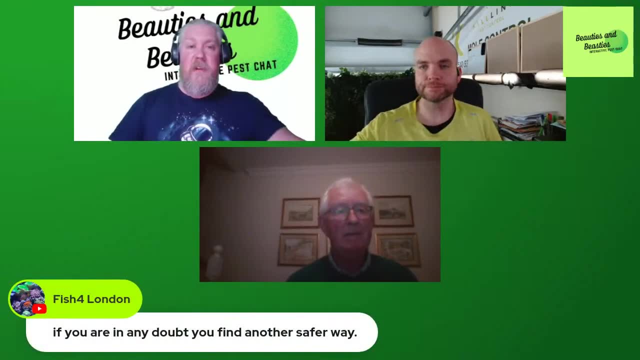 know it's um the 90s. it looks like this: either which way around the 50 percent, it's probably not. it's probably what we call tail, that leans probably more towards one side than the other. but even if you do assume that it's a bell curve, there are going to be. 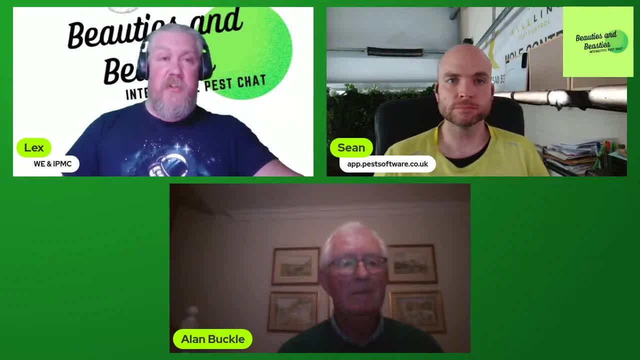 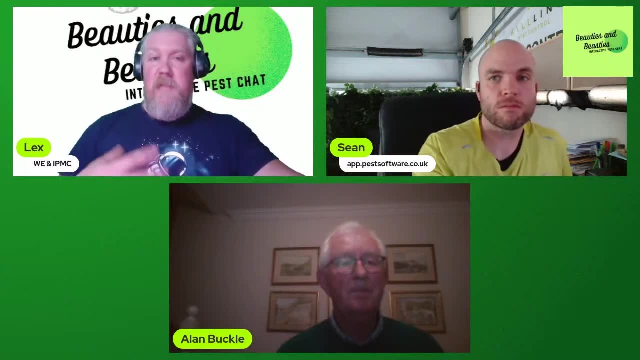 a number of animals who are going to be highly reactive at a much, much lower dose, and there's going to be a number of animals which will be, uh, unreactive at a much higher dose. the point being is, we can never refer to anything. we, for the love of god, we are using toxic substances. we can never. 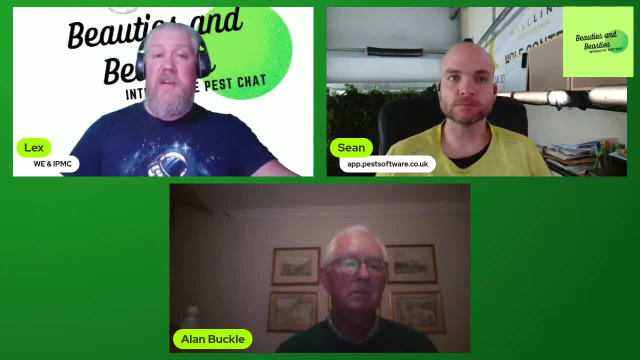 call anything safe. we never should use the word safe. we can simply just say the risks have been reduced and by that measure. the only way, therefore, then you can use your ld50s is as a measure of risk, comparative risk. certain products will have a higher comparative risk and others will have a. 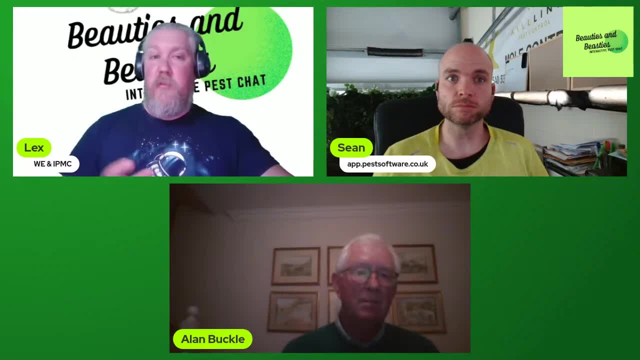 lower comparative risk. they're never to be assumed to be safe. there is always an inherent risk involved and all you can do through your kosh assessments and through your good practice is to pick the one which has the lowest risks and that you can use your ld50s to base that value. 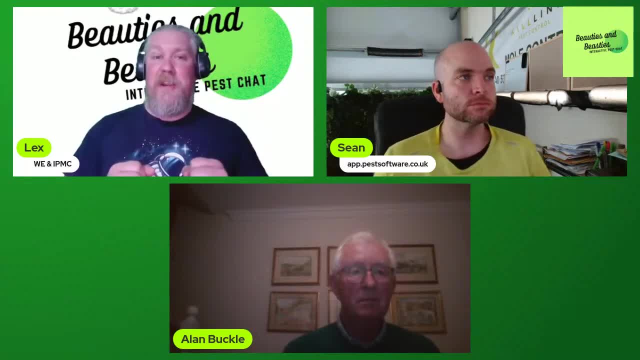 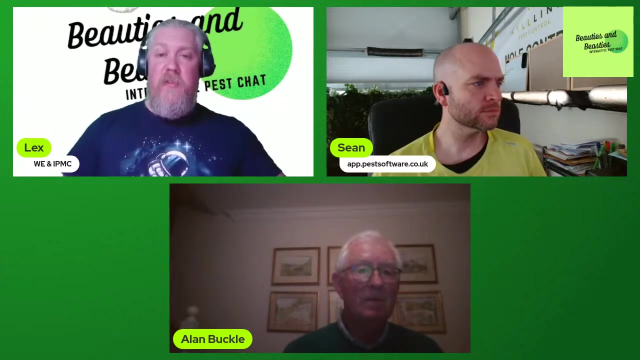 upon, not upon. it's okay to eat half a- you know, half a kilo, because your dog weighs three kilos and it's only x, y and z. no, it's a valuation of risk. yeah, there we go, so okay, um, i'll ask my last question: uh, alan, which is uh? and if you've got the time, who? who is the gentleman who is coming? 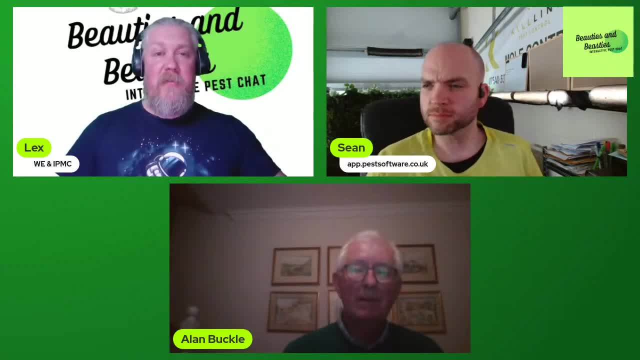 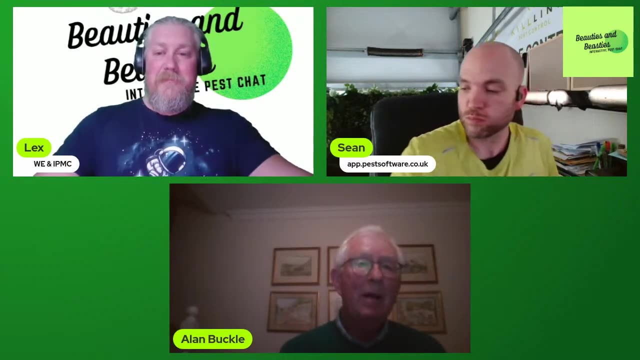 up to replace you. can you just give us, uh, a quick sound bite of who's nigel? who is, who is nigel, and and how did we get? how did we get to nigel, okay, um well, um, nigel, t is right. um, he worked for quite a long time in the renticle company and he was 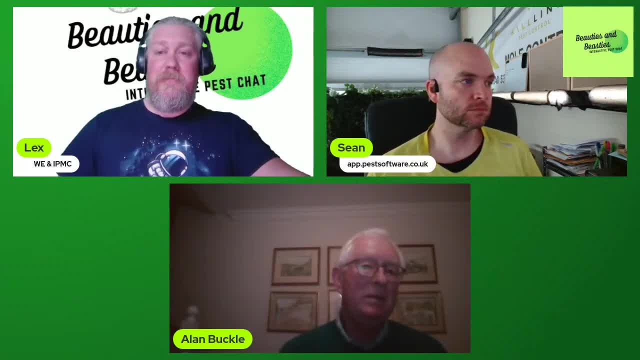 treat Kelvin j, mistress of um in crew. um he he. he was quite senior in the research and development side of royal and he came into crew and was the renticle representative and in fact the renticle director on the crew board for some years- um five or six years he was. 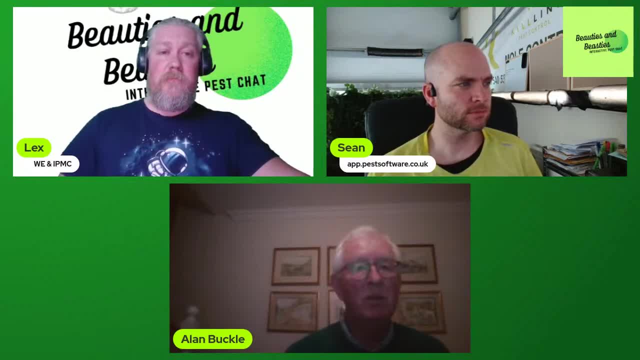 around in crew regime. you know, i told you we had these three or four years, actually frantic, mad years, rushing around meetings, um with all the user groups and so on, and he was around at that stage. so he was in at the start, um, he, he left rent to kill, um, but, um, when i said that i would no longer be doing this, 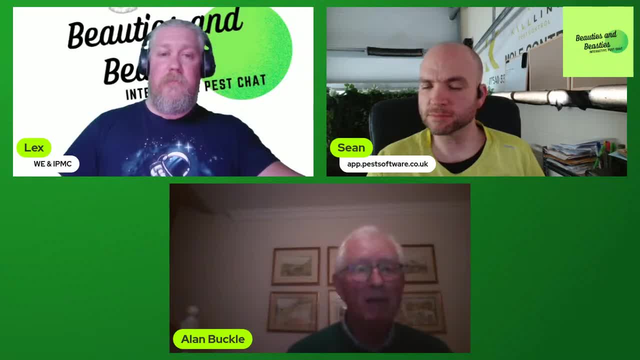 job, um, when i'm 75, which happens the middle of next month. um, the crew directors thankfully took me at my word and put the word out, um, and they, they advertised and and they got quite a good field. and the crew board and i had absolutely nothing to do with any of this whatsoever. i, i, i. 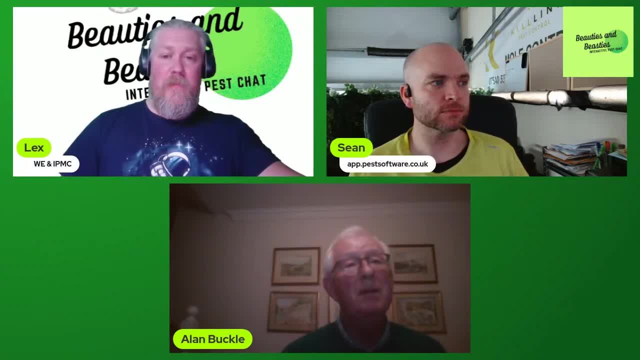 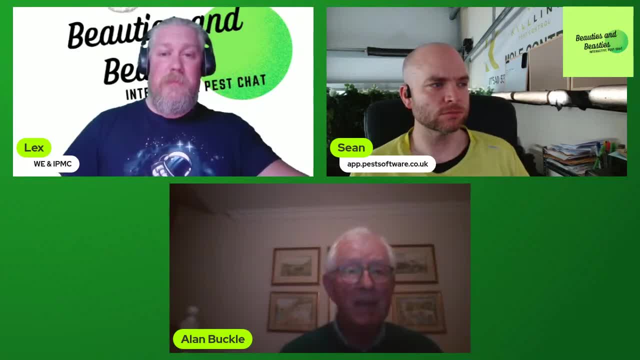 he's an excellent guy, um, technically, very, very sound um, and so i think i think he's he's a great guy and he'll do a great job. um, and i'm not just saying that i, but it's absolutely the case. i'm very confident, very to be handing over to him. i've been, we've had these two months as handover. 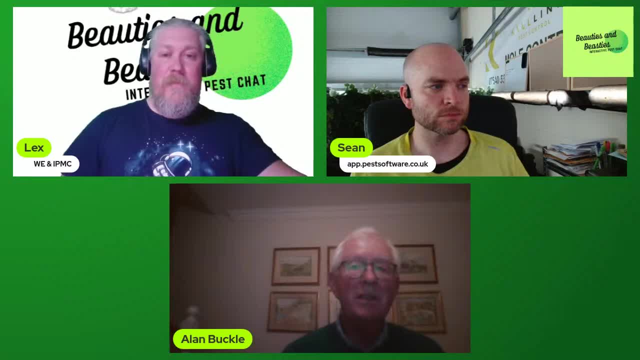 period and i've been talking to him on the phone almost every day, um, and so i've i've got to know a lot about him these last two months. he'll do a great job. good luck to him, okay. well, we look forward to getting him on the podcast and 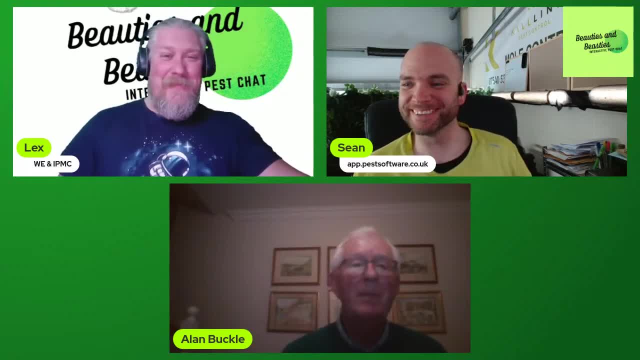 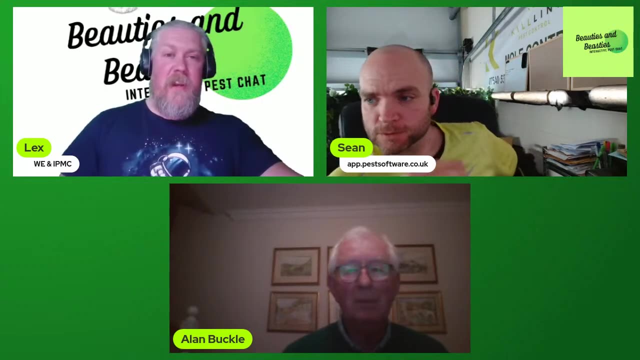 seeing what he has to say. yeah well, good luck with that. i, i hope, i hope you manage, i, i, um, i'll let him know that i've, i've been on and see, he see if he's up for it. oh, absolutely he's, he's got to do it now. you've, you've. 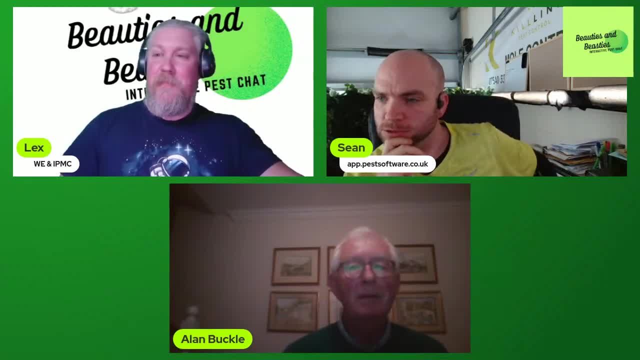 you know you've set precedent for this. um, he, he has to come on. but i think that brings us very much to the end of the show. thank you very much and i'll see you next time. you know to the close with this now. so, um, i'll put up the the closing three questions that we 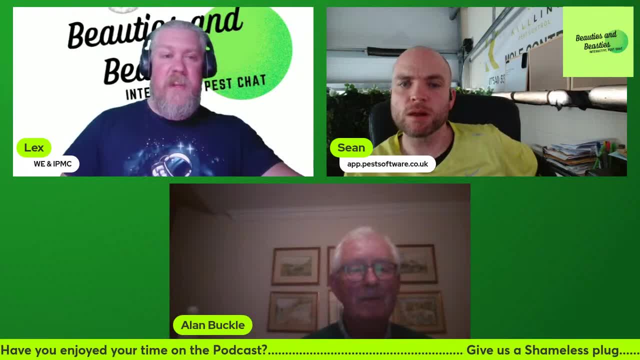 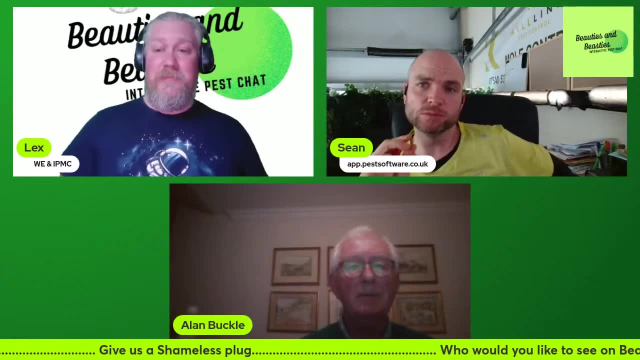 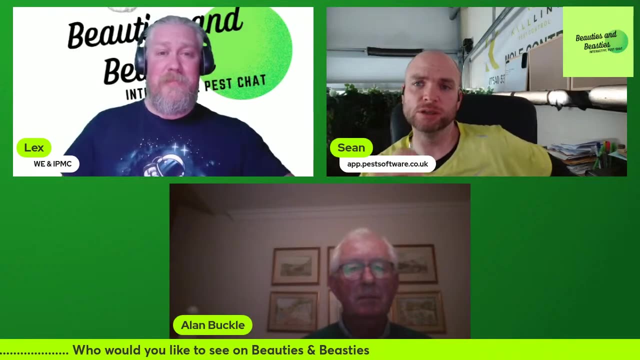 always, always, put up there and, sean, do you want to, do you want to lead? yeah, yeah, just before that, i just want to say a massive thank you, one for coming on, but two for what you've done with regards to getting us to the initials. so, getting bradifficum flamocafen all those years ago. 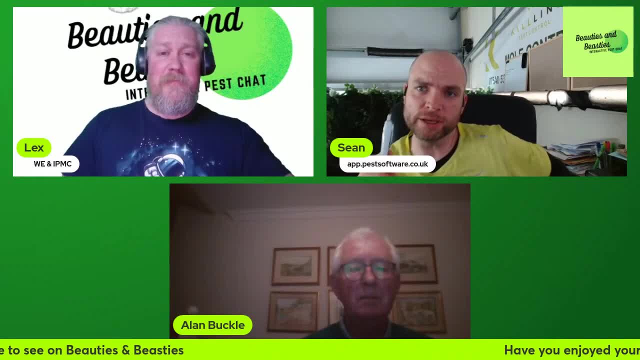 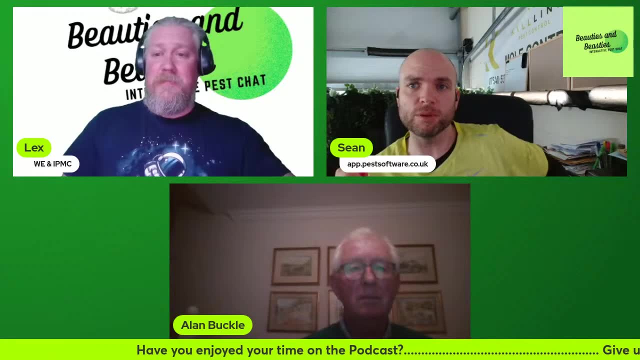 and the fact that we still have them in our toolbox. it can't be stated enough that we wouldn't have them now if it wasn't for for that work. so thank you from the bottom of my heart for everything that you've done and, um, you've been a fantastic guest. but to our three questions. 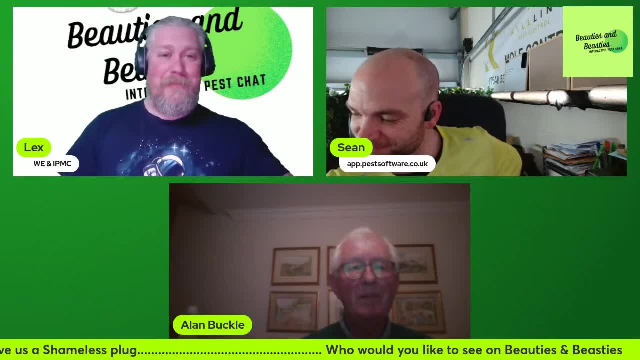 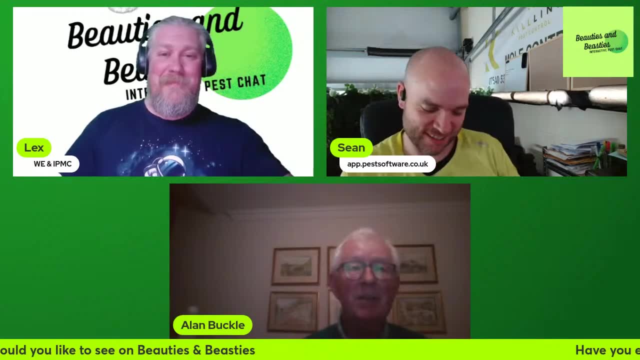 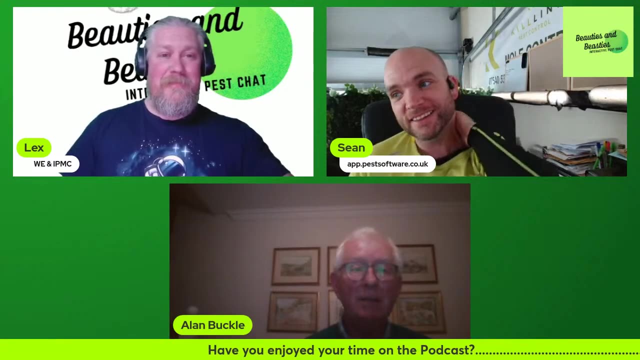 have you enjoyed the time on the podcast? is that, is that your your question to me? yeah, yes, yes, absolutely i- i don't know what's taken me so so, so long. it was a very lucky um time that that we met at at pest. yes, and so i'm, i'm. 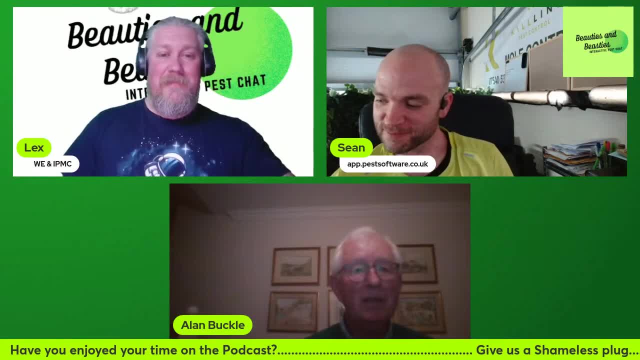 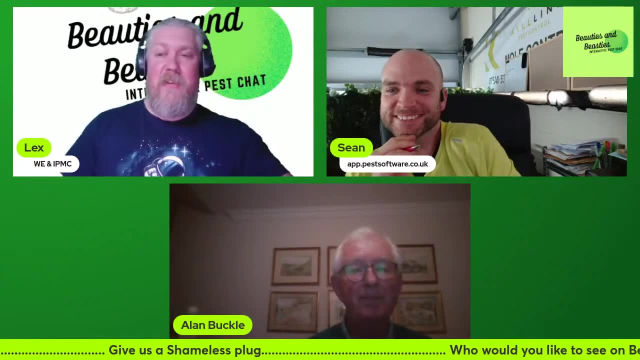 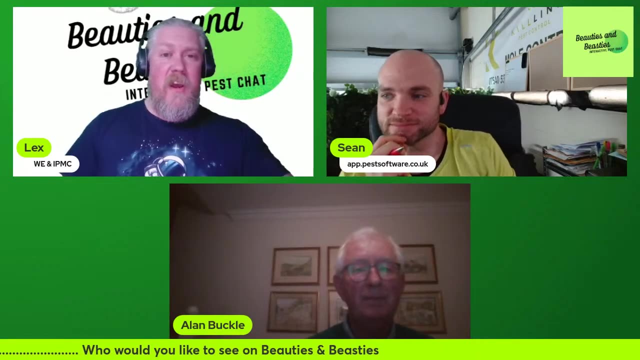 i'm pleased with it. um, probably, looking back on my time, should have done more and should have done it sooner, but i've enjoyed it, thank you. well, thank you for being on. i think that this is going to have people talking for a long while to come and i think it's going to put a lot of uh, a lot. 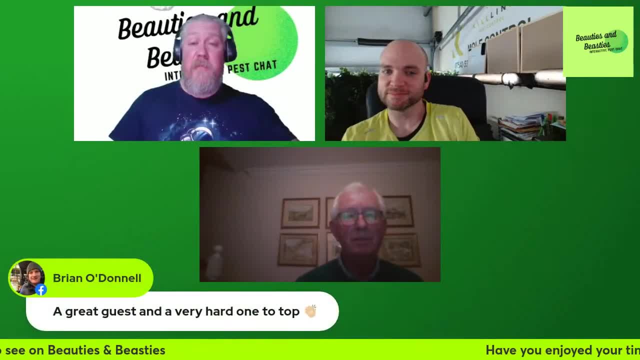 of people straight at the end of the day, it's going to have, um like sorry. and my question therefore- you know, i i picked the second one there is- which is usually give us a shameless plug because, because we usually have someone with a who's supporting a business. but uh, i'll rephrase: 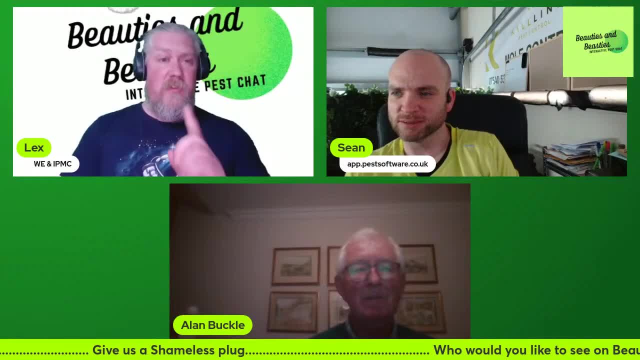 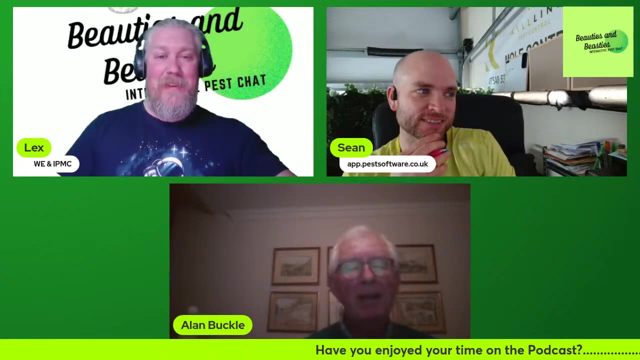 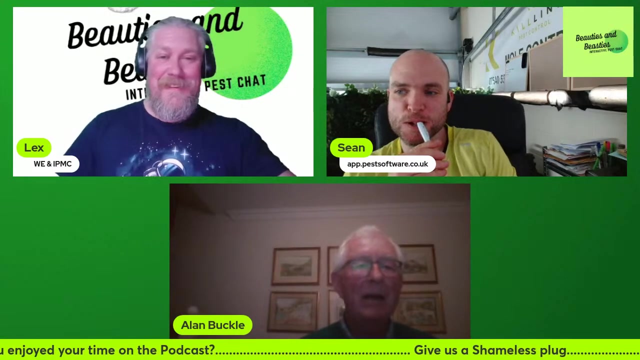 that to say, if you could ask the pest control community to do just one thing, go out and do just one thing. what would that one thing be? oh, my word, um, it's almost. i i just can't think of one of of of one thing, alex. um, i, i see. 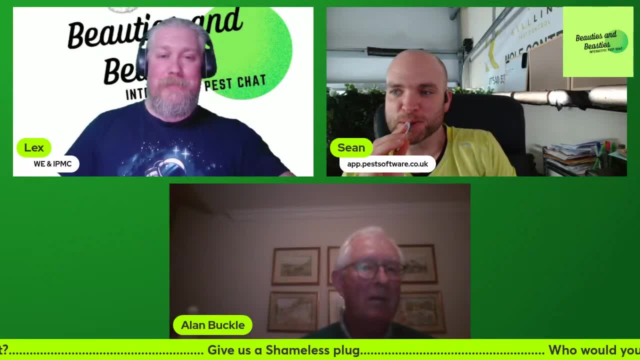 so much information about how good many of these people are and i, i would just say, um, if you're as good as our information tells us, you are, just carry on doing a good job and that's that's the best, that that's the most i can ask. yeah, i think that's a fair ask, to be fair, and you know. 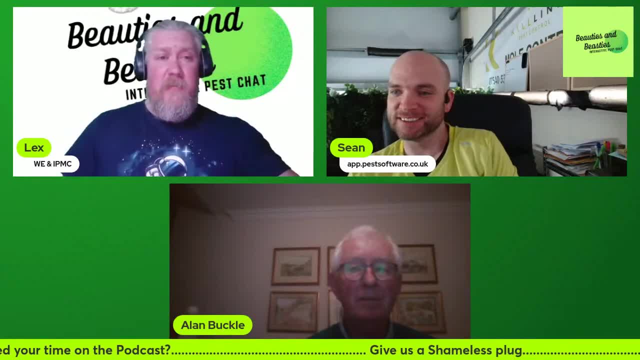 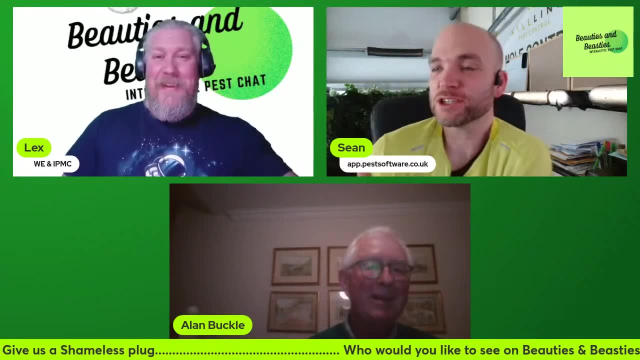 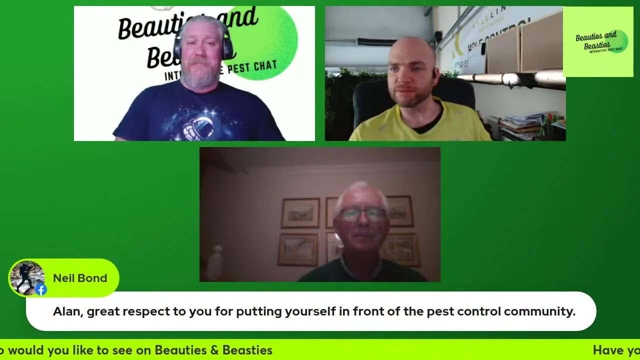 um, i think we can sum that up with: guys, be good, don't be shit, alan told you. so yeah, so there we go, um, and then last question, but quickly before i just want to read out some of these comments: um, alan, great respect for you for putting yourself in front of the pest control community. 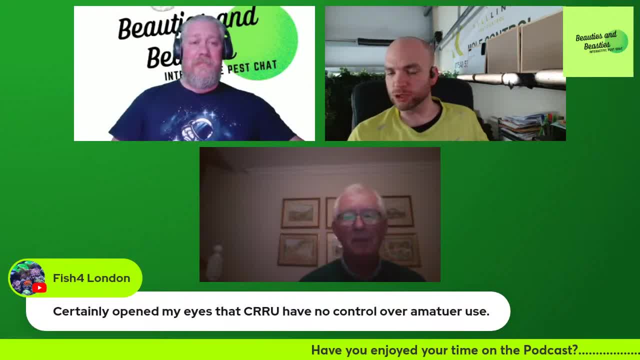 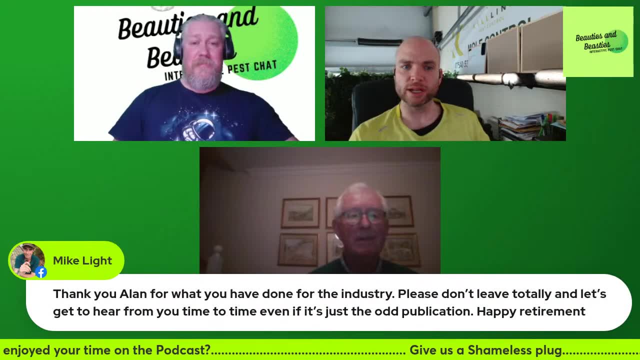 um, certainly opened my eyes that crew have no control over amateur use. um, thank you, alan, for what you've done for the industry. please don't leave totally, and let's get to hear from you time to time, even if it's just the odd publication. happy retirement, um. 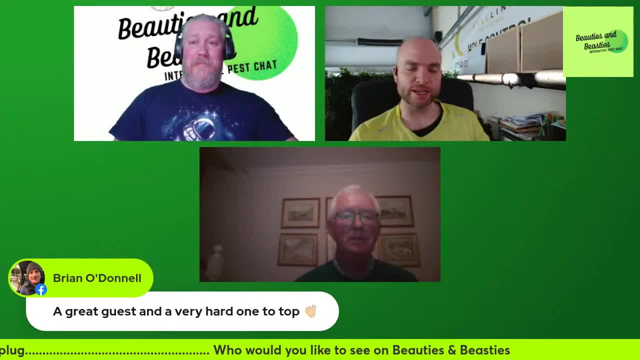 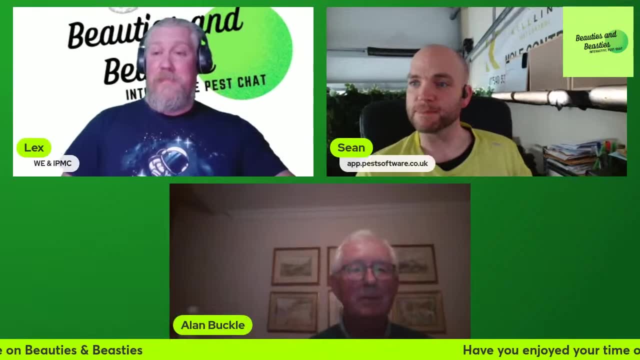 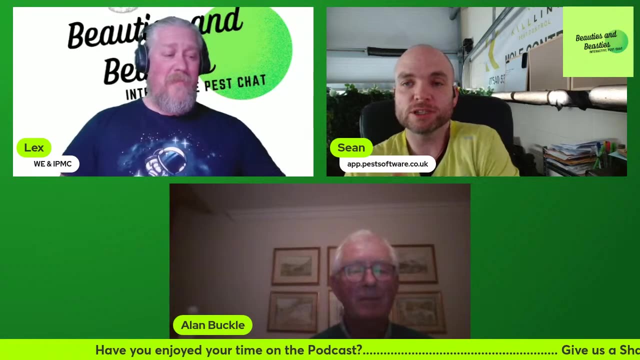 a great guest and a very hard one to top, and i can't lie to you. i'm sitting there thinking that that is a monumental um mountain for us to climb now, alex, to find something. um, yeah, but last question is um, who would you like to see on the podcast? who would you like to see come and talk to. 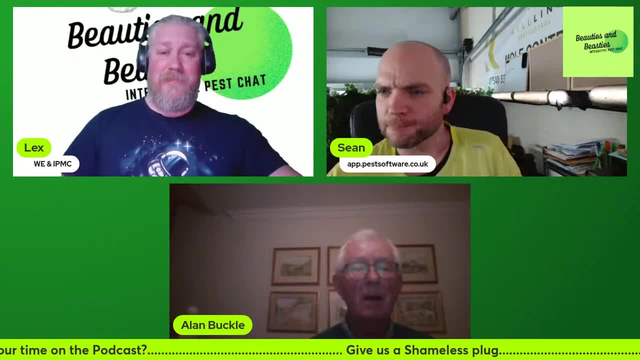 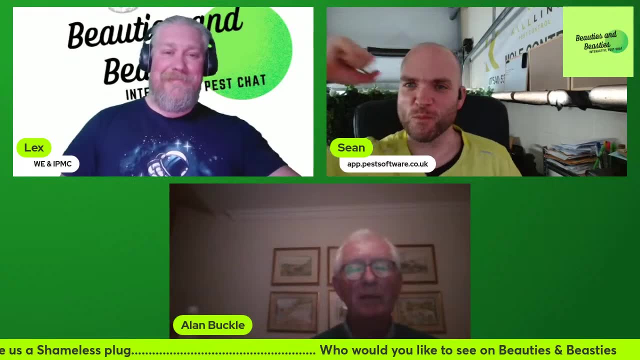 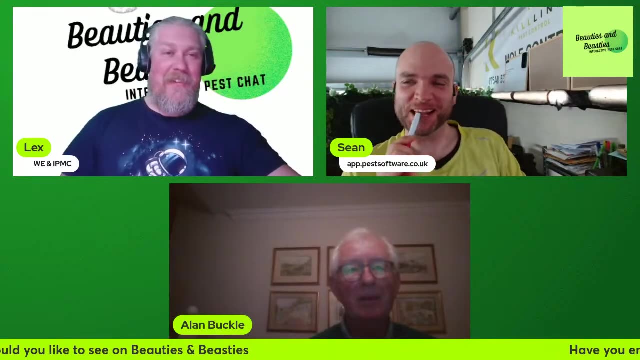 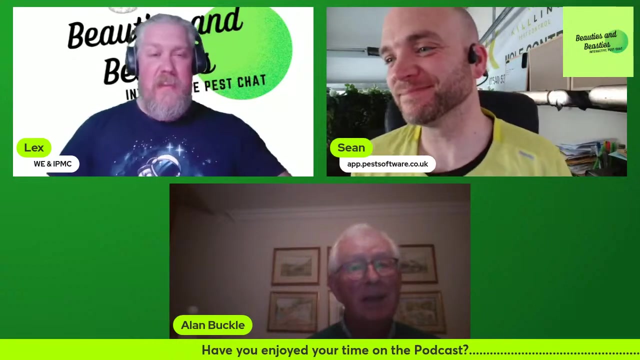 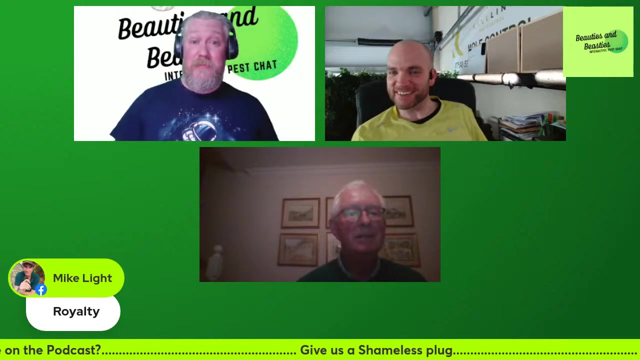 us. well, i, i think now we've spoken about nigel. i'm gonna have to warn him that, um, that he's he's gonna have to show up. yeah, yeah, oh, excellent, i'd like to hear. yeah, perfect. well, if you tap him on the shoulder- sorry, i might, i i just want to say i've seen loads of questions going down the right hand. 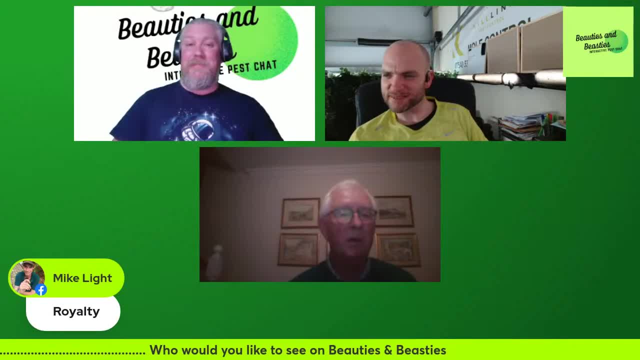 side of the screen. i would have loved to have answered, but if people want to just drop those in an email, stick it to info. i think wildlifeorg? um allow a couple of weeks to do that. so, um, please, please, do feel free to drop those questions into crew and i'll do my best to answer them, and i'm sorry we couldn't get. 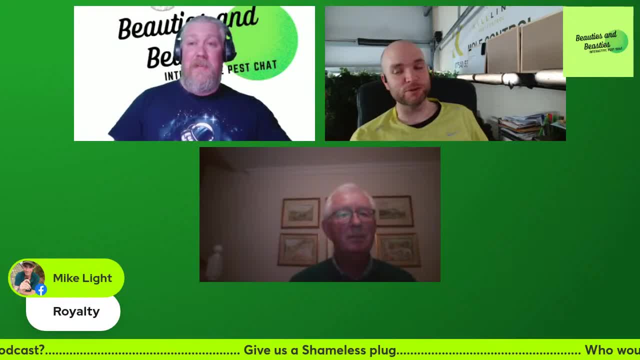 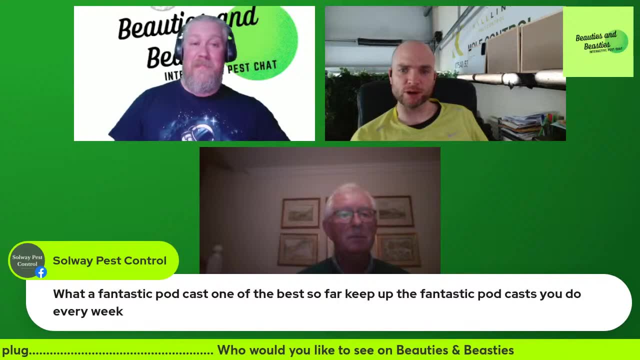 around a couple yeah hour and a half. it flies, doesn't it? so comment comment from mike, like royalty, and then from solway: what a fun, fantastic podcast, one of the best so far. um, you know, yeah, yeah, it's just. thank you very much for coming on. from the bottom of my heart, it's really. 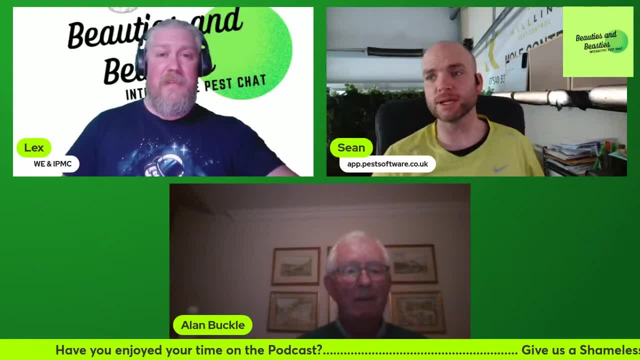 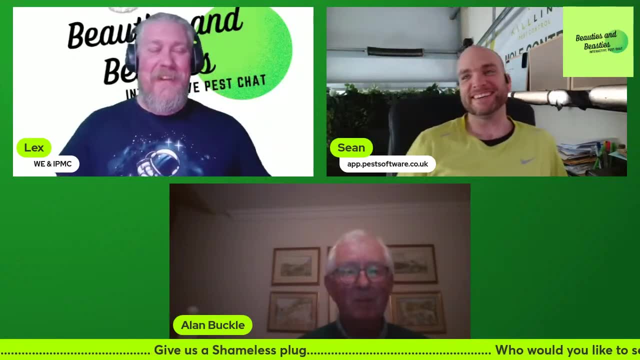 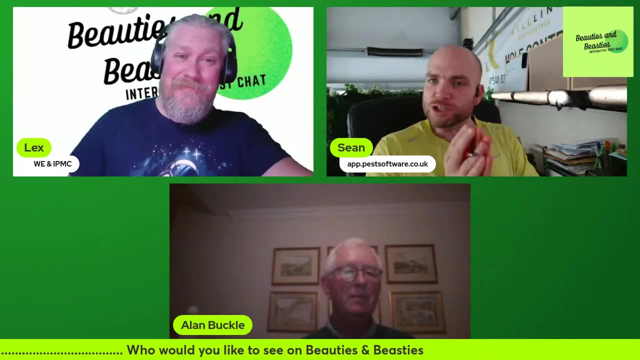 appreciated and i know it's appreciated from everybody watching as well, and me and me. great thank you. yeah, i speak for both of us. yeah, yeah, yeah, without sorry. sorry, are you going to dip your toes a little bit, alan, or once you're gone, you're gone. no, i'm once, i'm gone, i'm gone. i mean i, i, i'm. 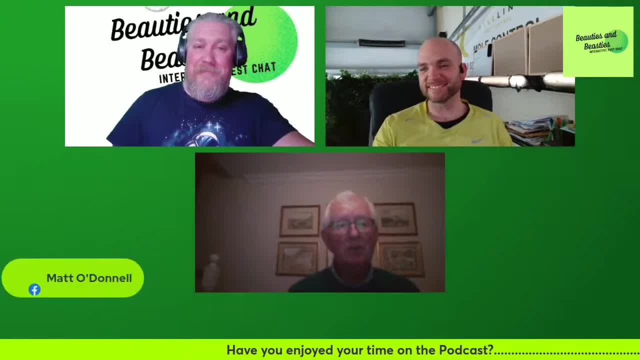 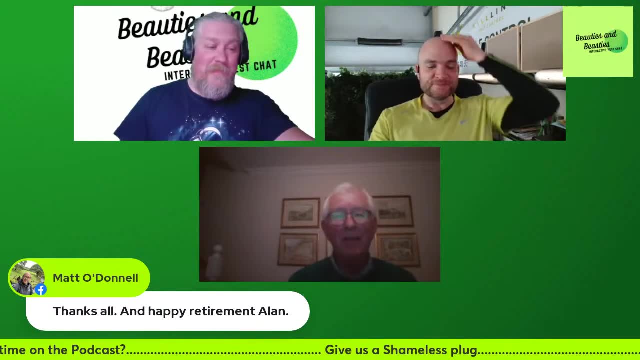 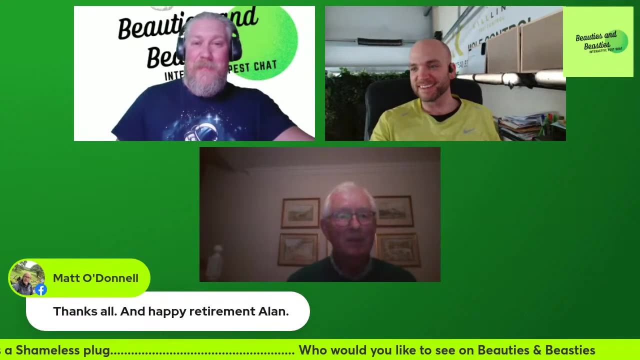 i let out how old i am. i am 75. i i should have retired 20 years ago, and, um, yeah, it didn't work out that that way, but i'm. i'm really not thinking of being a toes in anything other than a pint of beer, i'm afraid. yeah, so that's it, guys. this is, this is a auspicious moment. this is the first.